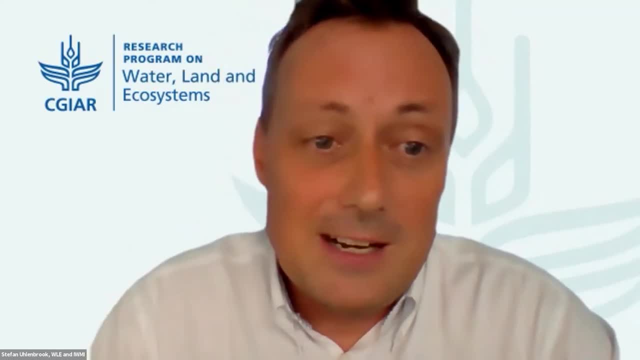 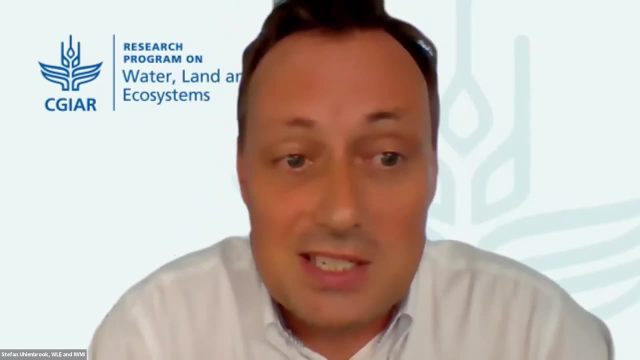 forward to the next hour where we will discuss cost-effective solutions that countries, communities can adapt, can adopt to enhance disaster prevention, preparedness and adaptation and mitigation to climate change. Colleagues at WLE, we have different flagship programs. 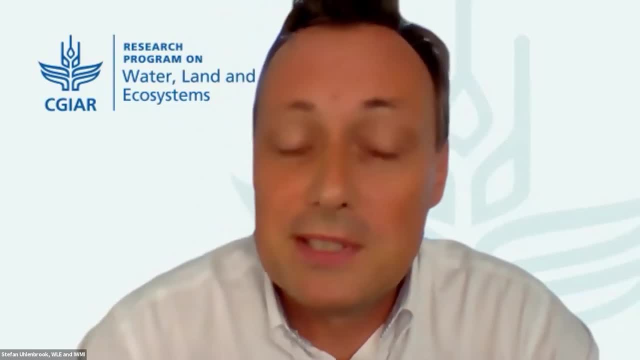 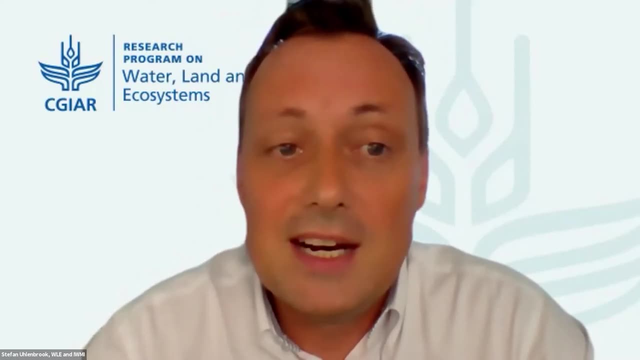 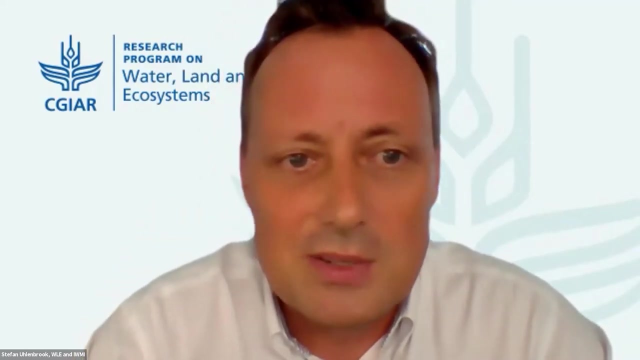 We have one flagship program that focuses particularly on the assessment of floods and droughts and also on improved solutions for mitigating and risk management in South Asia Particularly. there's not only focus on South Asia, but a lot of work has been done in South Asia. We will hear today more details about that Colleagues have achieved. 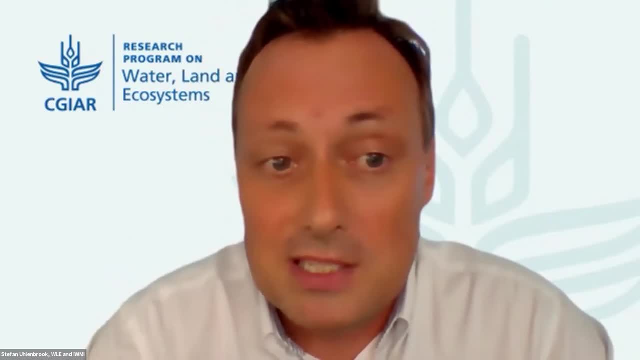 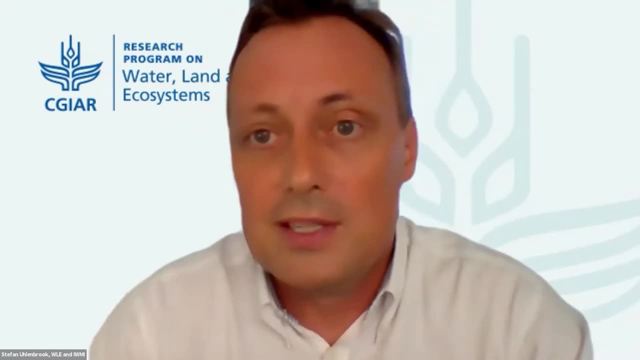 a lot over the last years. They established multi-stakeholder participation. they really very dynamically mitigated the impact of the pandemic on the environment and they have also been able to do a lot of work to mitigate drought risks through innovative ideas. They 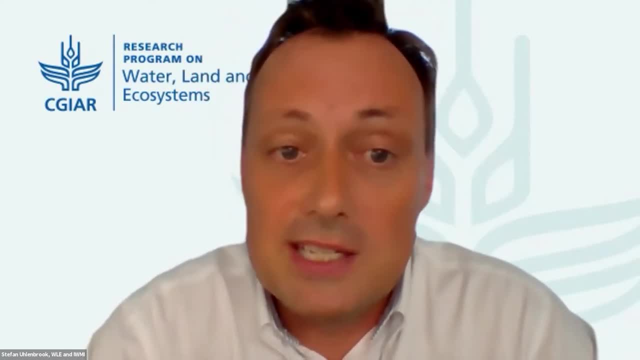 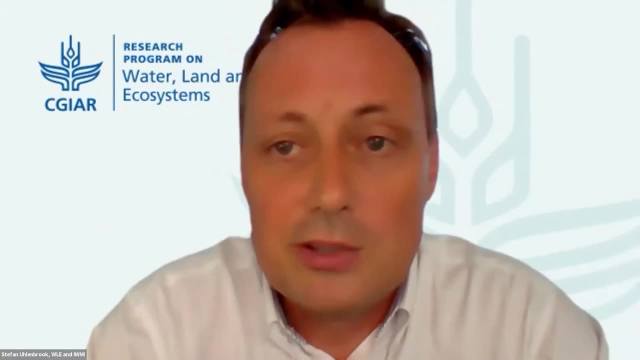 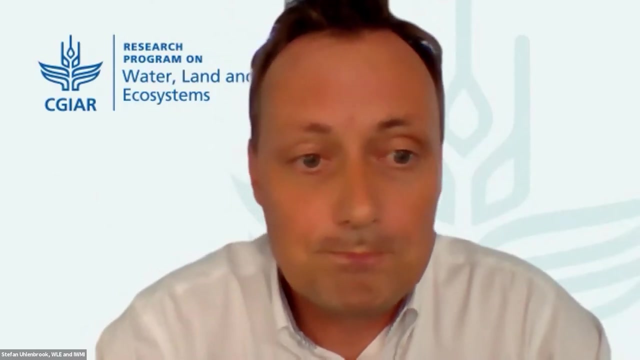 introduced high-tech technologies and brought that to index-based flood insurances. what really helped. These are low-cost insurances that are scaled up and scaled out to literally thousands of farmers, and that's due to the collaboration with insurance companies and many other stakeholders. That has been done with a number of partners and I'm very happy. 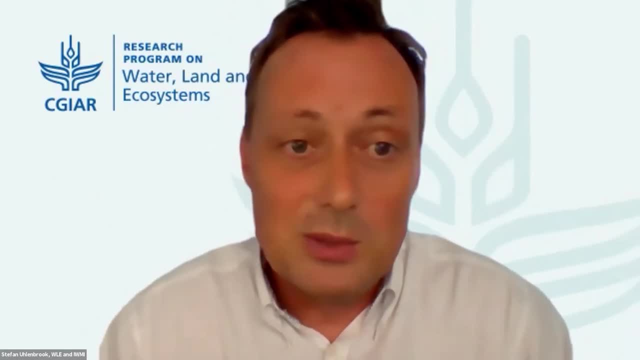 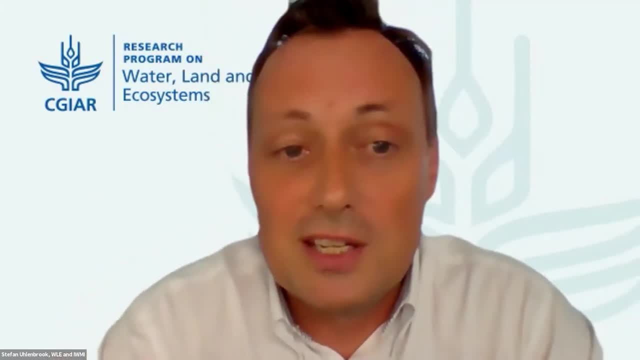 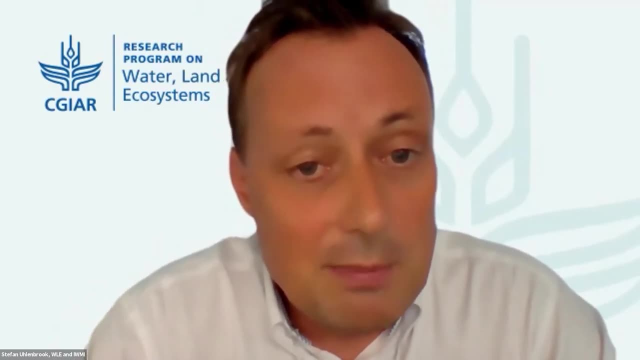 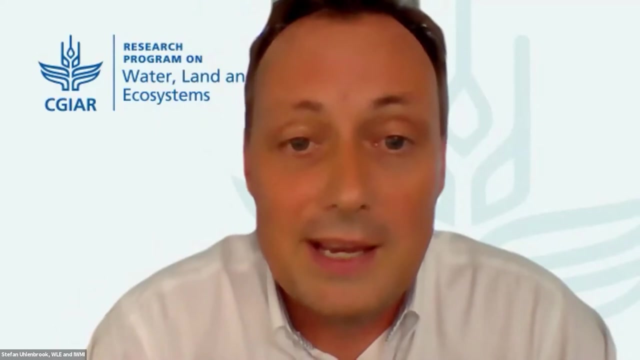 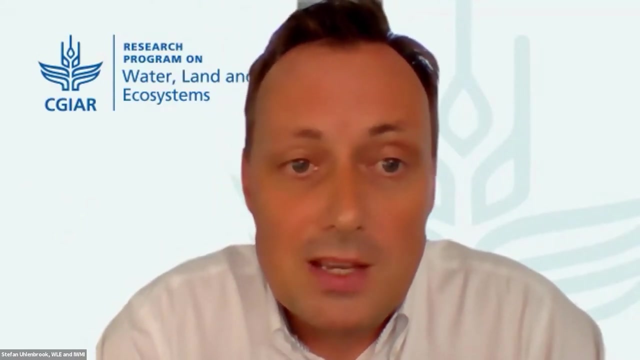 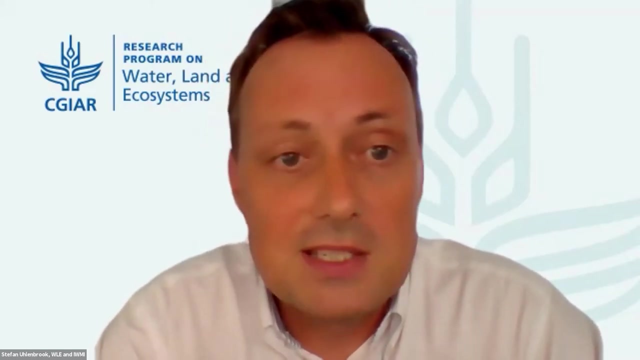 States of America, Sh EP of India and the President of the United States of America, iniz uh, introduce innovative disaster risk management solutions, uh, including the south asia drought monitoring system. we will hear about index based flood insurances and about bundled insurance solutions with bundling of seed systems, as well as climate information services. so quite innovative. 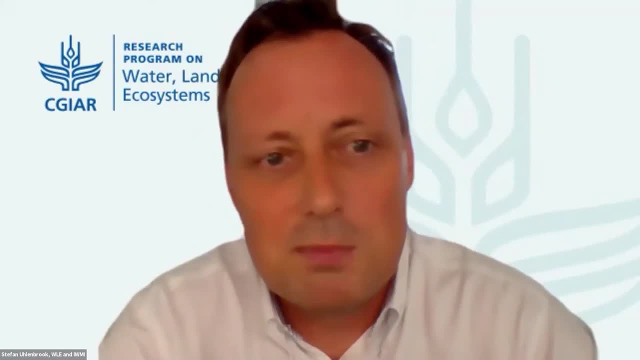 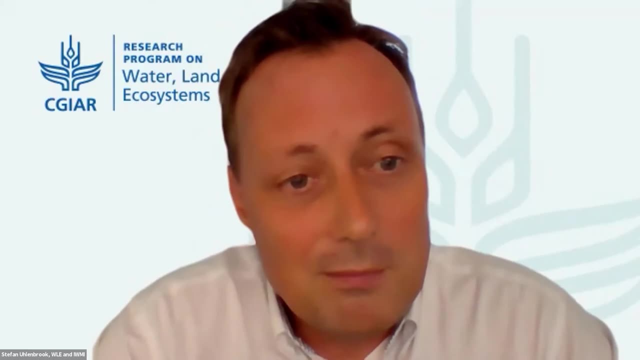 work. we will have two exciting keynotes. i will introduce the speakers in a minute. after that, we will have a panel discussion, which will be moderated by a colleague, and i'm very much looking forward to here, listen to the different perspectives from research, from development partners, from private sector colleagues, un uh, people working on the ground, uh, etc. and always. 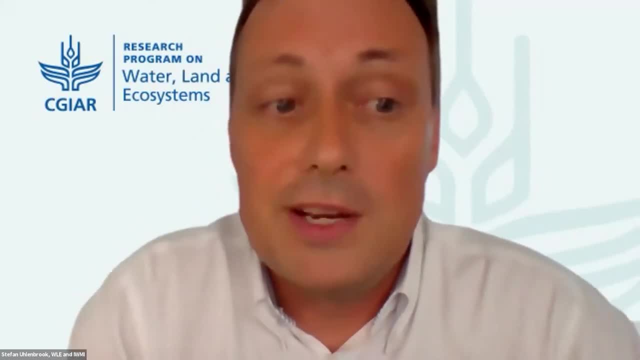 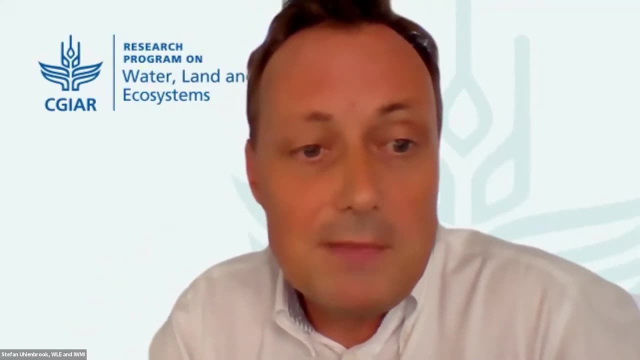 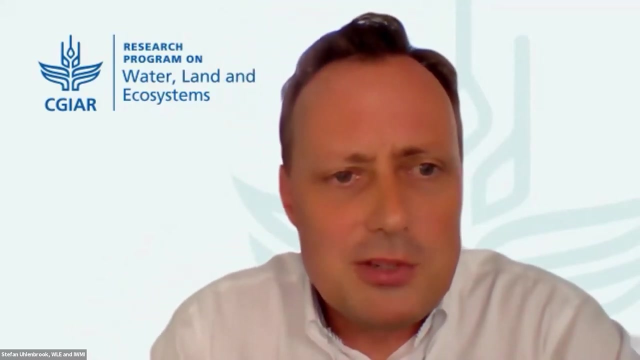 the objective to to scale up solutions to enhance the resilience of climate vulnerable farmers. so this is a great opportunity for south south learning and to raise the capacity and manage uh knowledge and share knowledge to reduce risks for professionals and uh multilateral organizations and companies. colleagues, let me let me introduce the first speaker of today and it's 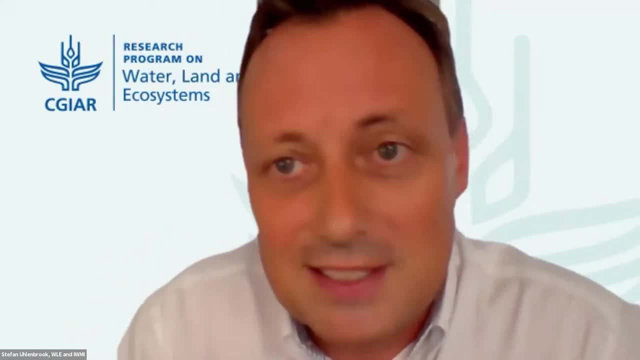 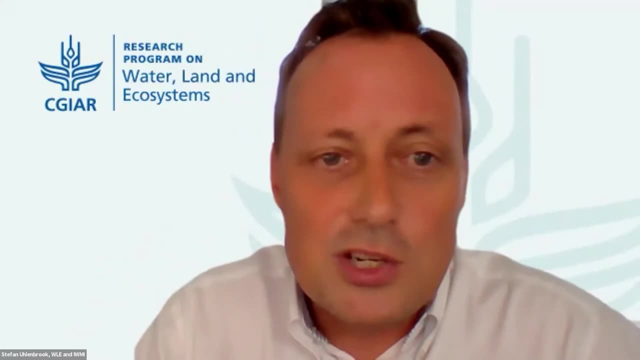 a distinct pleasure to introduce dr giriash amarat. uh, dr giriash was also the main focal person to develop the program of today. uh, he is a research group leader, as at the research group water risk to development and resilience. at any, he's a. 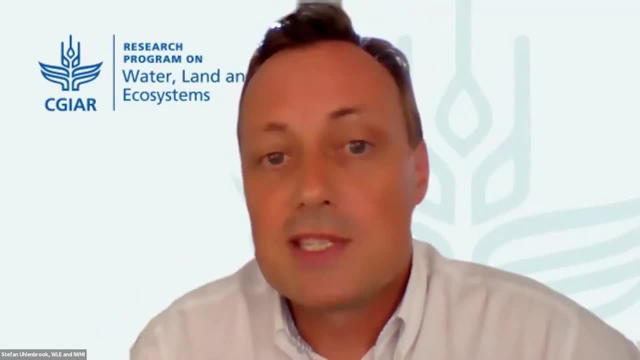 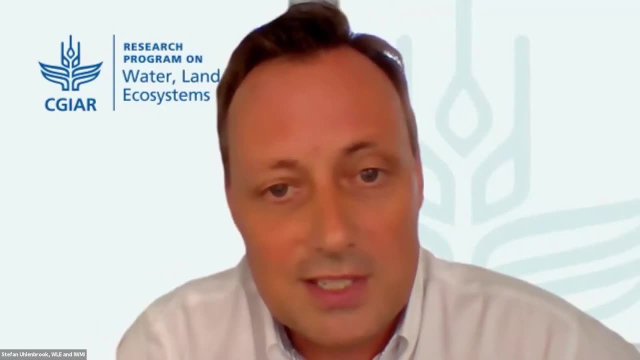 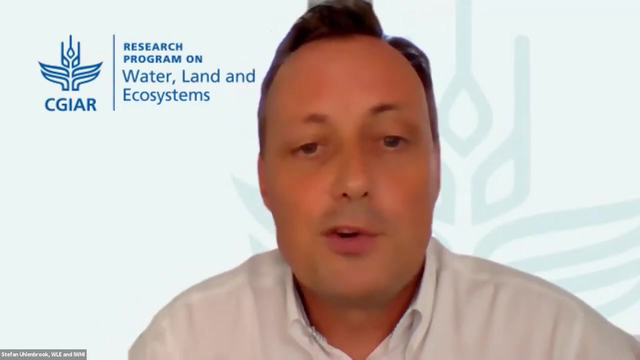 received his phd back in 2003 and applied remote sensing and landscape ecology later in germany and then later he worked as a postdoc at a french organization- also hold a faculty position at the university of bayreuth in germany. then he worked for easy mod in kathmandu in the period 2008 to 2011 and imi is very happy to have. 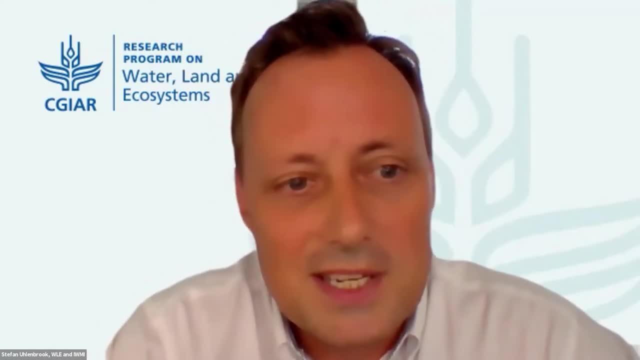 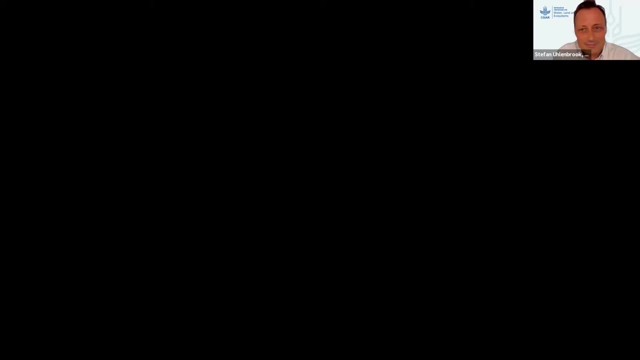 dr giriad as a as a now principal scientist- uh, since some 10 years- and a hand over to giriash to deliver the first keynote. over to you, giriash. thank you, stefan, for warmly introducing me to the participant. is my screen is visible. 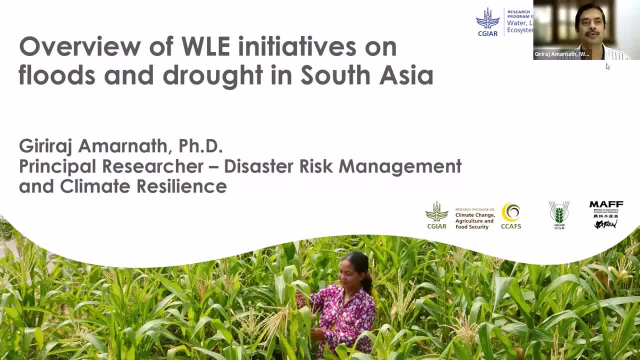 yes, thank you. thank you, stefan. so without further delay, given it's a very short uh intervention i would like to bring here. uh, i would just say thank u, dr giriash, for their like for uh check out what we are. uh, my giriash voice is dearly albany child, so, uh, thank you for everything and i appreciate it just. 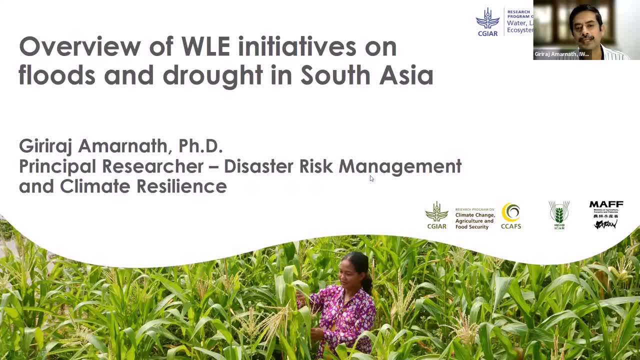 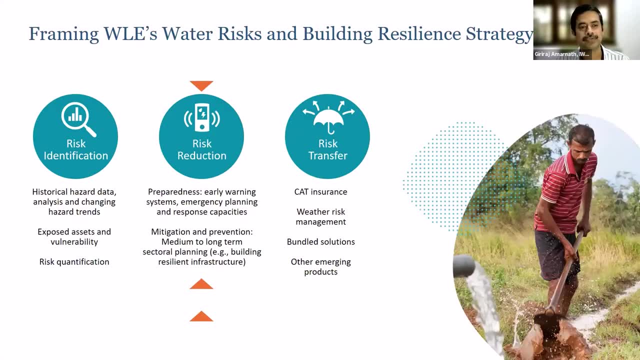 ICR and from the government of Japan. and now, before I step in more broadly, the fundamentals of why this water risk program is critically important. so this is how we frame our WLE water risk program. on the one side, we look at in countries identifying risk not going. 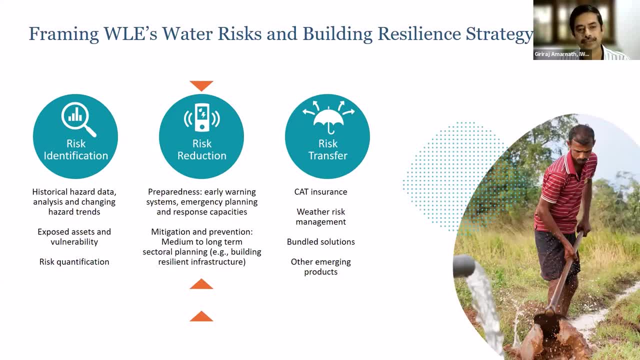 more technical details and then help us to know how we can reduce risk through early warning and contingency plan etc. where the ICR is going to speak more today on that. and then the risk transfer is about risk management, whether it is through bundle solution risk management. some of our partners from private sector will be speaking today, while we holistically 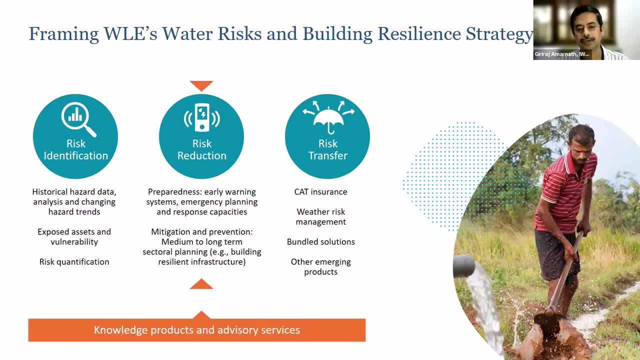 look this three pillars of our, we will be in a position to say what knowledge, products and advisory services will be able to provide across the range of partner. and then, while we're doing that, it is inclusively important to look at policies and institutional, without which we don't look at inclusivity issues. and 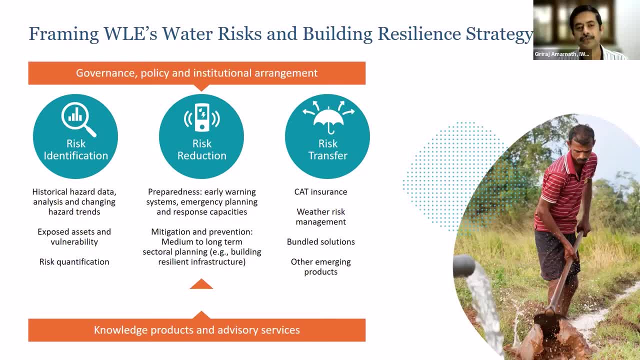 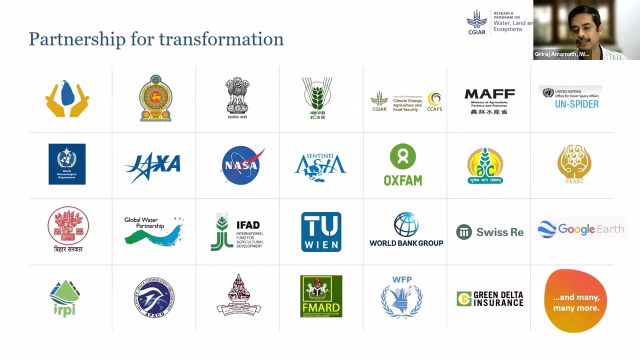 also, over years, we can look at how we strengthen the multi-stakeholder institutions in the process. and I think, equally, we have been proposing and implementing capacity building and the gender inclusive strategy led by some of our colleagues. so I think I must also thank here, before I go more into the technical. we believe in partnership that led to this transformation. 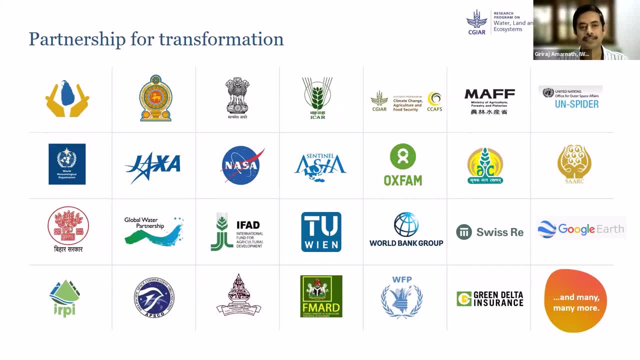 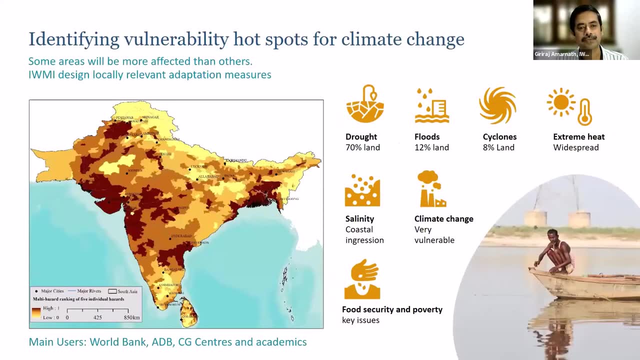 of this important pillar of CGR program on WLE. Thank you for that question. Thank you, speaker. my name is Dr Amin Patel and I am the social and economic services coordinator for the WLE program. Me and Dr I have been working with please for the past three years, which is a project called. 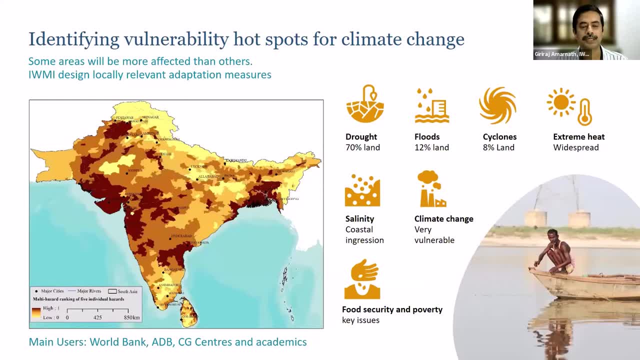 continued efficiency of the WLE to identify climate risk at the risk level for urban areas and also for the risk level for urban planning. so we look at different climate hazards in the area, whether it is flood or drought. we super impose and come with the hotspots where 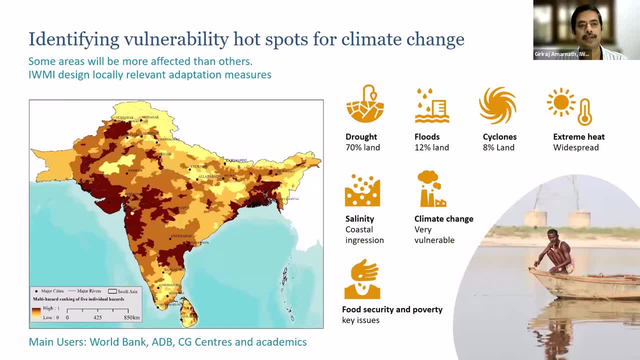 regularly the areas are going to be a climate hotspot. and then what locally relevant adaptation measures we can develop, and one of that is identifying flood prone regions for risk transfer mechanism, for which we have developed a SWMR to be able to optimize that. Thank you, 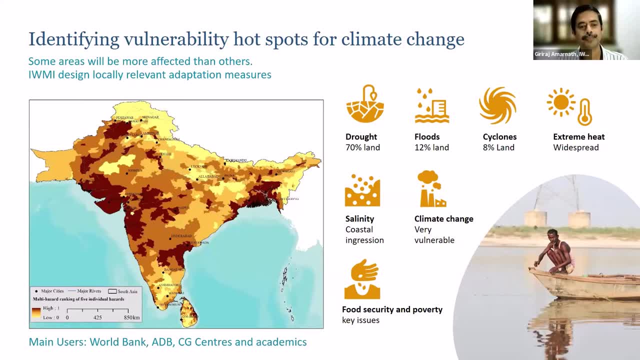 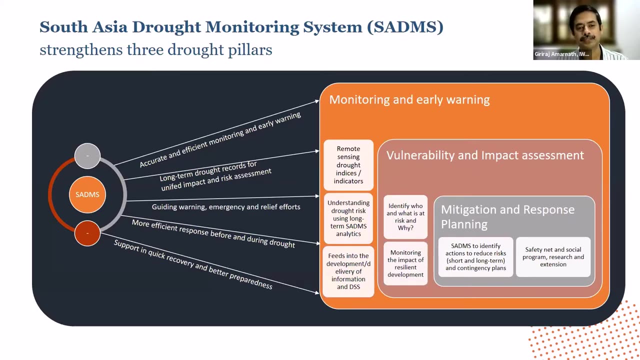 suite of tools and technologies which we will speak today. in the other set of intervention, we are focused on the drought preparedness strategy, which we will be also briefly going through that. so i think, uh, while we are started the wle, there was also a major milestone from wmo in terms of 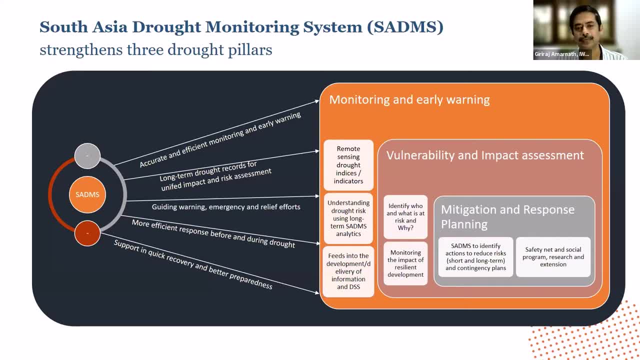 integrated drought management program, which is a very popular strategic framework developed by wmo and gwp. and if you look at this three pillar, talking about monitoring and early warning, vulnerability and impact assessment, and the third set of pillar is mitigation and response planning, wle was good enough to implement across these three pillars, using technologies, using ground, 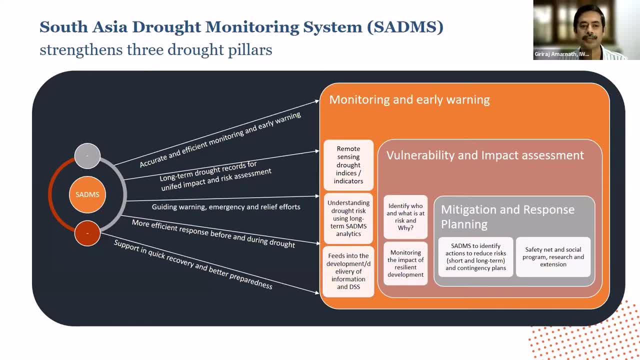 based information and to ensure the south asia drought monitoring system is not just about data collection, but also looking at response strategies and also how this data can be useful for risk insurance related uh elements. now, as i said, with limited time, we are not going to go more detail on south asia. 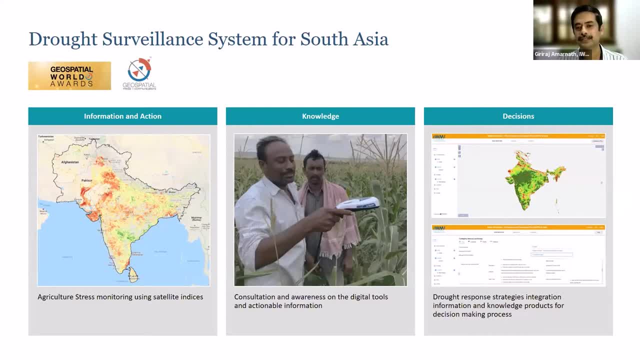 drought monitoring. the purpose is: we produce this data where we work with national members. it could be icr, it could be disaster management or with the world food program. our colleague from world food program sri lanka will be speaking during the panel session, so taking the ground. 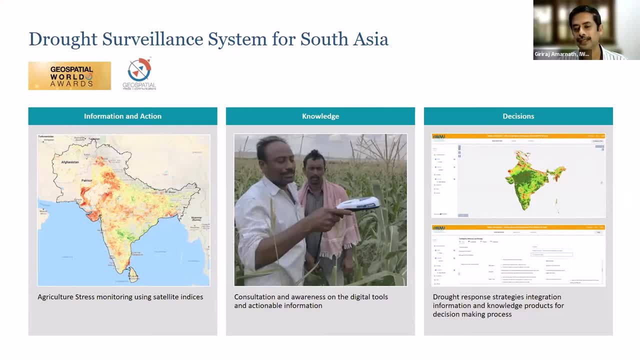 based information, satellite data, you could come up with a near real time contingency plans to help how countries can respond to the crisis. so during this process, we were able to recognize this particular initiative from the geospatial consortium of winning the 2020 geospatial award for this. 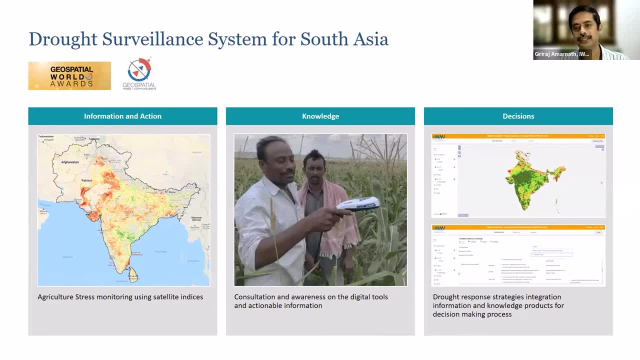 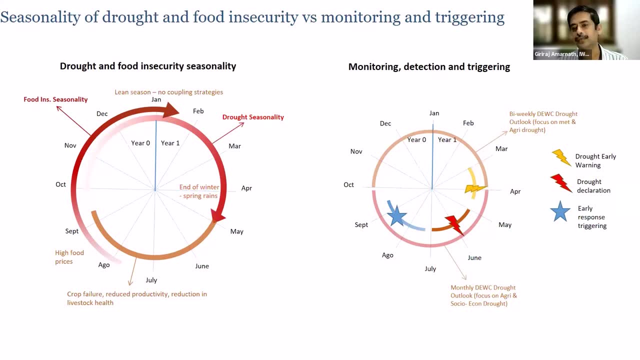 particular system capabilities, and i think it's not just about monitoring and information. what we are looking at is to monitor, detect and trigger, timely the response strategy- a good example we have been doing in uh, following this good work in afghanistan, where this particular system is rolled. 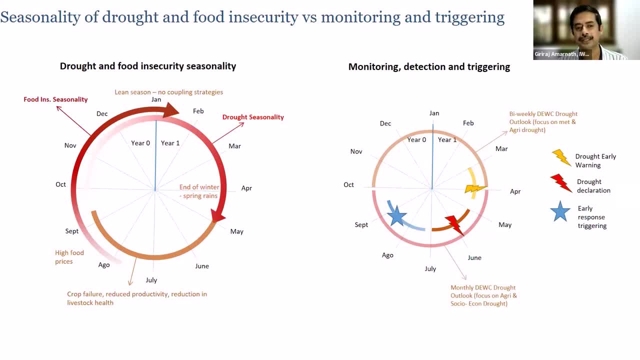 out and it's been used and, in fact, for the first time in afghanistan, the declaration has happened quite early compared to the 2018 drought, where there was a lot of challenges of having timely intervention by the policy makers to declare drought and also provide relief. 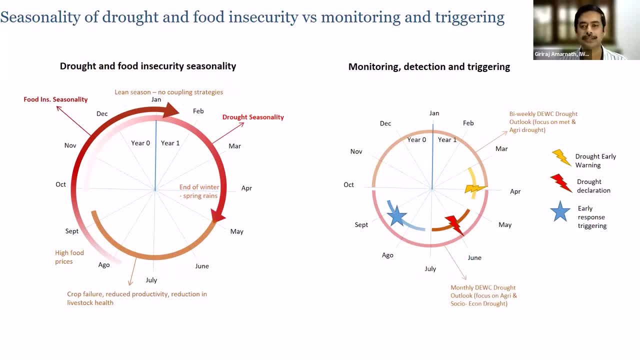 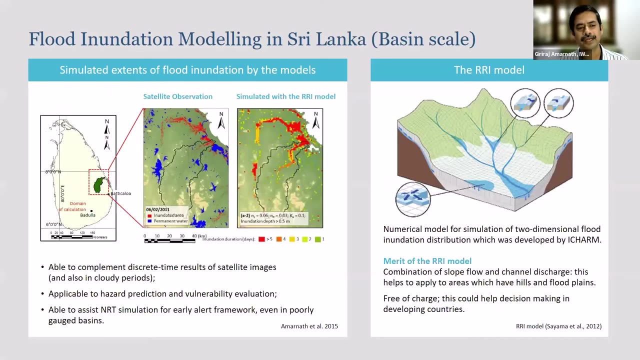 so understanding the seasonal behavior and also the challenges of drought severity, you could come with these kind of a modern form of information to provide drought mitigation efforts. and just moving from flood to drought, we have proven flood inundation models. we believe in open access, the principles of what cgr we follow. 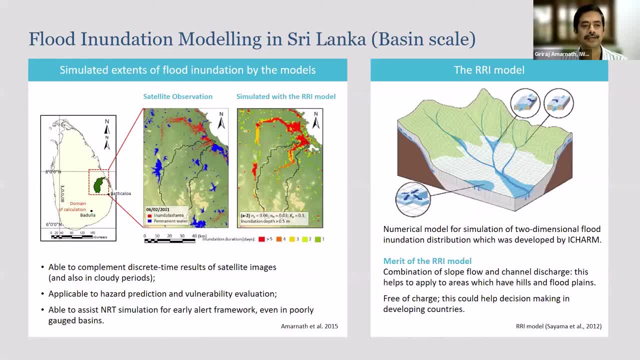 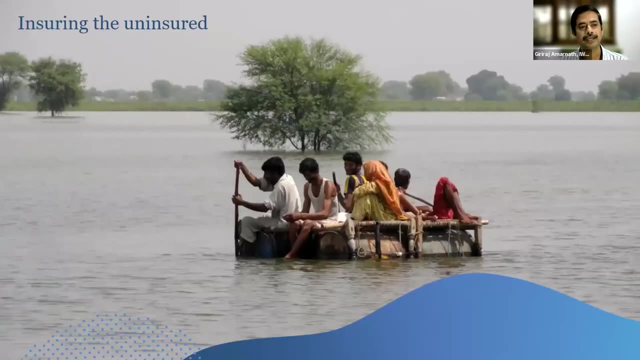 we have a suit of tools that are developed for small scale river basin to large scale river basin models. that led us to developing a flood parameters and using that flood parameters. we were focusing on how we can ensure the uninsured right. so that's the main focus of that and we 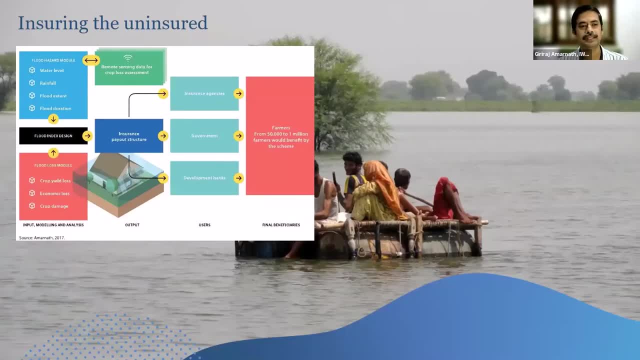 developed with uh insurance companies, including swiss free and others, to design and flood index And today this has been scaled out: over 100,000 farmers in different part of the regions in India and Bangladesh, where I believe other in the panel will be speaking more on that. 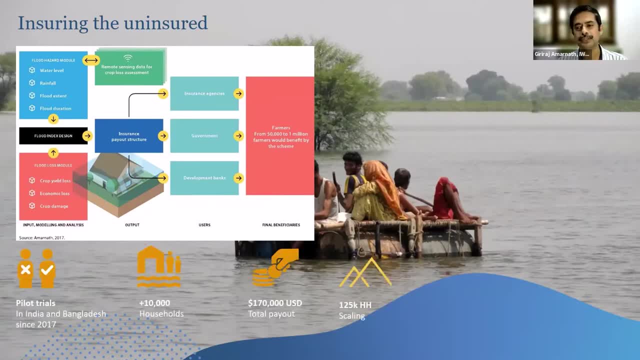 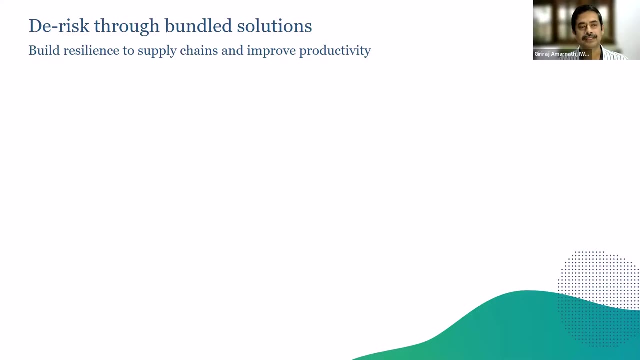 So these are some numbers And again, these proven solutions are again being recognized by Group of Earth Observation in 2020 for winning the Climate Action Award from the Group of Earth Observation. And I just want to also take it further like, yes, risk transfer is equally important, but we also need to look at how we look at the larger de-risking strategy in providing better supply chain and improve productivity caps. 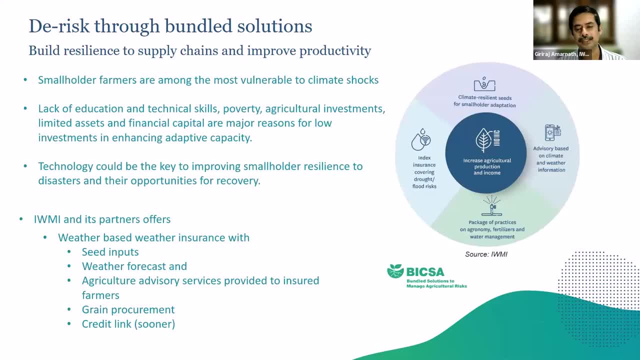 So what I mean? I would skip this point, but what we have done is we work with various partners. it could be a private sector, it could be a government agency. So what is trying to see here, this particular model is we look at. 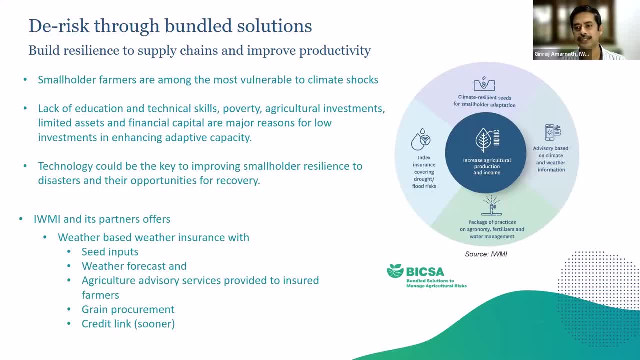 We look at the entire value chain, from seed distribution to advisory services, to weather insurance And also this is the this season. we have also spoken about the grain procurement as well. We are now going to also launch the credit link related product as well. right. 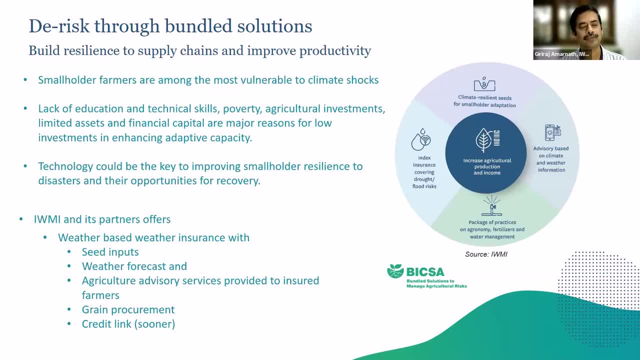 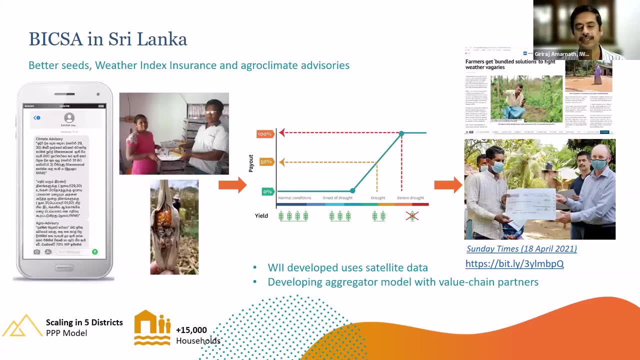 So this is just a sample for Sri Lanka, where we have rolled out weather advisories, are provided best management informations are tailored to the communities And we are growing with those evidences where open access data- such innovative technology We're- We can blend in seed companies with insurance. 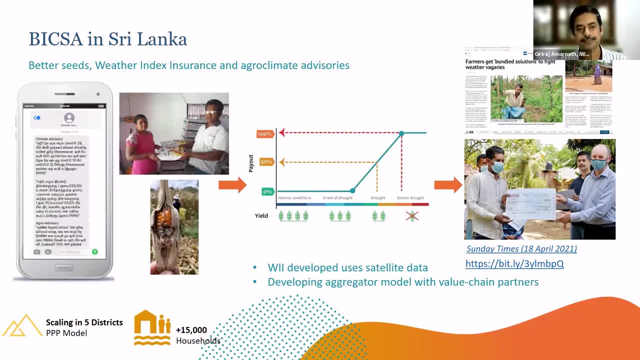 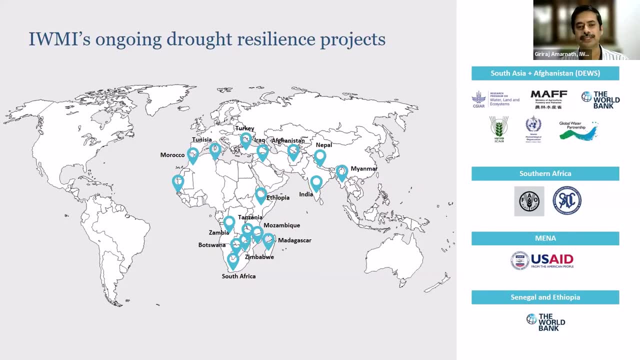 We can say the larger resilience strategy can be addressed here and not just about the pilot. We are now talking about scaling. We have been expanding to moving from South Asia- though this event is for South Asia- We are now growing into Africa, to Middle East, et cetera, with the great commitment coming from the strategic partners. 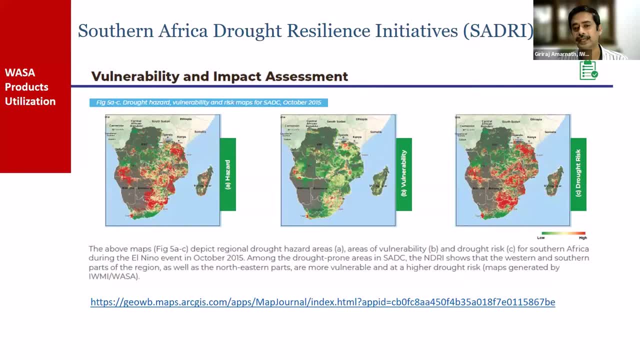 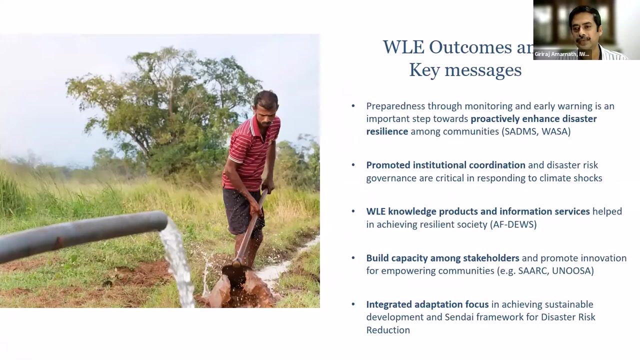 And, as I said, this is one piece of information where the entire Southern Africa has adapted our framework and we will share this link where Southern Africa drought resilience initiative is also launched by World Bank. They are using pretty much the framework. What I WMI through the WM initiatives and my take home outcomes from all these pieces of work is one is: it is very clear that for preparedness, you need near real time monitoring and early warning information. 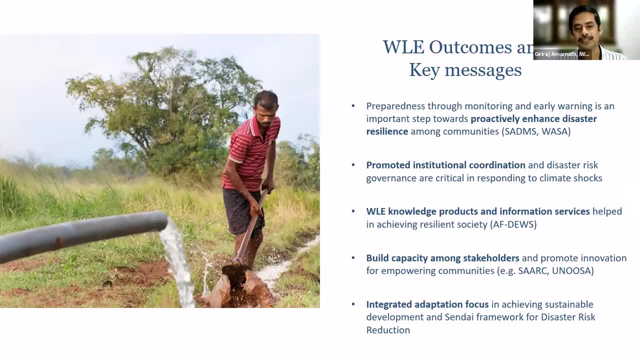 You need to have better institutional coordination. It's not about silo driven Outputs will never make any delivery, So we need to look at Institutional coordination and I think we can speak of the volume of WL knowledge products that has been developed and disseminated to various countries in the region. 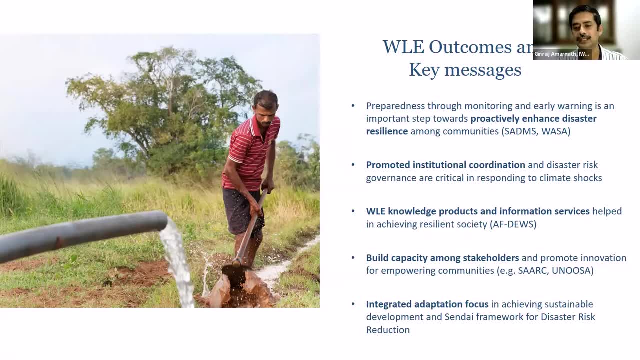 And we also work with you and also, and with Sark and other partners, to build the next generation of capacity building And that's that's always a sustainable way to look at the next generation of capacity building. And I think the larger focus we always see is the adaptation. 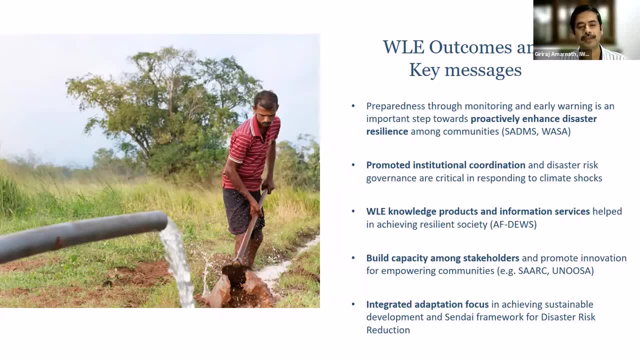 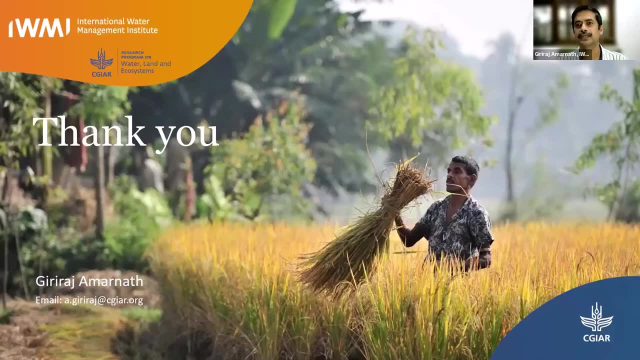 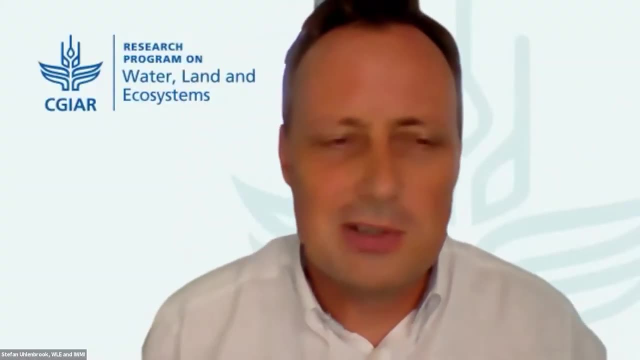 Focus is not just about doing something, But also keeping our goals of SDG and as well as the Sendai framework. with that, I stopped here. Thank you over to you, Stefan. Thank you, Gary Ash. It's truly impressive to see you know the work of the last 10 years that you and your colleagues have achieved and how this is scaling up, but also out to to other continents, literally the whole world. before we enter the discussion, 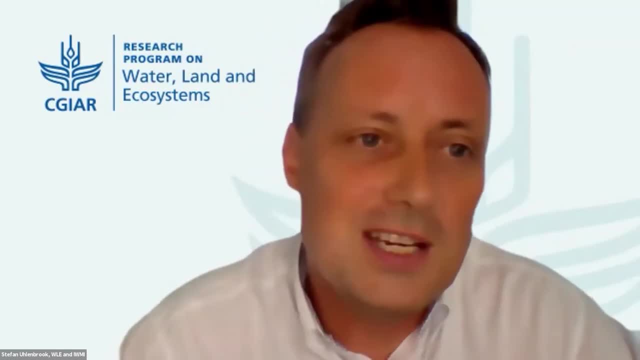 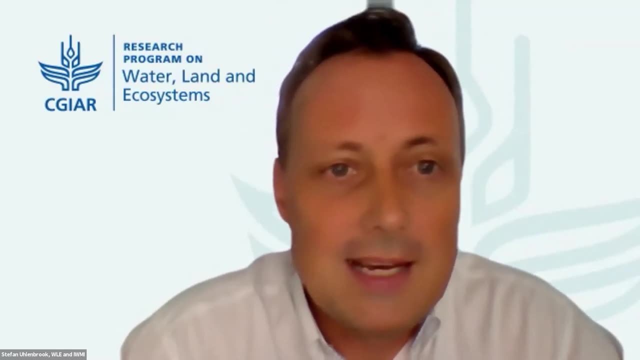 I it's a pleasure to invite the second keynote speaker of today, and Dr Abdul Islam is the Assistant Director General for Soil and Water Management at the Indian Council for Agricultural Research in New Delhi. Dr Islam holds a master and a PhD degree from the Indian Institute of Technology in Karagpur. 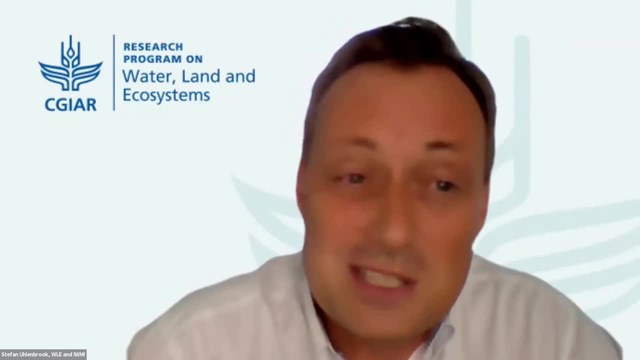 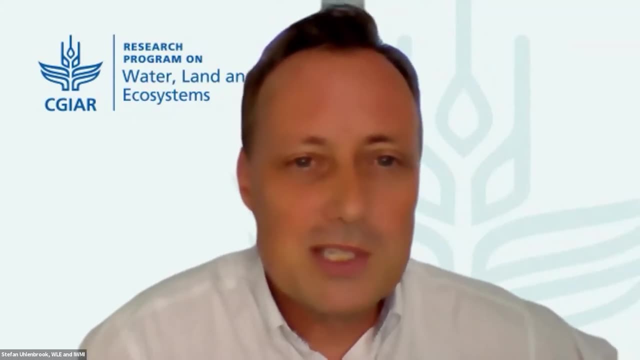 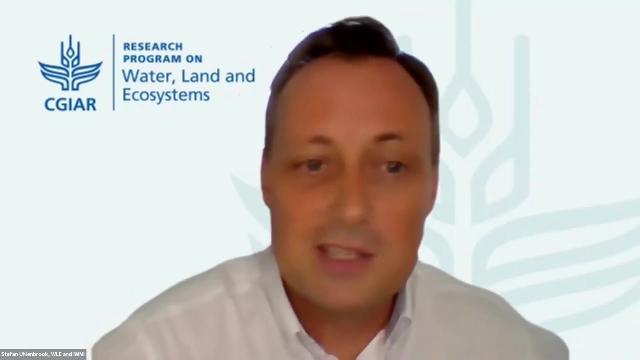 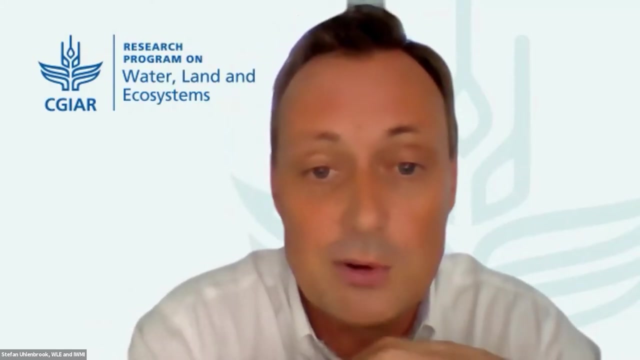 I hope I have correct correctly said that he's quite an established and accomplished scientist as well, So I'm looking forward to his presentation. among other things, he has been awarded the Global Research Alliance Award, the Norman Bullock International Agricultural Science and Technology Fellowship by USDA and others. that Islam has 25 years of experience of research, research for development on issues related to soil, water management, agricultural water resources planning, management, modeling, hydrological modeling, but also hydraulic modeling, and for irrigation canal operations, etc. 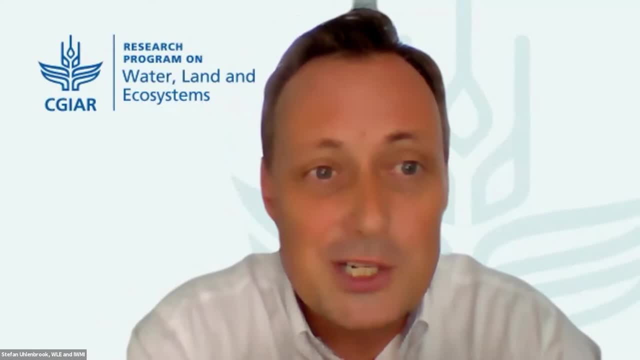 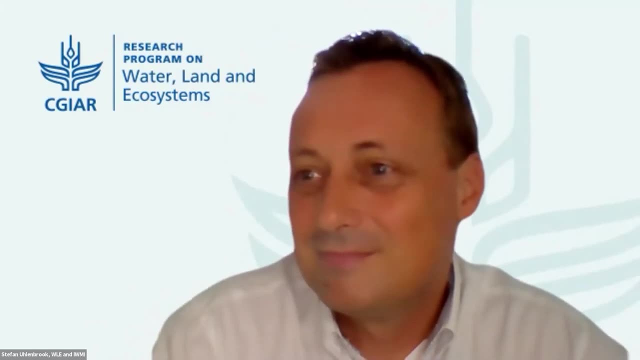 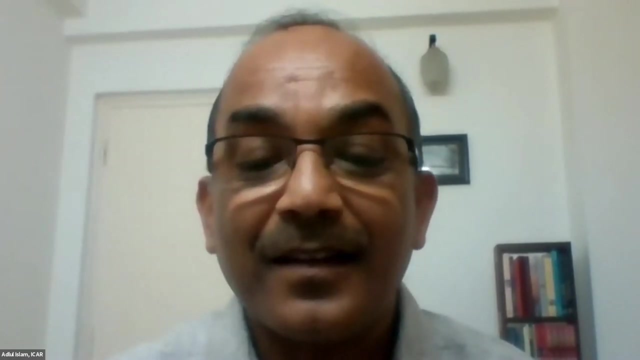 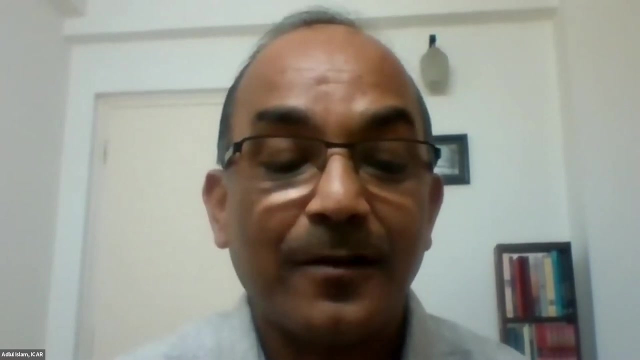 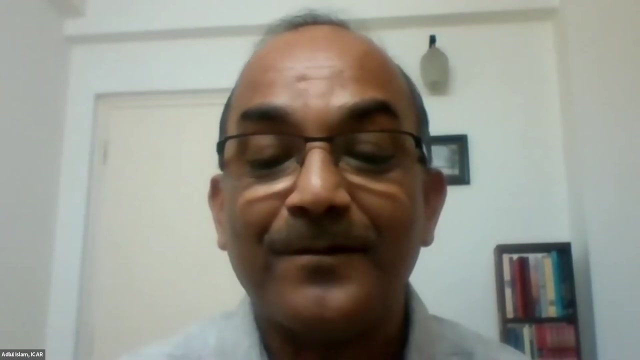 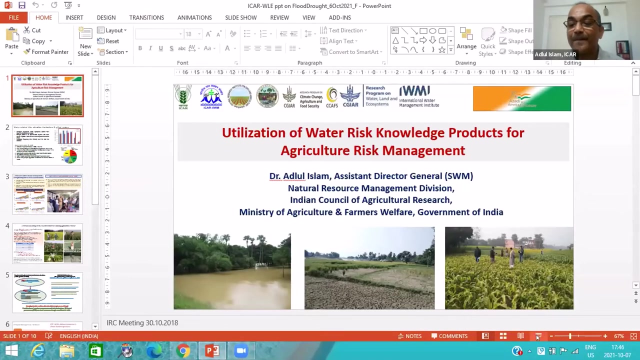 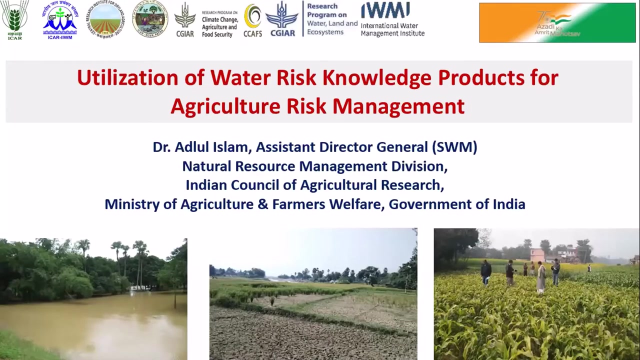 He has published some hundred plus papers and I'm very much looking forward to learn from him over the next eight minutes. Please, Dr Islam. Thank you, Yeah, Yeah, sure, Thank you, Stephen. So I'll be speaking on the water related risk knowledge. 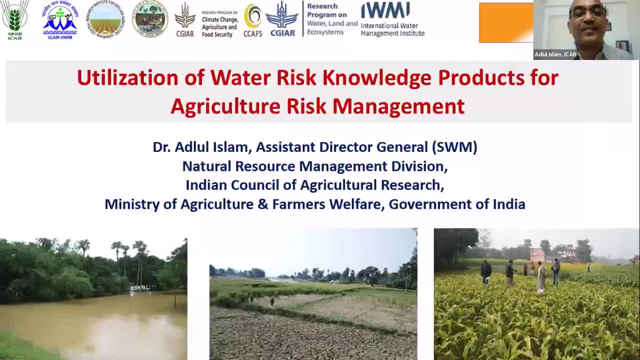 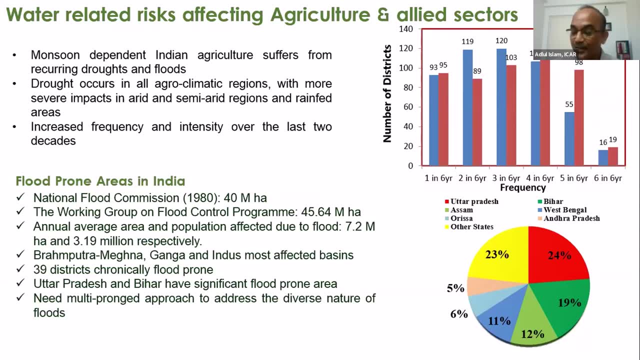 product in agriculture: risk management In India. drought and flood are the major water related risk affecting Indian agriculture. This drought and flood occurs at the same time in different parts of the country due to different climatic and rainfall pattern in different parts of the country, And in the recent years there is increase in frequency. 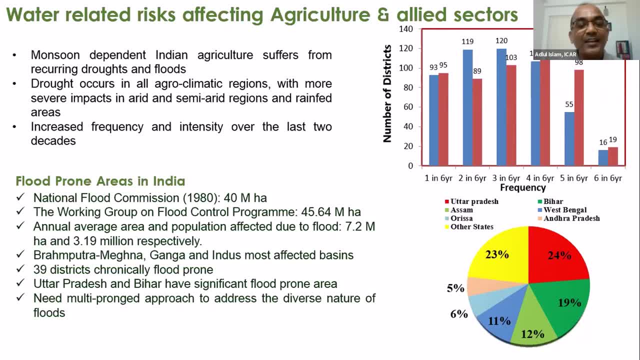 and intensity of these climatic extremes, and it is expected to increase further due to climate change. As far as flood prone area is concerned, in India, there are about 45- 46 million hectare area is flood prone and 39 districts are chronically flood prone, and 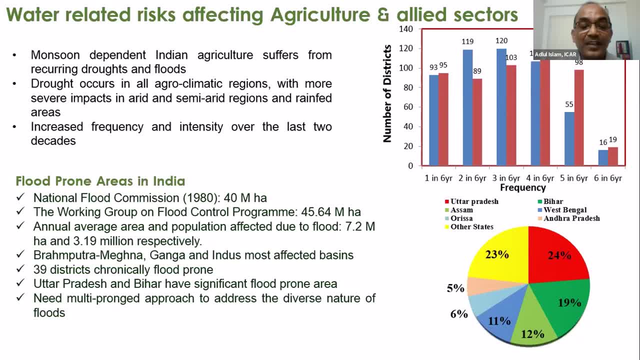 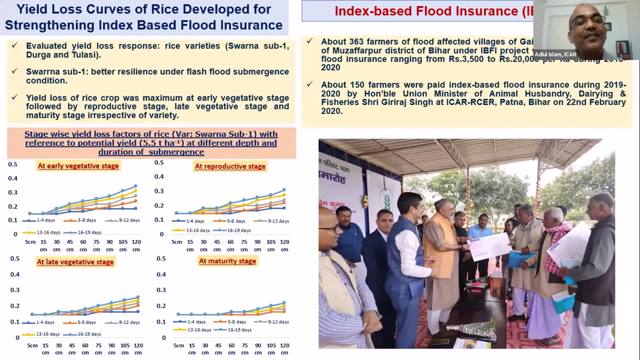 among the different states, Uttar Pradesh and Bihar have significant flood prone area. This drought and flood, these climatic extremes, cannot be stopped or eradicated, but it can be managed or its impact can be mitigated through different management strategies In this direction. 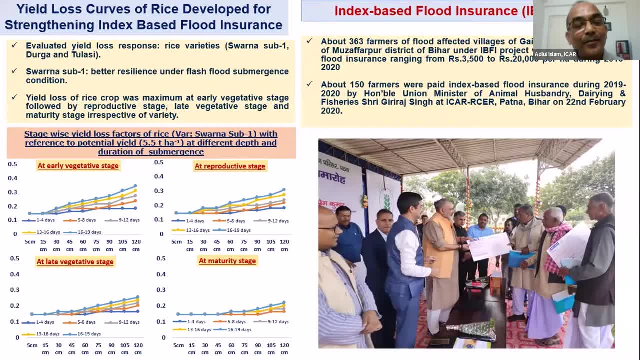 earlier the different major approach was towards engineering design of dams and dams, In this particular case the management strategy of dams, dams, reservoirs, etc. But now there is understanding that no even the management strategy like IVFI can be used. This IVFI index. 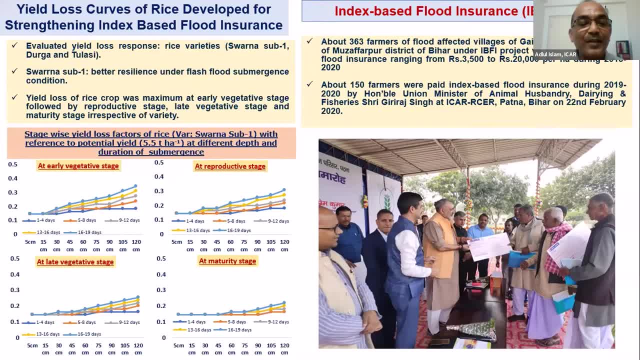 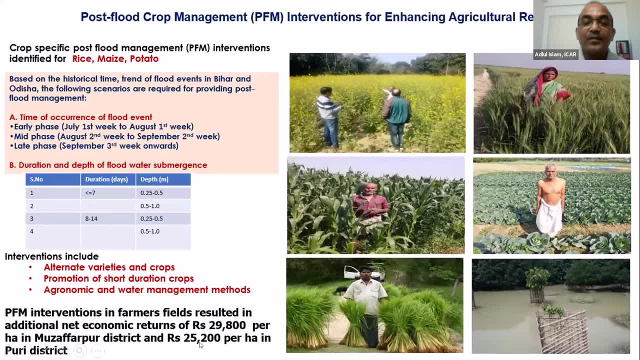 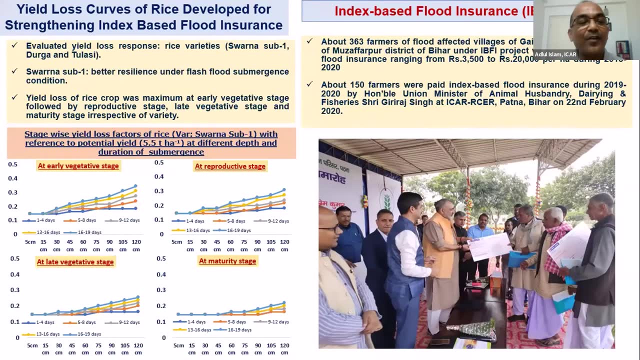 based flood insurance product has been implemented in collaboration with IWMI in India. So ICER is working in two different components in this IVFI product. First is the estimation of ill loss curve to decide the amount of payout to for compensating the loss due to the flood event, and another is the post flood management So for ill loss. 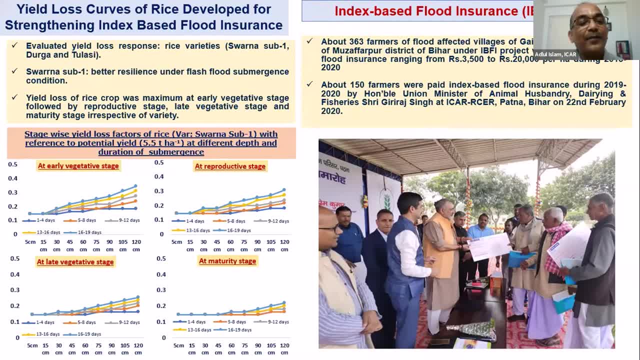 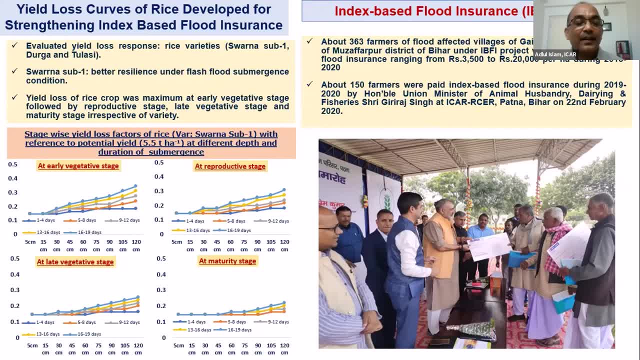 found to be best performing for climate resilience. So ill loss curve has been established for the different depth and stages of crop growth And based on this IBFI. this IBFI product has been implemented in Bihar and Odisha. This around 363 farmers have been paid. 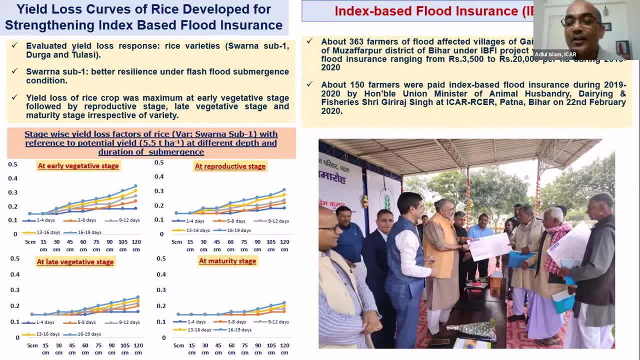 through this IBFI product and around 1.7 million Indian rupees, that is, around 22,000 US dollar, has been distributed during the 19, in three years period 1918 to 2020.. This photograph is of that. our union minister, Gita Singh. 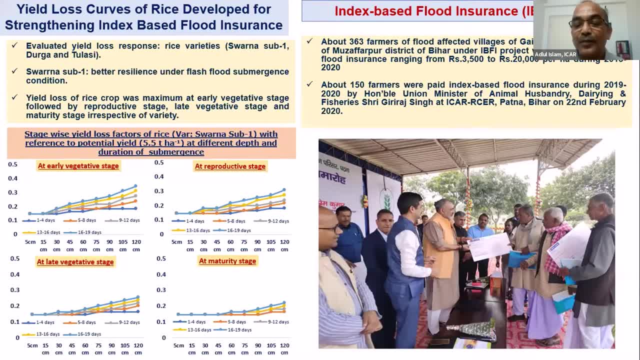 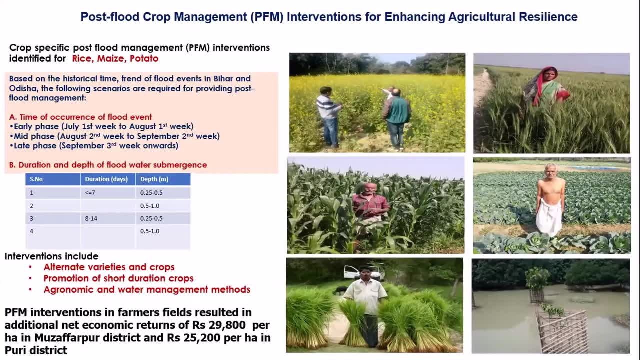 is distributing that payout to different farmers and this payout has been decided through this index-based plus insurance product. The second component: ICR is working on post-flood management intervention. Once flood has occurred, then to minimize the loss, the ICR is implementing different interventions. 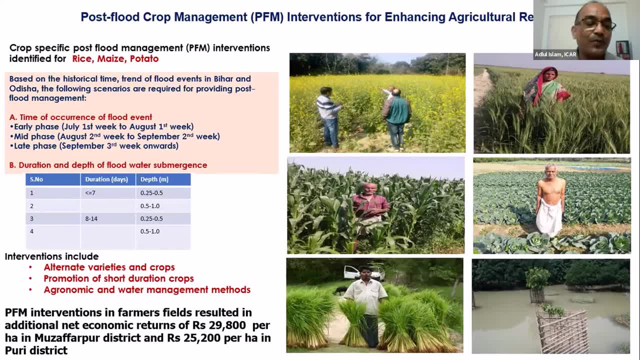 like alternate varieties of crops, short duration varieties of crops and different agronomic and water management interventions to raise the income of the farmers. This implementation of post-flood management interventions has increased the income of the farmers in the range of rupees 30,000,. 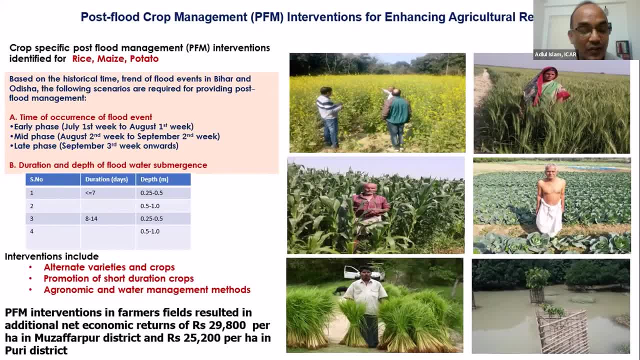 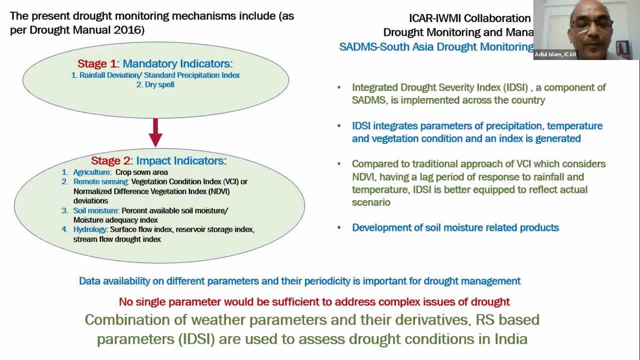 25,000 to 30,000 in different different districts. That is around 300 to 400 US dollar. Apart from this, drought, like flood drought, is another frequently occurring problem in India, and government of India has published the Drought Manual 2016. 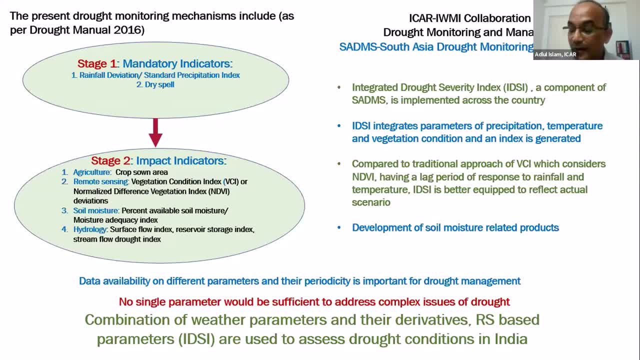 where, two or three years ago, the government of India has published the Drought Manual 2016,. where, two or three years ago, the government of India has published the Drought Manual 2016, to identify the drought areas or drought carbon areas. 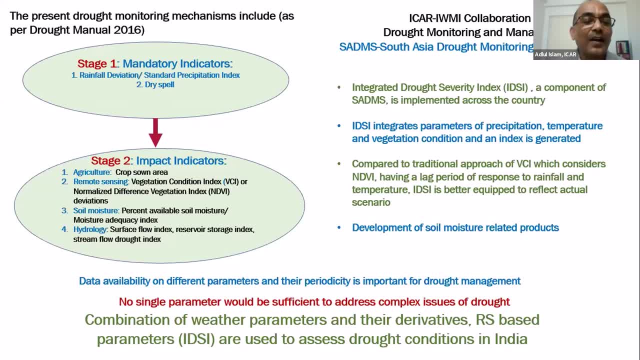 and different indicators had been specified, like in visitation state, that is, the rainfall deviation from the average rainfall, dry spell or standard precipitation index is considered. Once the rain occurs, then there is an impact on crops or and area vegetation condition- NDVI- as well as soil moisture availability. 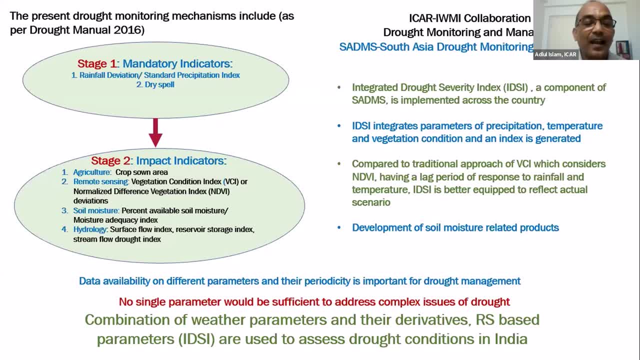 reservoir levels. So these are the different indicators assessed for weeks forि. Oliver said he wanted to see someone who will help on this. public comment- private comment- impact assessment. Now, this drought management manual also emphasizes the need for assessing the drought using different indicators through using GIS and remote sensing approach. 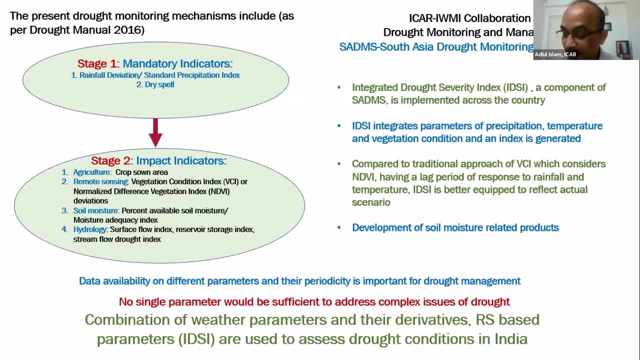 In this direction, ICR, in collaboration with IWMI, is implementing the IDSI index. IDSI is an index which uses satellite based product and other data and computes soil index, soil moisture index, precipitation index and integrate with other data to decide the drought severity. and this is 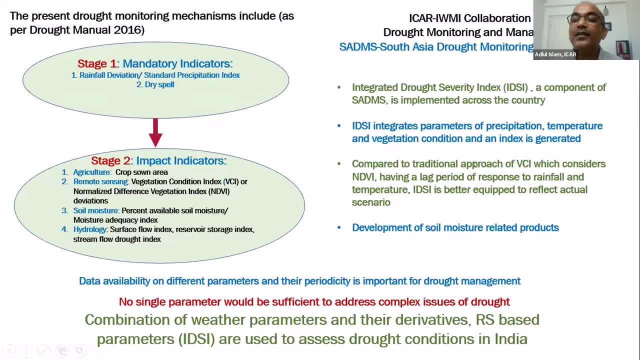 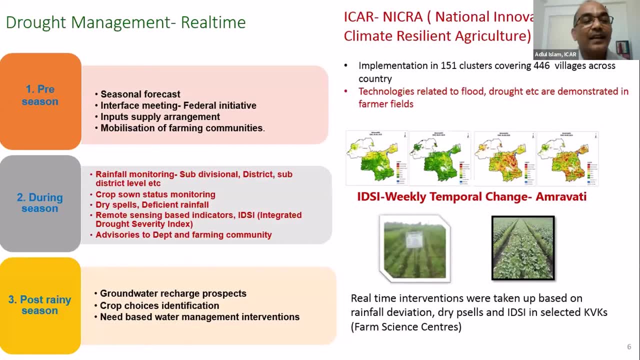 implemented through SADMS, that is, South Asia Designed Drought Monitoring System developed by IWMI In India, that the drought management is a continuous process. It starts with decision planning, like interface meeting, and then again monitoring different indicators during season and then again post decision monitoring: ground water recharge, crop choice, identification, etc. So the drought 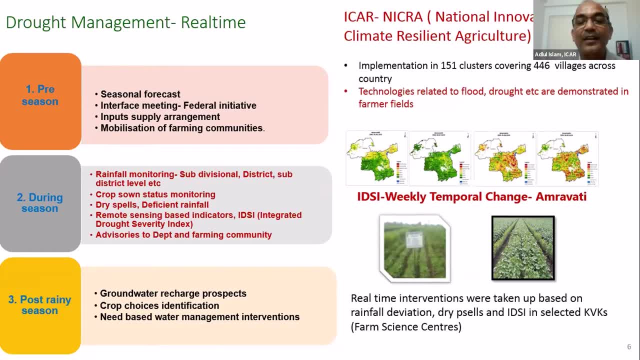 management is a continuous process. in India, government plan and ICR is implementing the another in flagship program, that national innovation on climate resilient. This program has been implemented in 151 cluster of covering 446 villages. So under this program, different technologies related to flood and 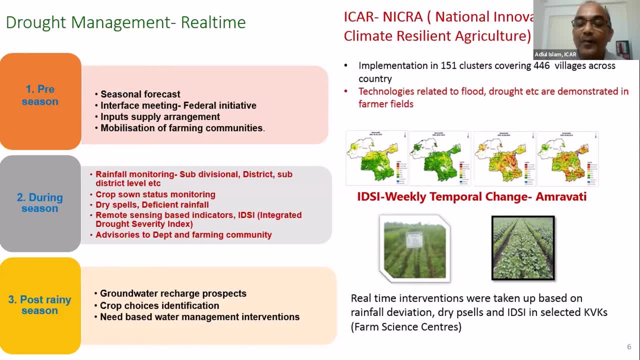 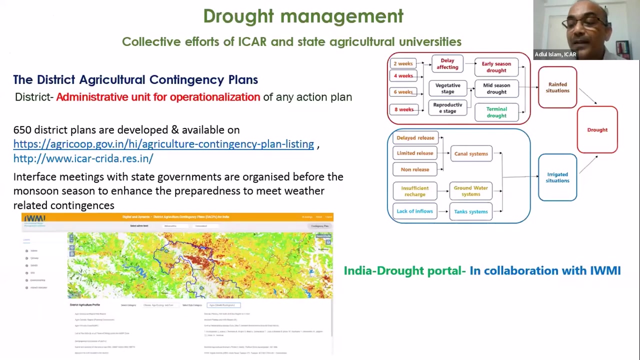 drought managements are implemented in farmers field. This IDSI product has also been tested through farmers service center, that is, KVK, in Maharashtra, Andhra Pradesh and Telangana states of India. Again, ICR has also developed district agriculture contingency plans to crab masih. 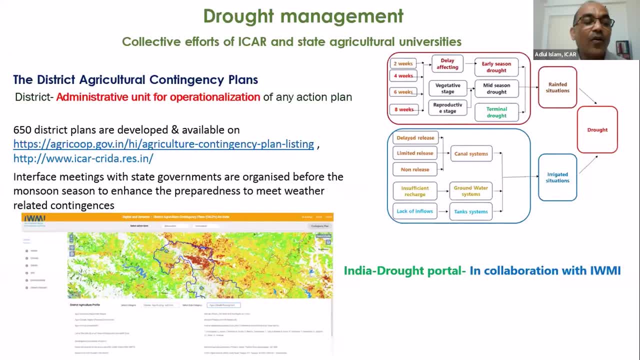 of climate, aeration and climate risk and all 650 district plan and�� Football, everything bigger. contingency plans have been prepared and implemented in different districts. Now there is also effort has been made to integrate the nature of satellite product along with this district control contingency plan pour all 50 Dustave. Interestingly, it is in their 이에요 St merit to use it to integrate Feather Cell Service. The from there are discussion of, not via infrastructure now model improvement, collaboration, etc. but what can I get into information across geologist the, the recovery sophisticated infrastructure elsewhere겨 have been involved here. 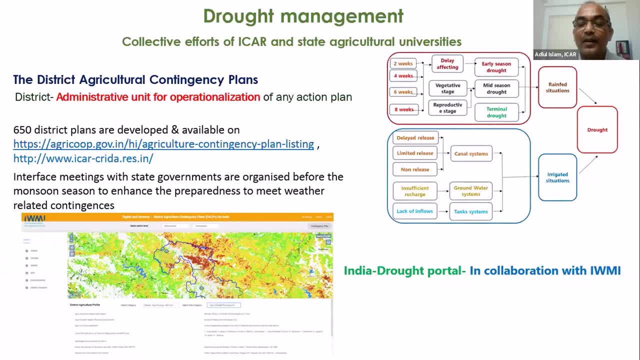 Our Ras scratched yours. had discussed precent nuestros refer plants. they are strong drivers, a result that both pe оч the question and I worked out that annual quick drive various thousands and many others. these elders were especially interested to think tremendously indigenous plants to prepare India Drought Portal in collaboration with IWMI. 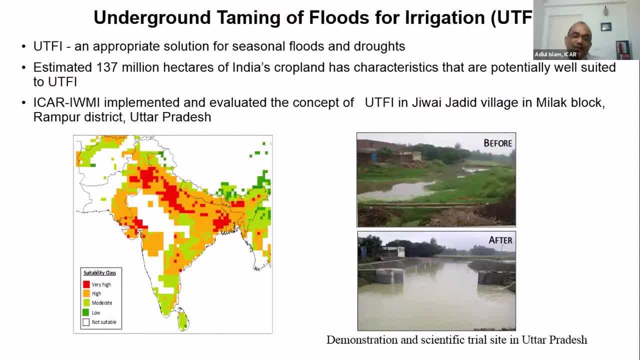 Apart from this, then ICR also worked with IWMI in another product, that is, UTFI Underground Taming of Flood Water, to address the issues of seasonal floods and droughts, And this has been implemented in the state of UP, Rampur district of UP, through in collaboration. 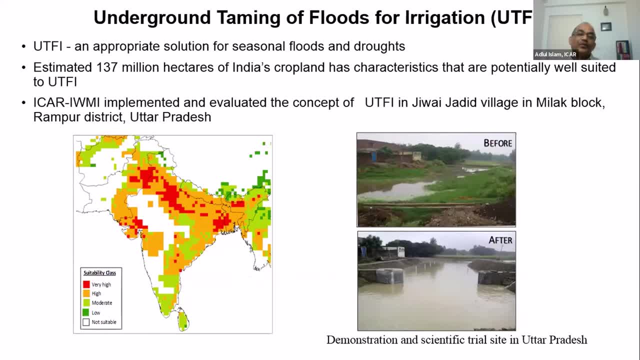 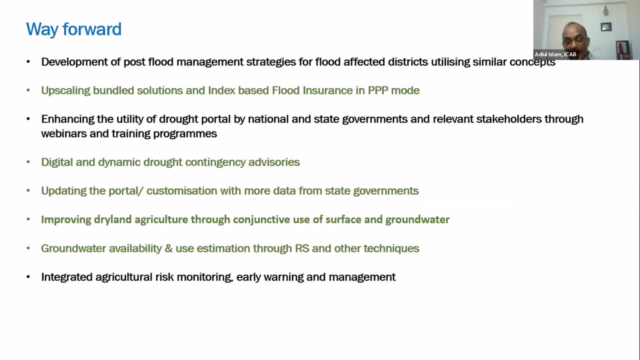 with IWMI. So way forward is that this IBFI, IDSI and this UTFI approach has already been tested in different parts of the country. Now there is need to develop post-flood management strategies For flood-affected districts, utilizing similar products and concepts, upscaling the bundle. 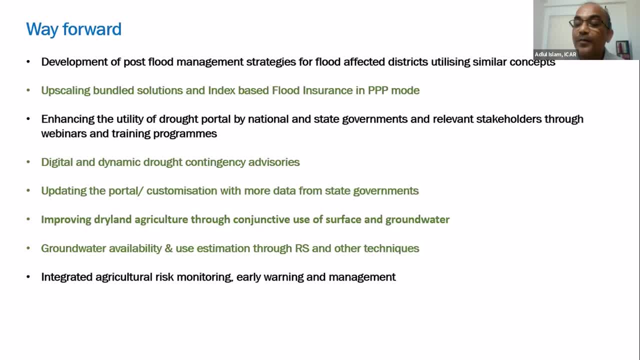 solution and index-based flood-sensitive product in public-private partnership mode. The IDSI product, that integrated Drought Severity Index product and SADMS- should be strengthened through the national and state governments data and through creating awareness about this product. Then again the dynamic drought contingency plans. already ICR is working on drought contingency. 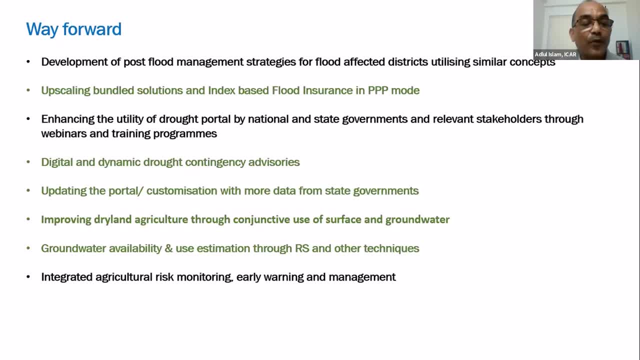 plan. There is need to use the satellite product and upgrade it to dynamic drought contingency advisories. Then improve dryland. there is need for improving dryland agriculture through of surface and groundwater for post-flood management. You have to round it up. 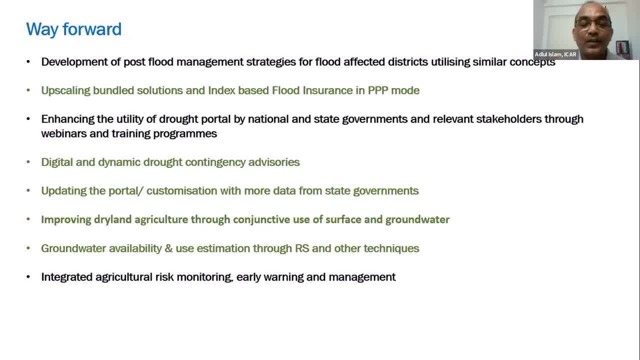 Sorry. And groundwater availability And use estimation using remote sensing other products, And also to consider the UTFI-like approaches for addressing the flood and drought issues And integrated agricultural risk monitoring and early warning and management approach. Thank you, sir, Thank you. 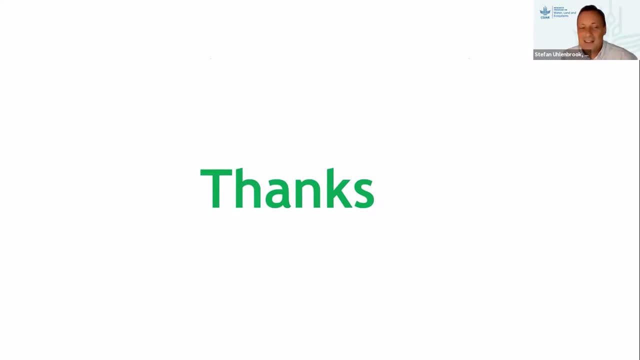 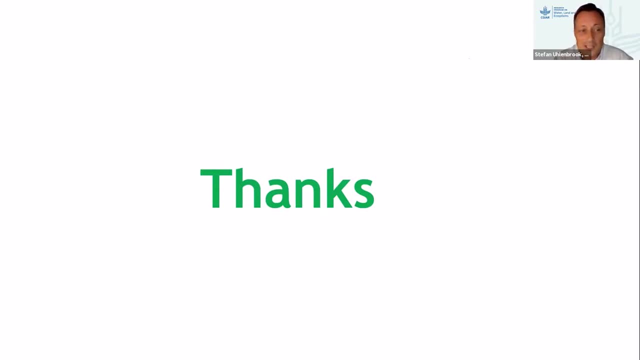 And he held so many senior positions in India before, among other things, the deputy director general of the ICR, director of the research complex in the eastern region in Pakhna. He was the coordinator of the Indo-Gangetic Basin under the CGR program. water for food. 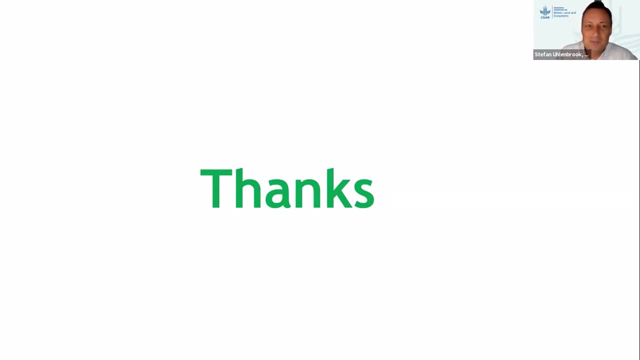 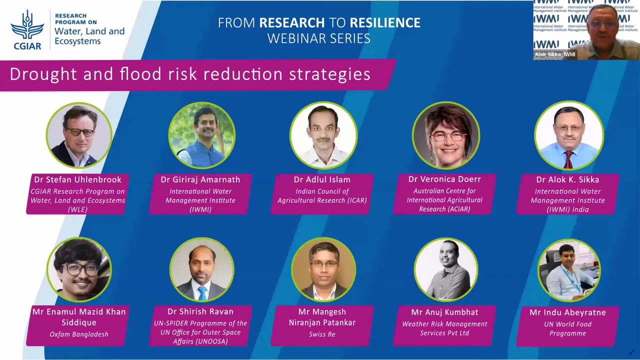 et cetera, et cetera, Over to you, Alok, Thank you, Thank you. Thank you very much, Stephan, And without any further ado, Because we have time, I know that we are a bit late, So I'll start inviting. first of all, let me thank the WLE and the organizer for having 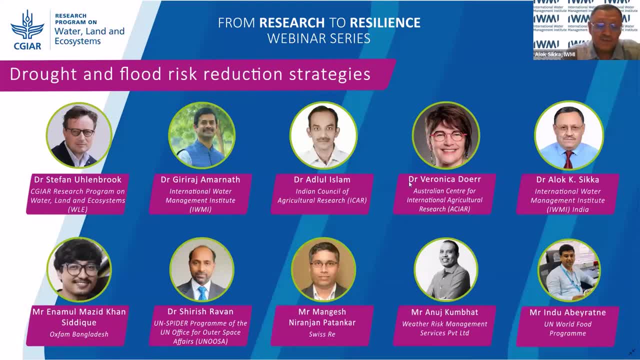 given me this chance to moderate this particular session, And it's really going to be an interesting session, but, of course, time is very short, So what I would like to now start with is, when we are starting with this, the possibility of this: 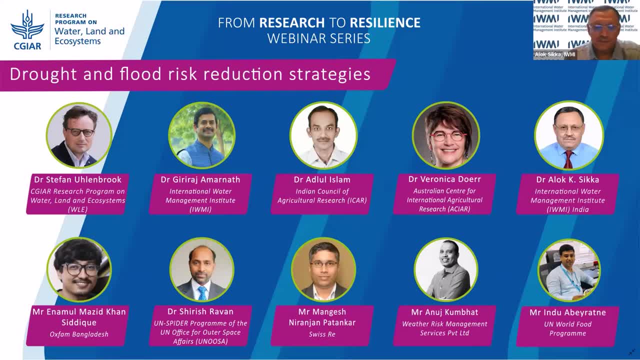 The possibility of the time. I would request the audience also that you can put your question in the chat And also the panelists can also simultaneously try and answer whenever they can. So I'll start with the first panelist, that is, Enamul Siddique, who represents Oxfam. 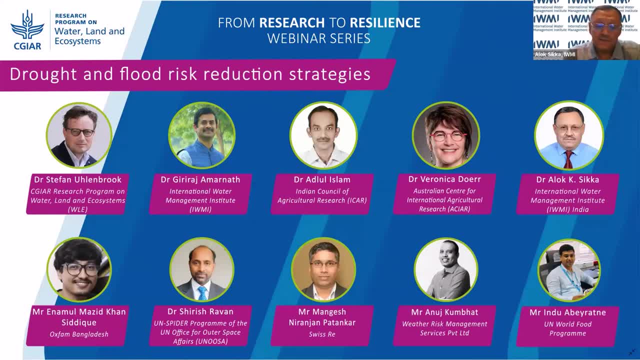 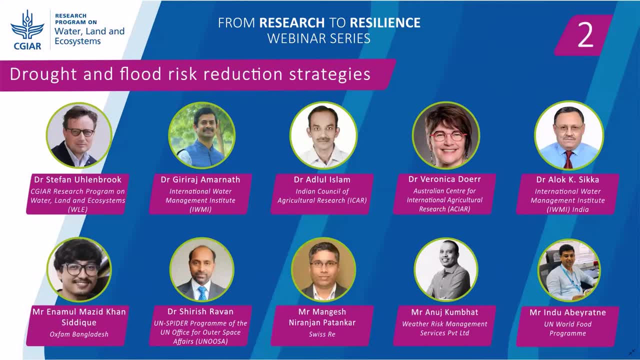 Thank you And Enamul. we would like to know from you if you could quickly describe the initiatives of index-based flood insurance as a collaboration with WLE and IWMI and Oxfam, And the connected question with that is: how did this solution unpack the challenges of? 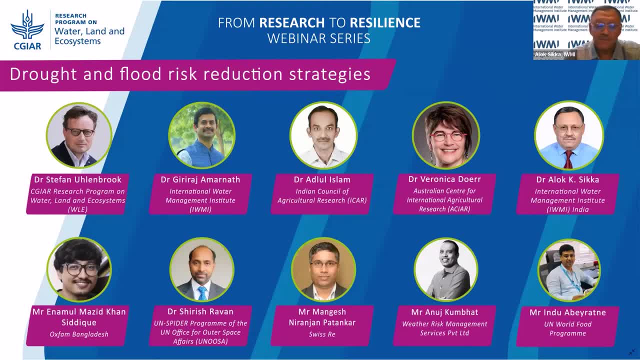 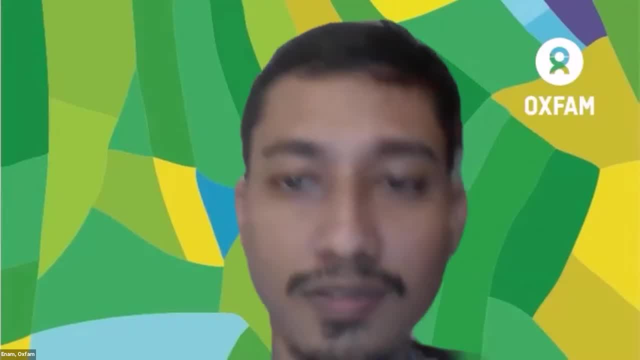 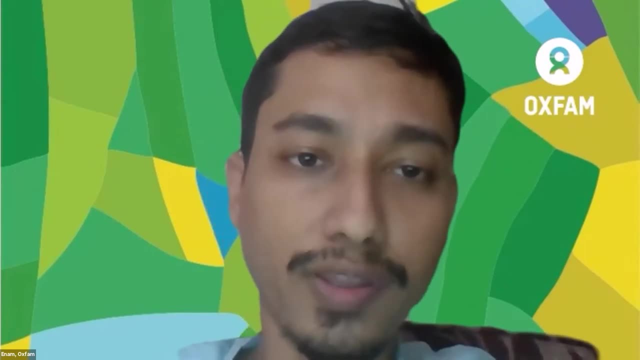 financial inclusion among the vulnerable social workers, vulnerable social groups, and so over to you in animal place and you have three minutes. thank you, doctor. so, uh, i'm working for oxfam in bangladesh and uh, the communities that we work with are most marginalized, which includes the farmers who are affected by floods every year. 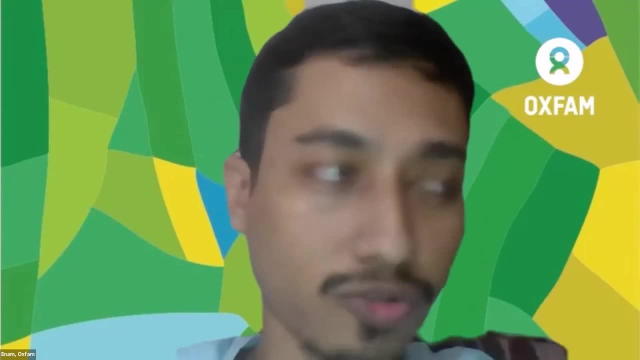 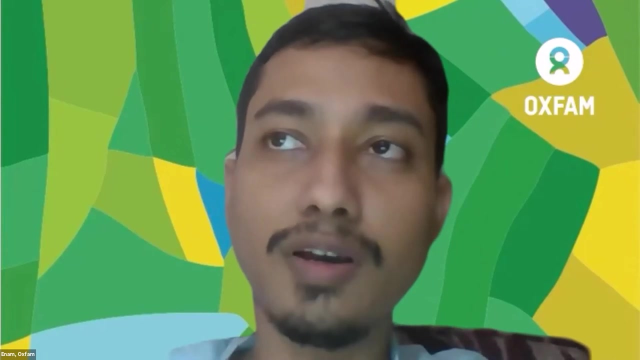 which includes the flash floods and the other seasonal plots, especially the monsoon right. so we have been, we have been uh working on on a on a solution, especially with index-based flood insurances, uh with farmers, and iwmi is a key partner in it because, uh the way the data needs. 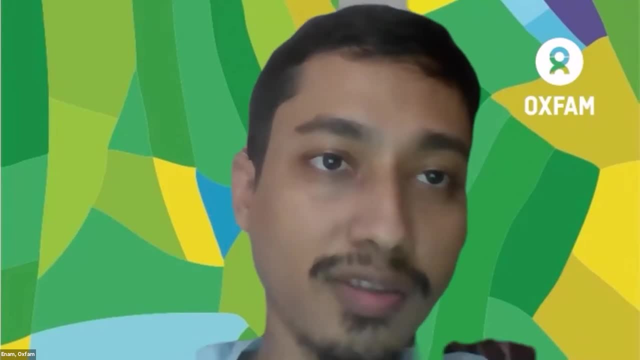 to be interpreted- to convert them into insurance products. that's where we depend on iwmi support and i think there is uh many things that we have already done. if you talk about the financial inclusion bit of it, i think it's it's larger than data. it's also about affordability and 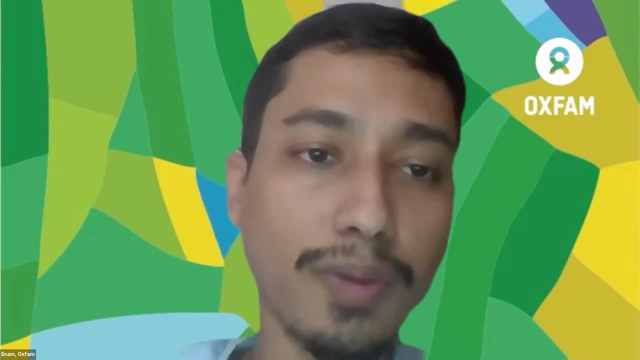 climate justice, which we need to resolve- but if we talk about how iwmi is linked with that. so so far, our collaboration with iwmi enabled us to support insurance companies and community members to get access to that data and convert that into insurance products, but it is not. 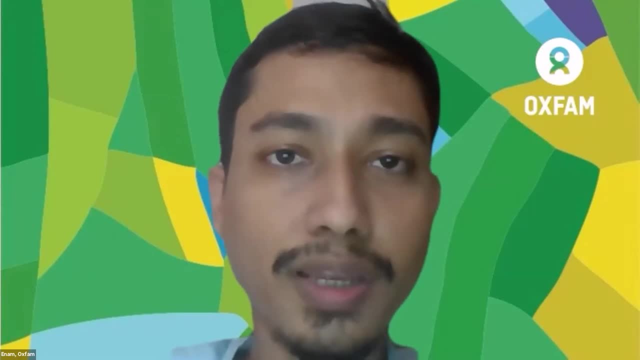 accessible for all the data that needs to be linked with insurance products. i think to make that more democratic and accessible to everyone we have to go some extra miles, uh, going forward, but so far at least we have tested a solution which can be implemented with the right resources. 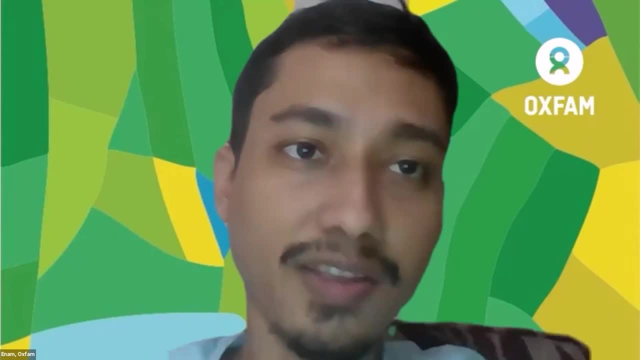 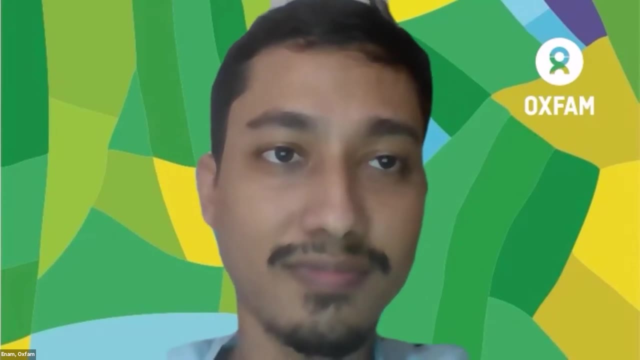 behind it. i hope that answers the question of signal. yeah, thank you. thank you very much, nanuel, for being so precise and being so much well within the time and, of course, if inshallah the time permits, i might come back to you again during the q and a. 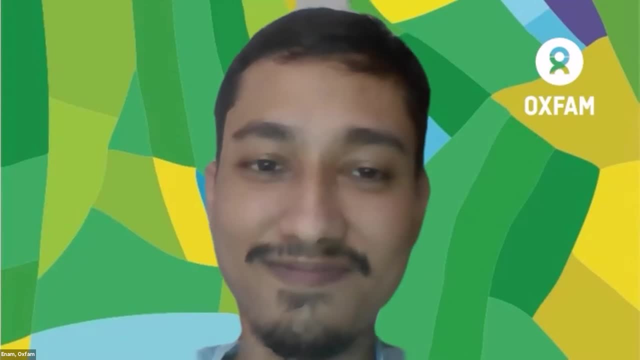 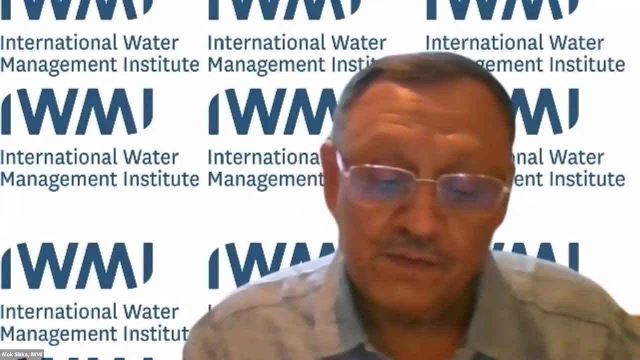 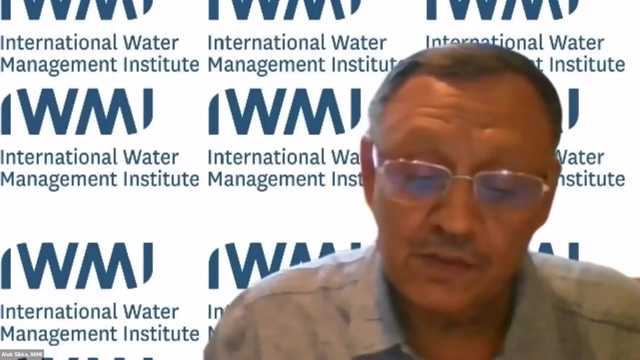 So, moving on to the next panelist, Indhu Avarathane, who is a national program officer at the World Food Program Sri Lanka. And, Indhu, we'll be happy if you please let us know how you are directly supporting the government of Sri Lanka and your collaboration with WLE on the climate and food security outlook. 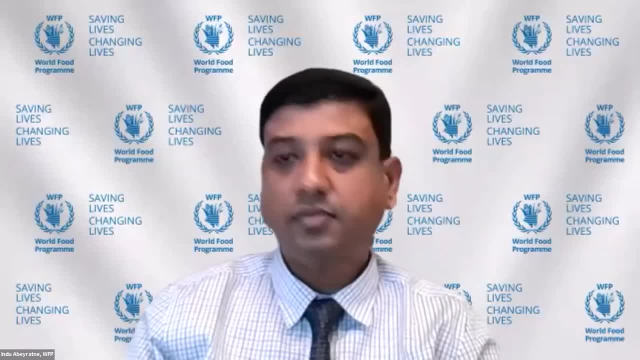 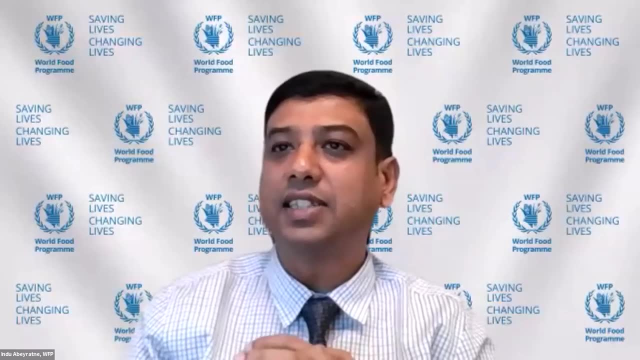 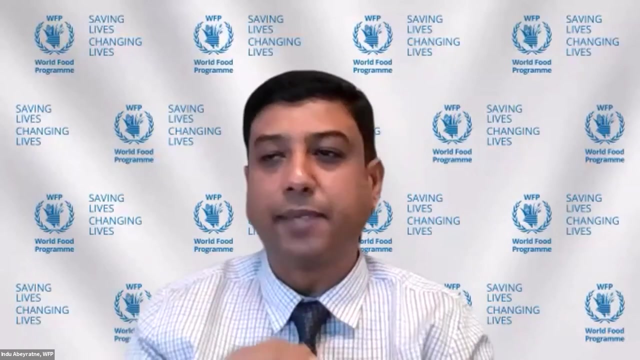 My first question and then please go ahead with that. You have two minutes for that. Yeah, thank you very much. Good evening, colleagues. You know, across Sri Lanka, the climate-related weather anomalies resulting extreme weather events, and it is becoming increasingly normal now. 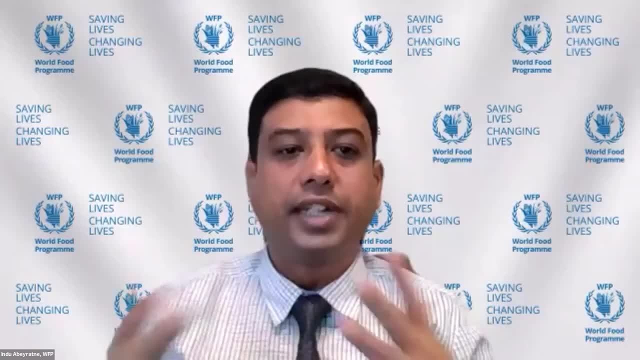 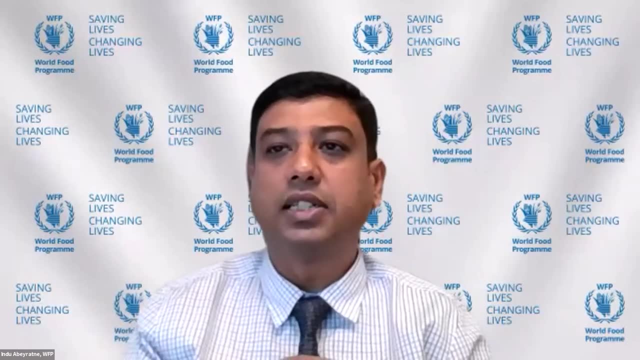 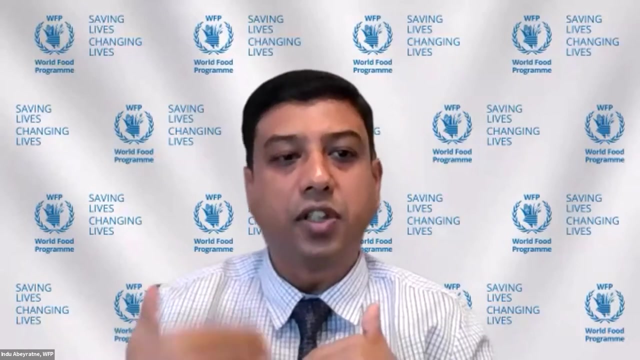 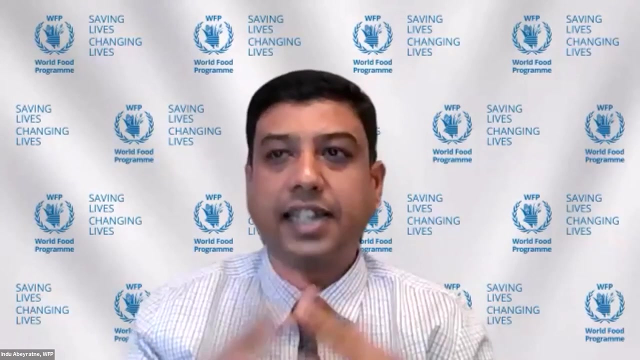 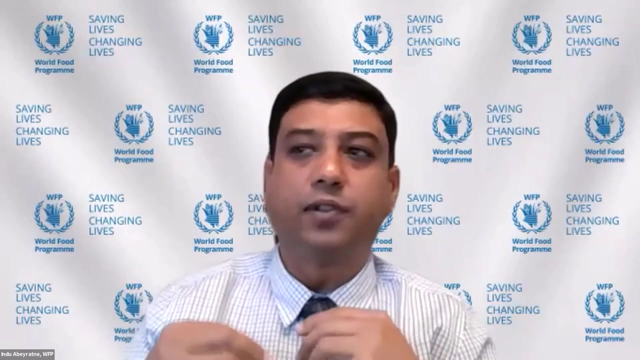 So this impacts, you know it impacts the country at large, but the farmers, agricultural workers are worst impacts due to these variabilities. I mean increasing Frequency of plants, droughts, flood droughts together. so these incidences in the last 10 years, you know, decade or so, if you see that it creates a severe, you know- hardship for the poor farmers across the country in various seasons. 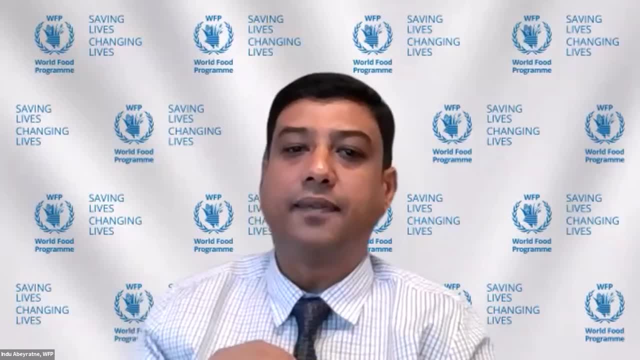 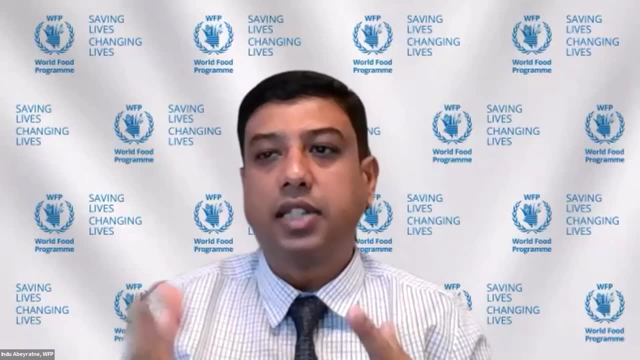 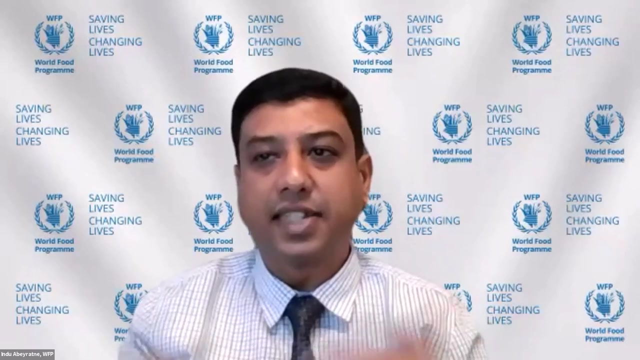 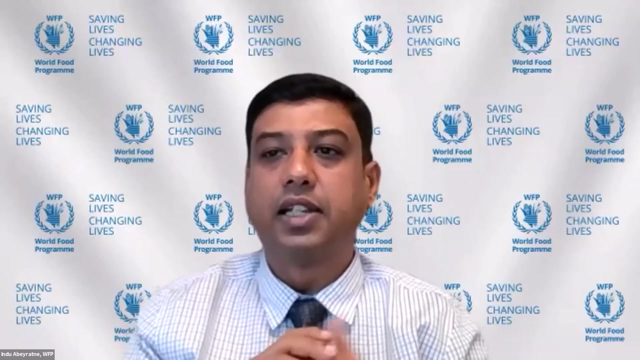 I mean this shows that link between the climate change and food security you know mostly explored. We've also seen, you know, the, you know macro movements on agriculture are also working towards impacts on water farming, agriculture production, irrigation and various other things which are linked to market chains and then, of course, eventually largely security. 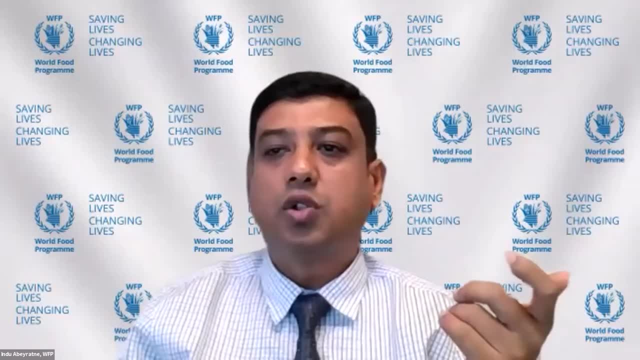 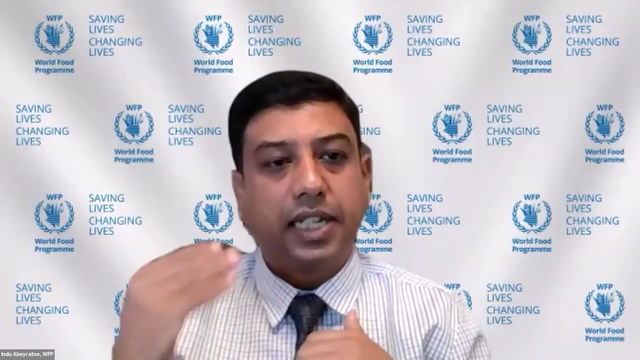 Now the important factor. so what would be the strategy over coming this? and there are certain challenges as well, but it always which we found that early information right. So what could be the strategies over coming this, But it always which we found that early information is very important. 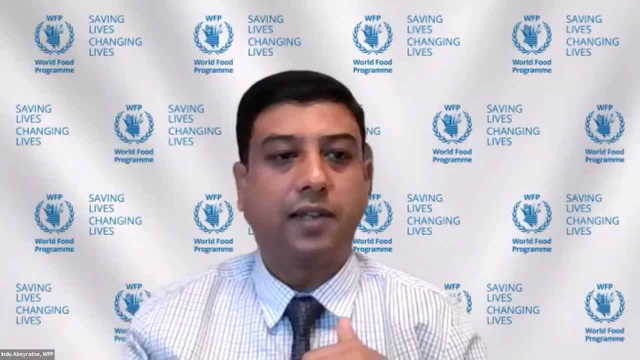 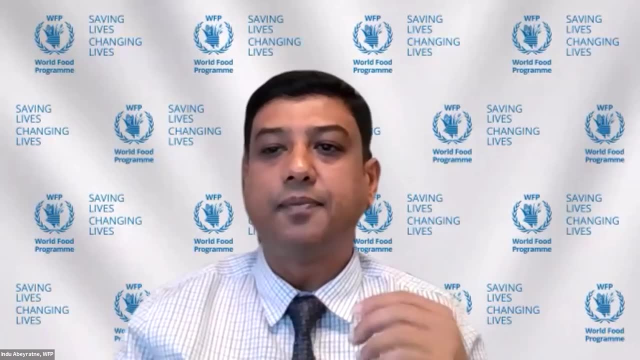 Thank you, Thank you very much. Okay, Thank you very much. Thank you, Thank you, Thank you. information is a crucial factor for evidence-based decision-making, which is somewhat of a solution in this, and especially analyzing different types of data and bringing harmonized you. 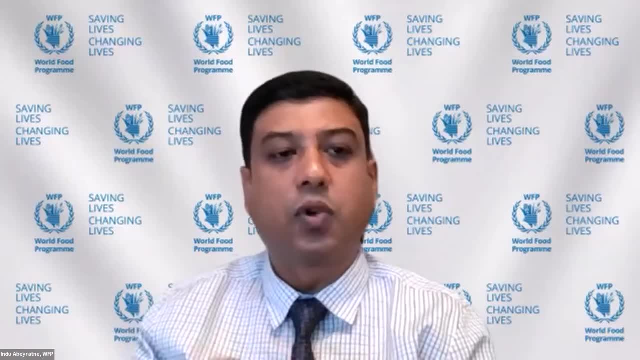 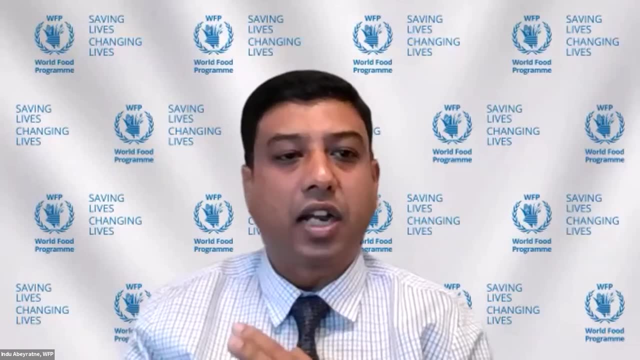 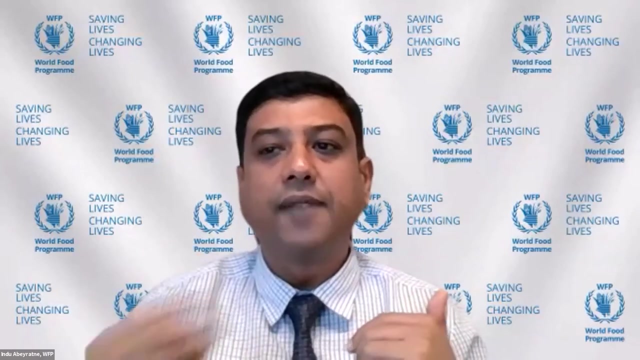 know, collated information, where that decision-makers and of course, the planners could take certain decisions at the ground and, of course, providing certain services to the agriculture, irrigation and you know, users, various livelihood groups as well, What WP is really doing: working with government, collaborating with meteorological agencies, 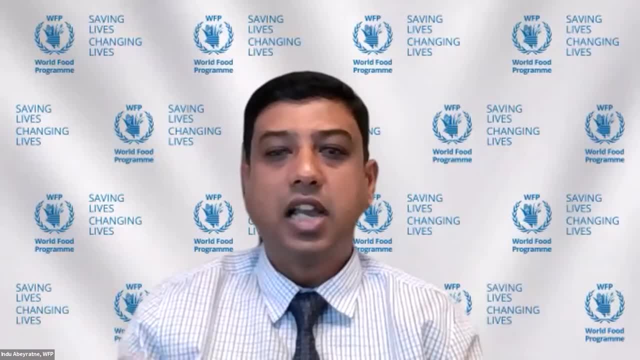 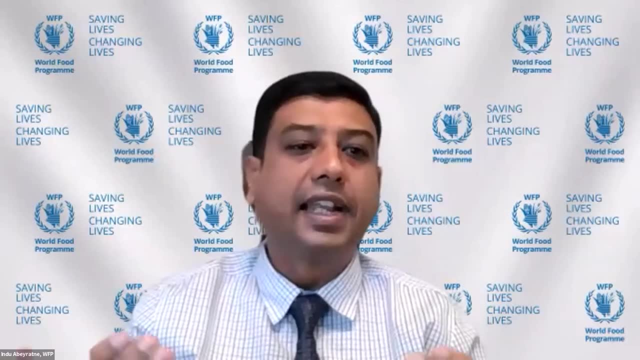 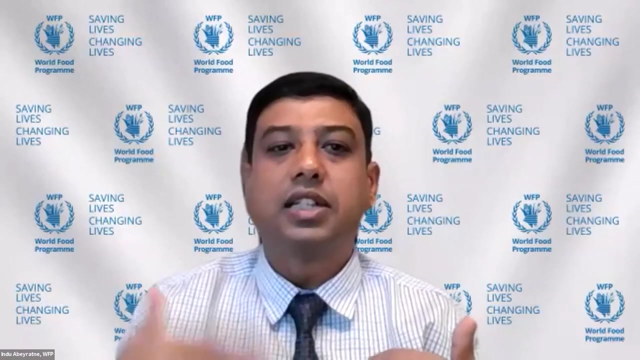 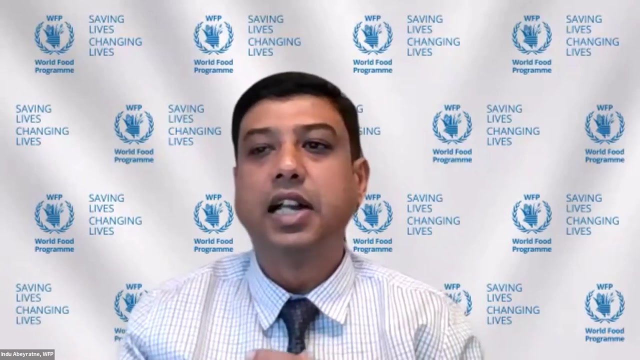 agricultural agencies, agrarian market chain and, of course, the IME, especially on the technical aspects, bringing them together, facilitating to bring certain information where we can analyze it together and produce certain information outlooks. We jointly produce twice a year a bulletin called Climate and Food Security Bulletin. 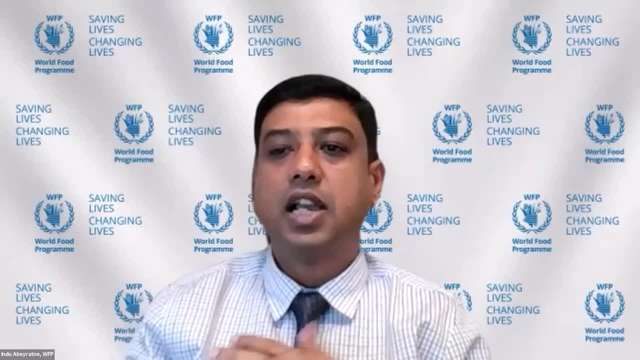 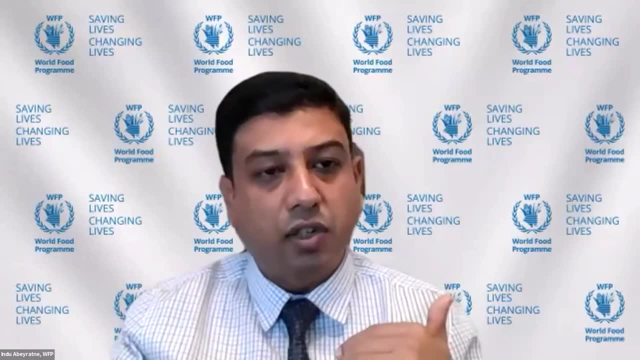 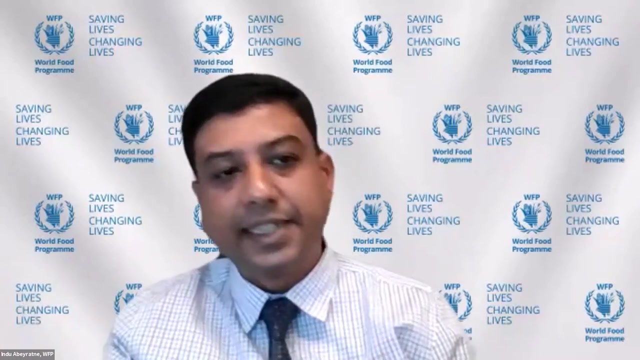 which IWMMA is part and partial of that. So this bulletin looks into key aspects of climatic and seasonal trends and their impacts on food security and, of course- which is, you know, leaning to the next season as well- how the next season is going to play out. 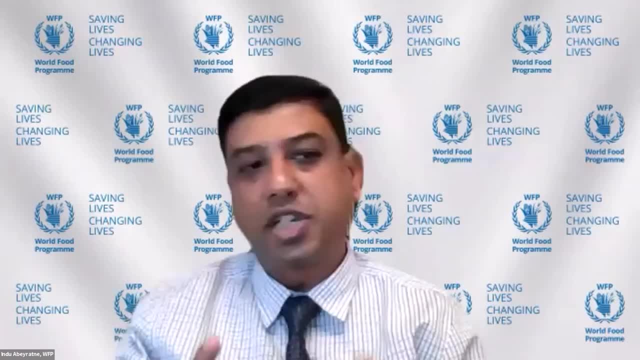 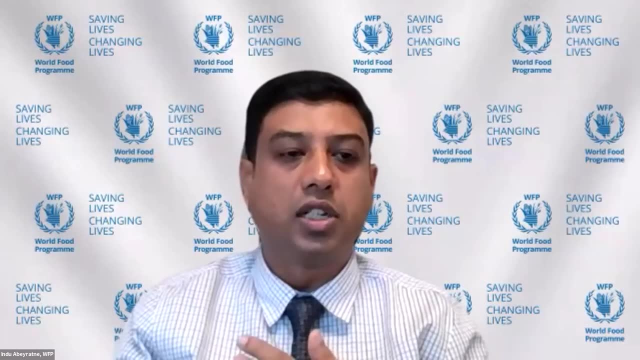 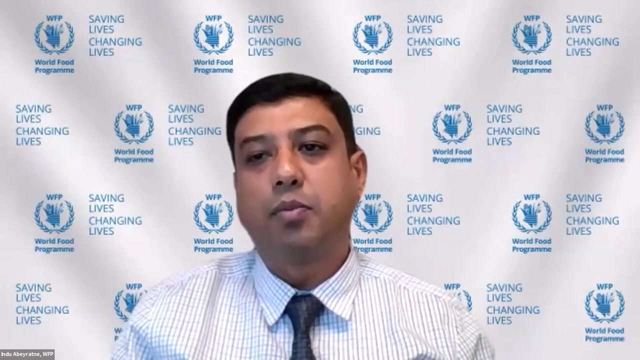 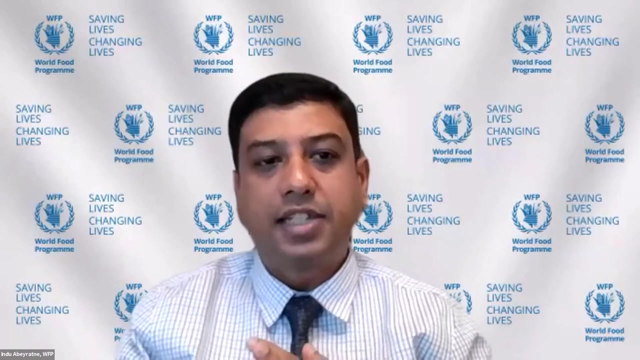 What WP looks like. So, all in all, all this information are collated together, which will be disseminated to appropriate channels and used in various, you know- strategic planning as well as day-to-day activities as well. So this is how that WP is providing and facilitating this particular, you know, technical know-how. 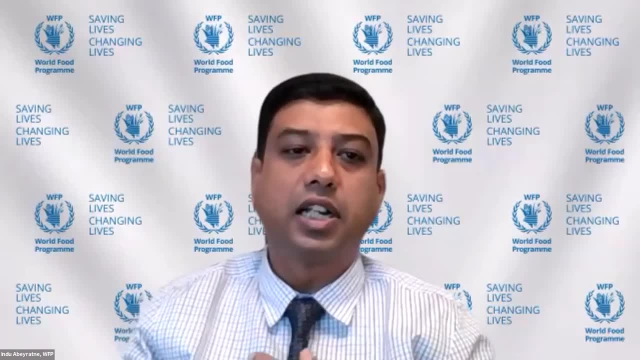 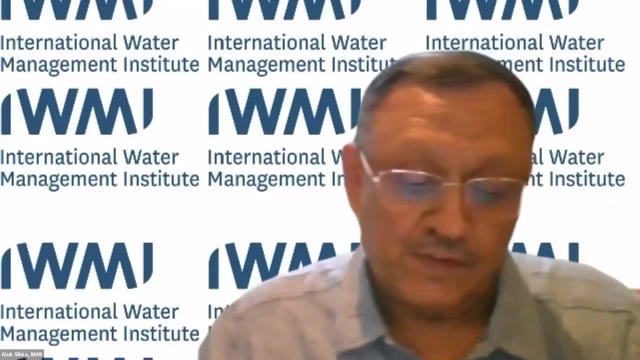 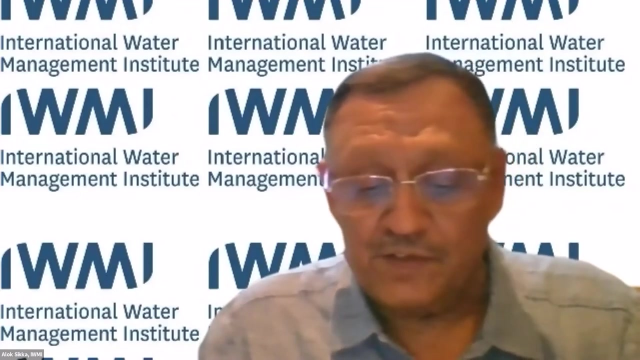 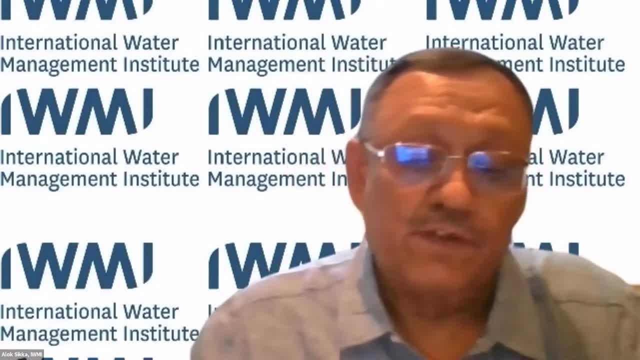 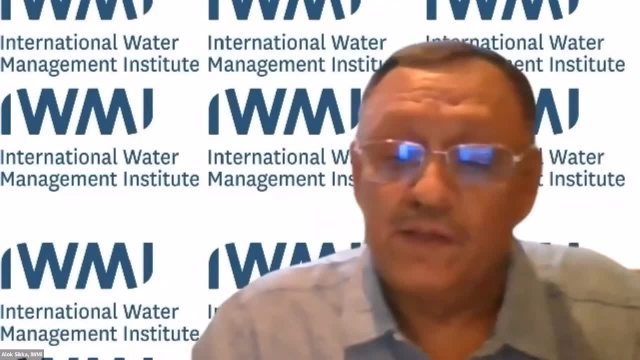 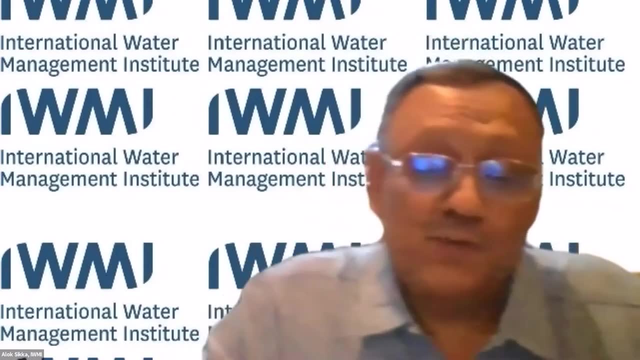 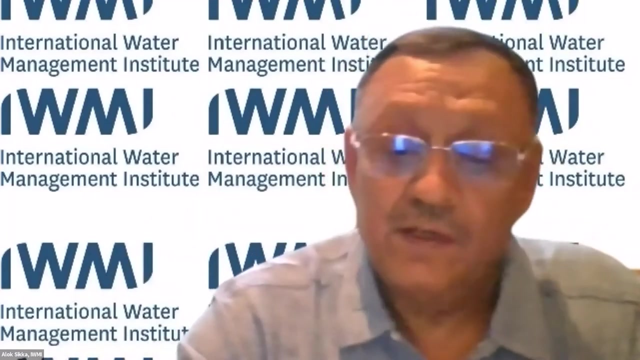 based technology, And for this I invite Sirish, who is heading the Beijing office of UN SPDR program of the USA. And Sirish, what we would like to know is that, as you are leading a very important disaster risk management initiative in Asia, and so can you briefly explain the UN SPDR platform? 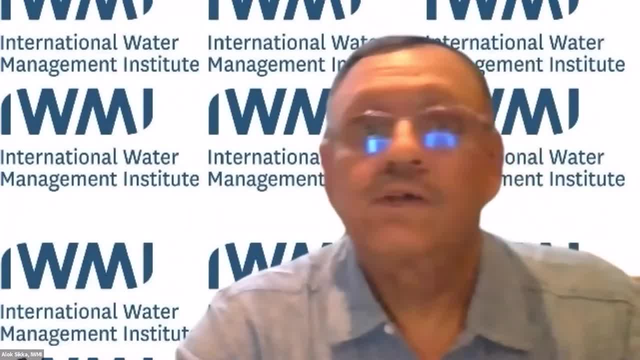 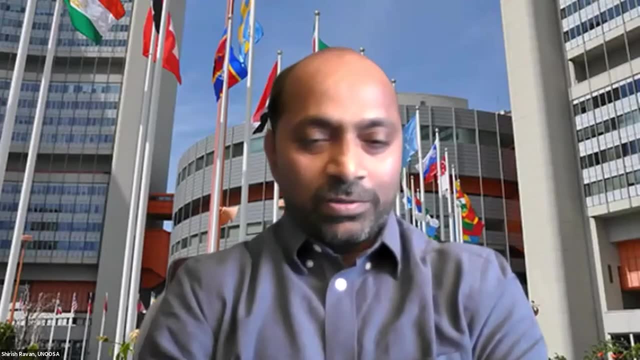 and how it facilitates the use of space-based technologies for disaster management and emergency response. with your vast experience So over to you, Thank you. Thank you, Sirish, And you have three minutes. Thank you, Dr Alok. So it's my pleasure to be on this platform today to share my experience here. 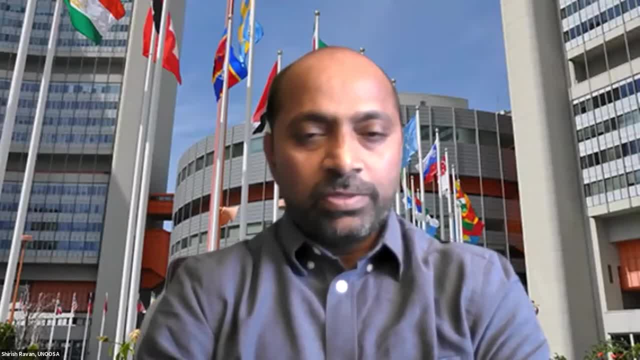 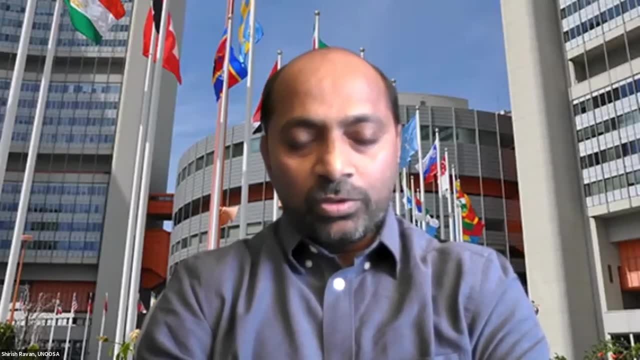 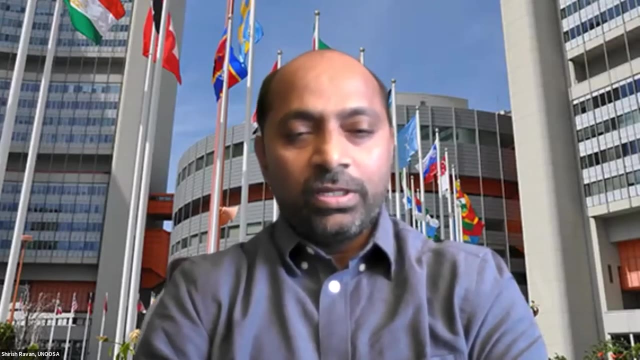 So, as you know, UN SPDR is United Nations platform for space-based information for disaster management and emergency response. So our job is basically to make sure that all the countries, mostly developing countries, use all types of space-based information effectively in all phases of disaster management. 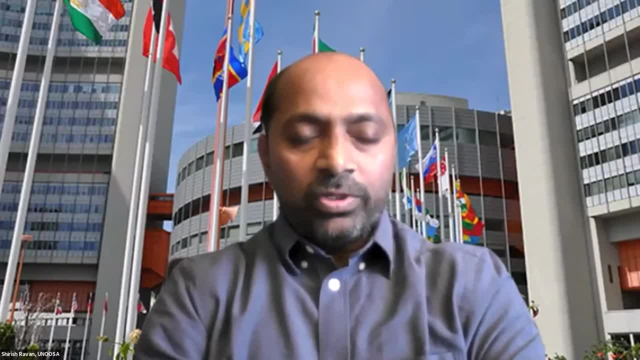 management and to that extent we have- uh, we are doing our interventions at at global, regional and also local, at country level. so at global level, i would say that we have been really very active in contributing to sendai framework. and if you look at the sendai framework and priority one and 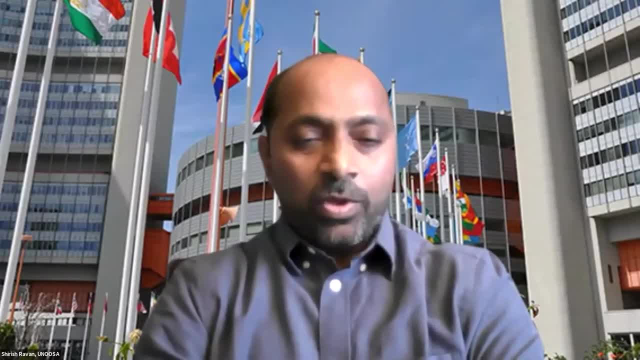 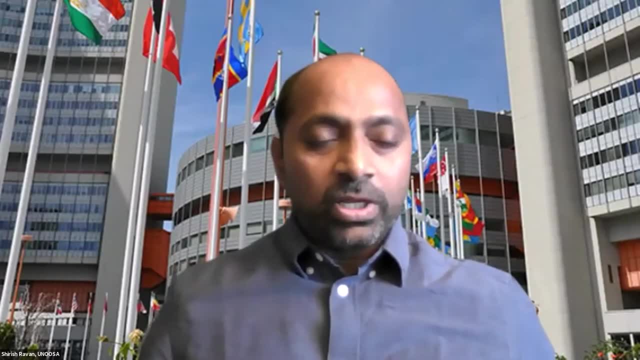 priority four. you can see there is a very clear mention of what uh how earth observation and geospatial information can contribute in achieving targets of sendai framework. so that advocacy has already gone at global level and the impact is very good because of that mention in the sendai. 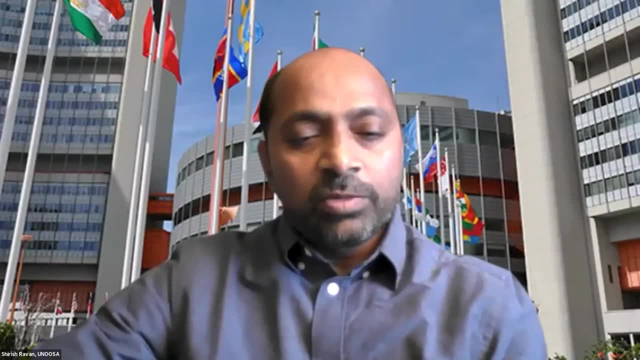 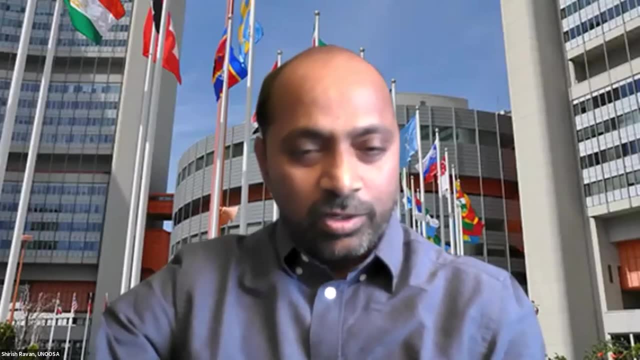 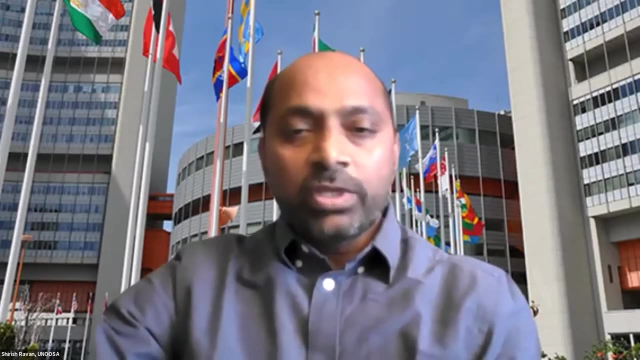 framework a lot of other national disaster management agencies who are preparing their disaster management strategies. they include use of space-based, geospatial and high technologies in their disaster management strategies and plans, and once it is in plan, we can see that it gets into action also. so that is what, uh, we have done at global level and we also advocate. 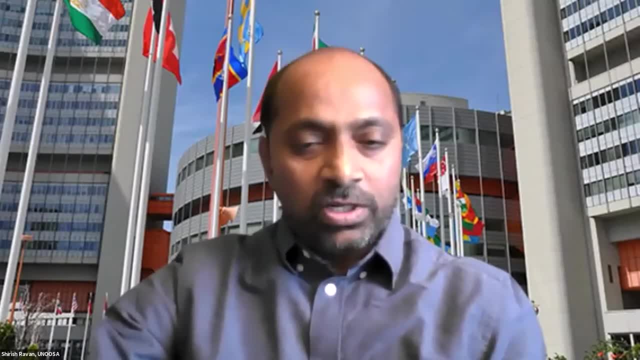 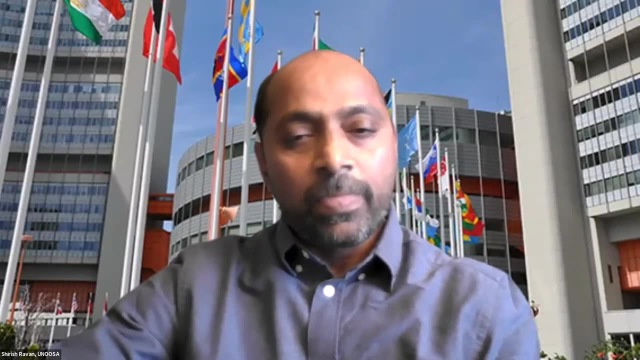 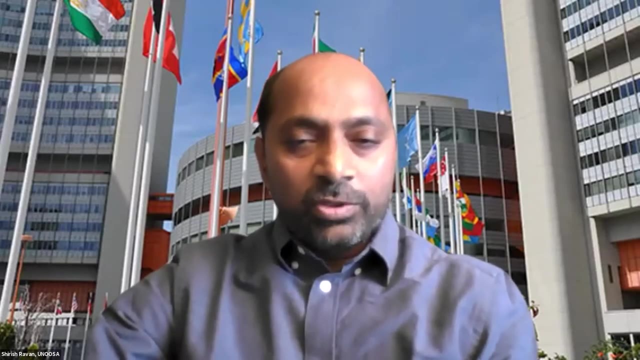 all the countries in how you can use space in achieving targets for sendai framework at original level. we have established no kind of standard platforms like with south asia with sharp disaster management center. we conduct regular training programs on various aspects and international water management institute and giriraj team is always has been part. 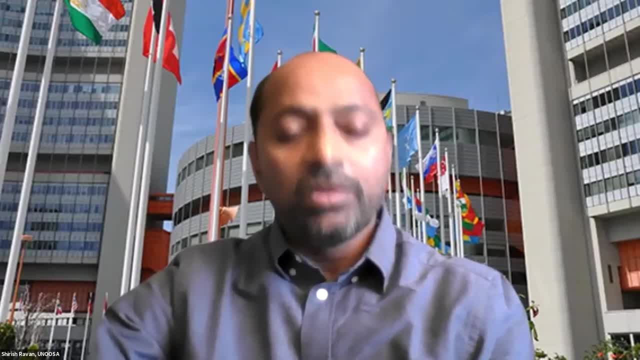 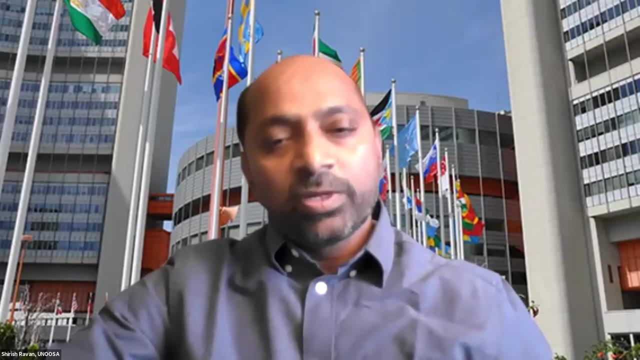 of our program and we have conducted almost like five, six programs and it is going on as a kind of a routine interventions at south asia. uh, we also have other interventions, like we conduct training international and global level in asean region or also for member states of absco asia pacific space. 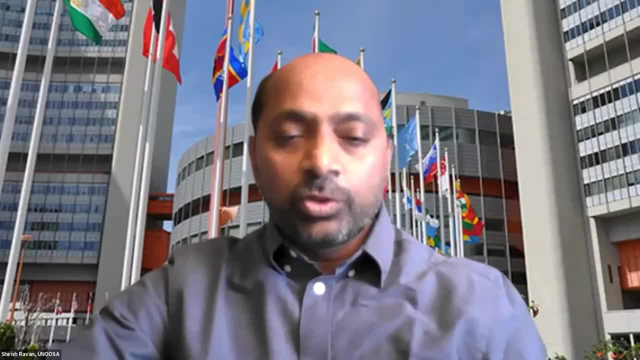 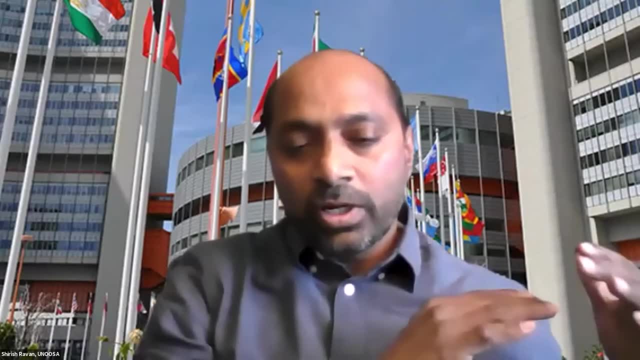 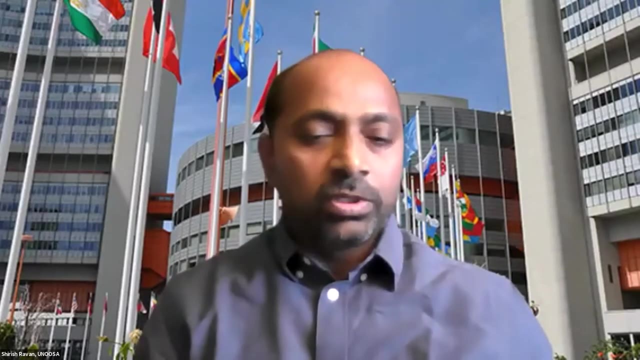 cooperation organization where international water management institute contributes. so, uh, basically, just to summarize in two lines, i can say that the interventions go at international, global, uh, the regional and national level, through advisory missions to the government, engaging with the national disaster management agencies, basically to build the resilience, how they can use the 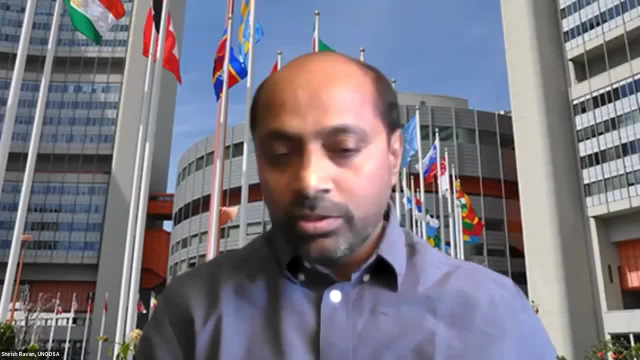 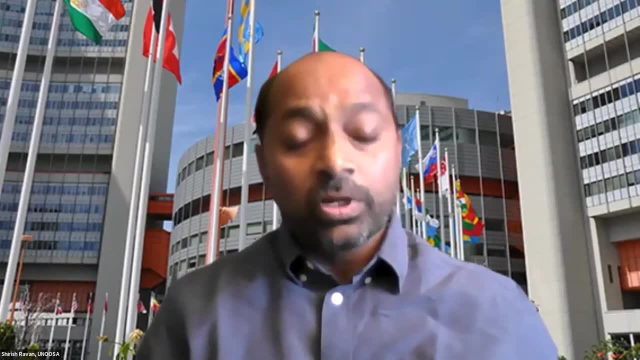 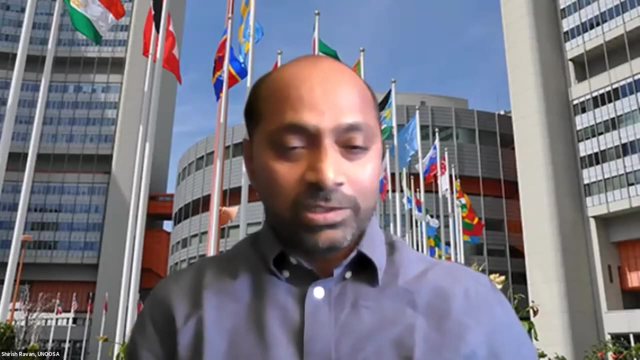 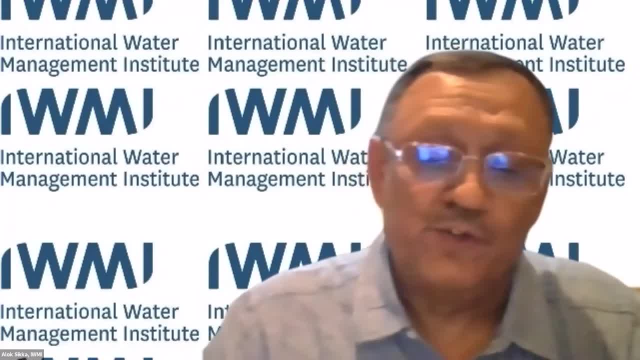 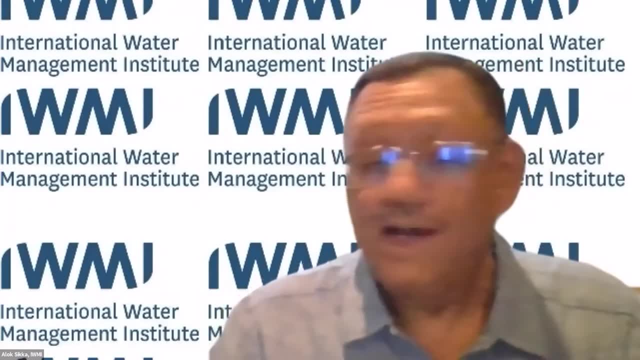 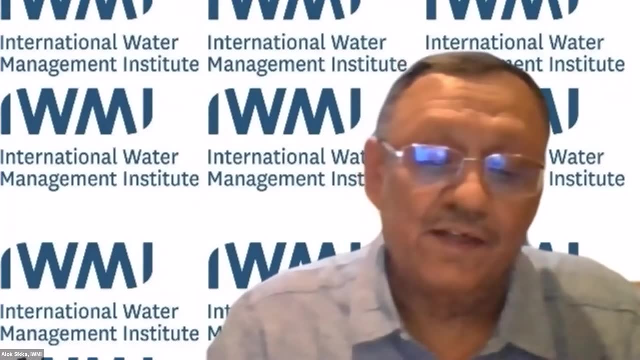 because for the q a. and so now i move on to a very important player who gives money to everyone after the damage happens. so, mangesh, and mangesh is the head of the agriculture, india, swiss re- and he has been working with us. so, uh, mangesh, you have been collaborating with the. 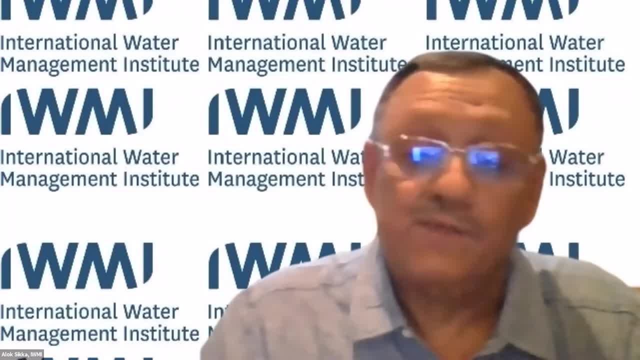 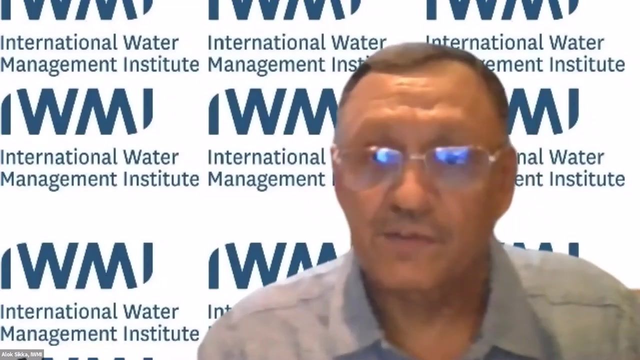 eme and wle on the development of index based flood insurance. so how do you see such a high-tech initiatives and the index helping farmers and the government broadly, and what are the opportunities and the challenges for scaling such a solution in the flood-prone nations, including india and other nations? so over to you for three minutes. 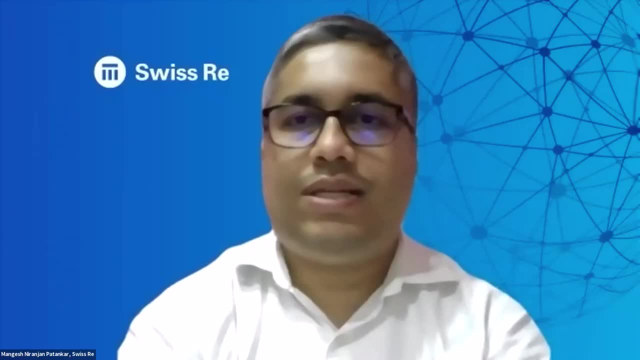 please thanks. thanks, uh, dr sikka, for this opportunity. uh also thanks to iwmi uh for allowing me to share the thoughts on this very important uh project. i think the product uh we're with iwmi, which we implemented in india and bangladesh, then the simple uh index formula, but 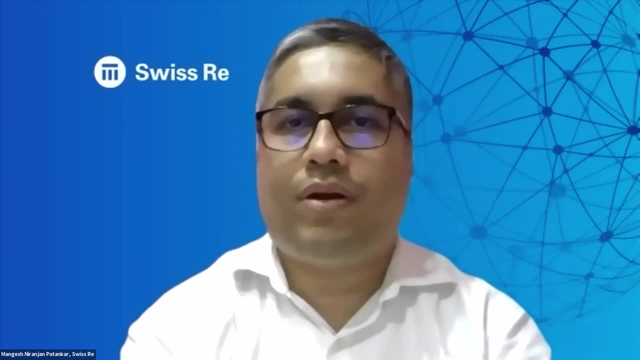 at the same time, the indices were actually derived from various data sets and the overall methodology remained quite complex. so, as you said, this is really a high-tech project. there are tremendous opportunities to extend flood index insurance in more territories, because there is a genuine protection gap in the flood risk sector and that's not only confined to, you know, the farming communities or 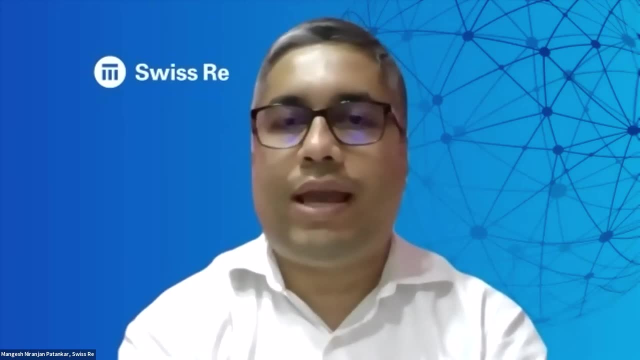 only governments, but it's actually applicable to every agri-allied institution and even general public, like you and me. uh, there are bound to be some risks which cannot be absorbed or mitigated and risk transfer through commercial insurance, uh mechanism. uh could be the only way and experience. 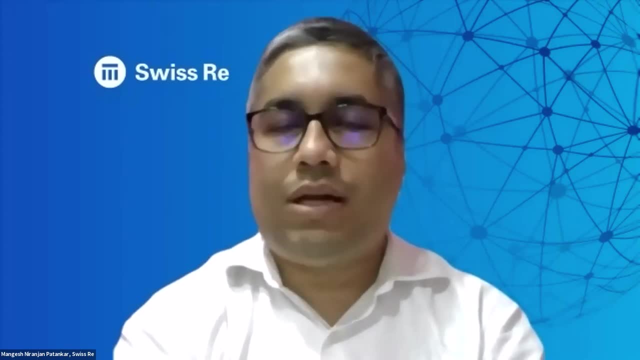 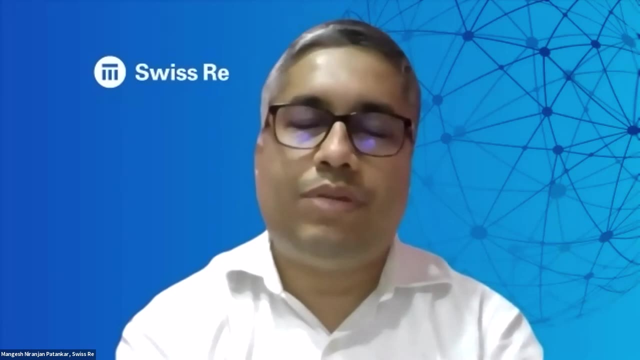 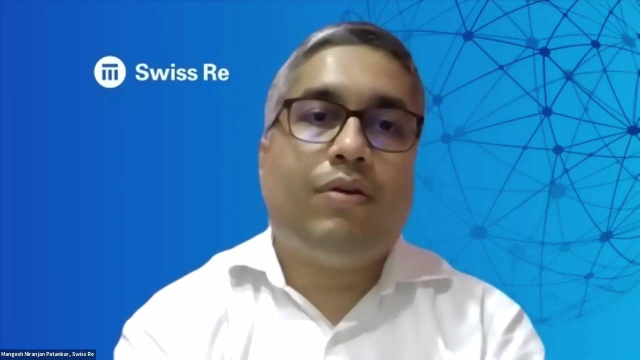 flood risk is definitely one of them. uh. now, as far as opportunities are concerned, uh, first of all, second based data data sets can actually help us in providing information on floods or excess of rain or excess soil moisture. we have actually a few successful examples already in china. 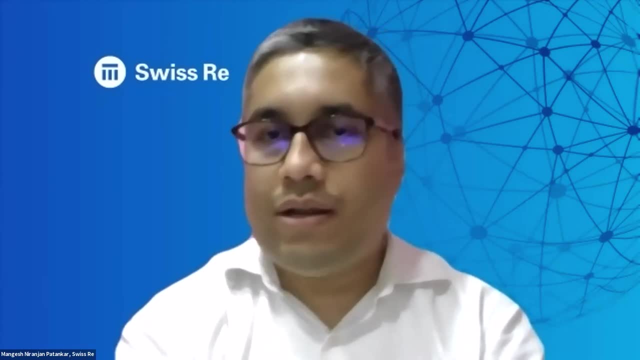 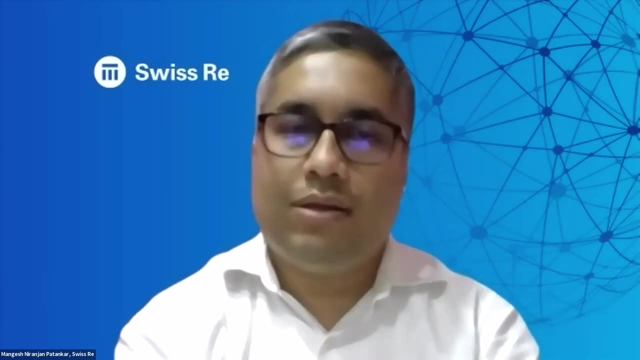 where the provincial governments bought flood index products, along with droughts and cyclones, of course. the project with IWMI is another successful pilot. We have some excess of soil, moisture products as well, running with providers like Vandercat, but those are usually, you know, given. 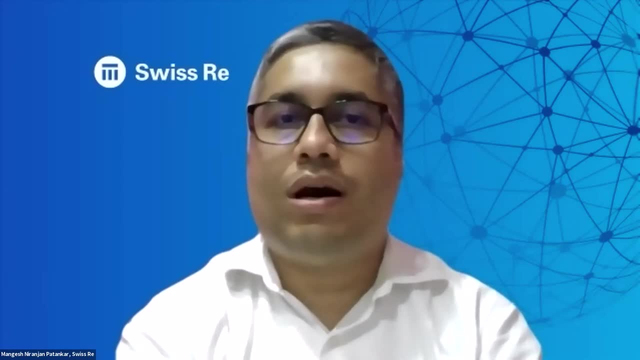 as sort of add-on products along with the trot product. Now, as far as challenges are concerned, first of all, establishing a correlation with the flood, between the, between the flood and the crop yield loss. It's always quite difficult, as compared to you know, establishing a correlation. 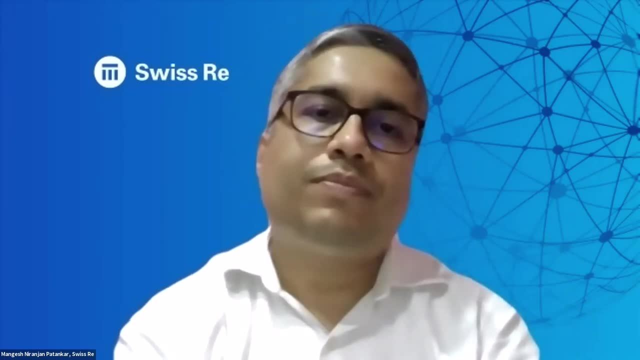 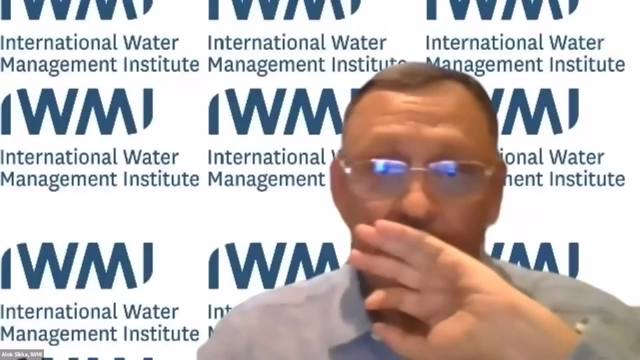 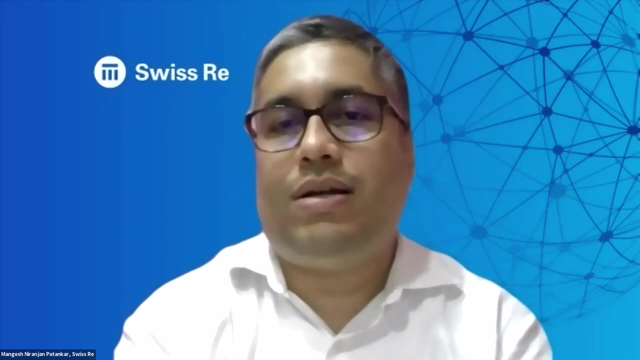 between trot and the crop yields. This remains a concern when we want to give a product for excess water sensitive crops like soybean. Apart from this, I think not on every level of flood risk can be, or needs to be, ensured And there could be a few other strategies to manage such risks, and I think this is fairly. 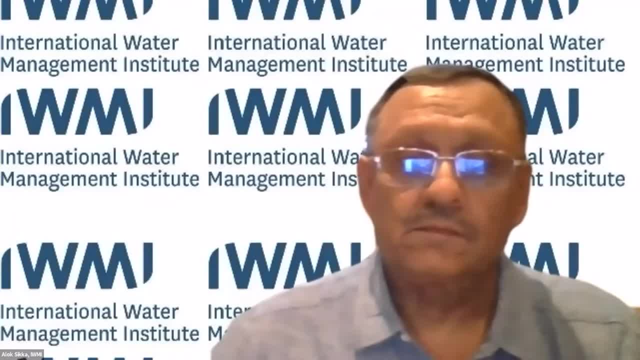 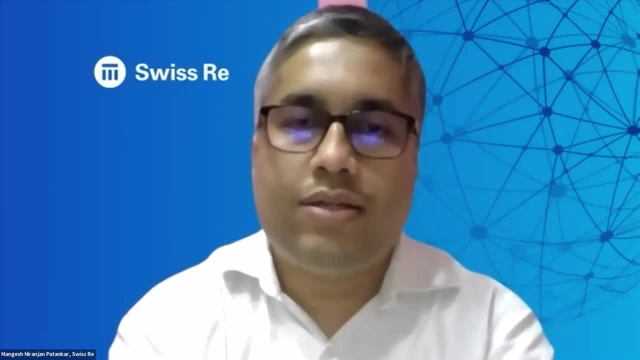 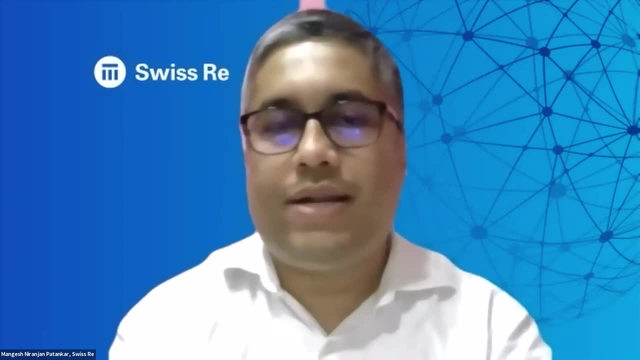 relevant with the earlier presentations which were made here, But I'm sure that we can create actually comprehensive risk management product for agrarian communities by combining the flood index concept with other types of indices And I have a strong belief that, as long as we develop. 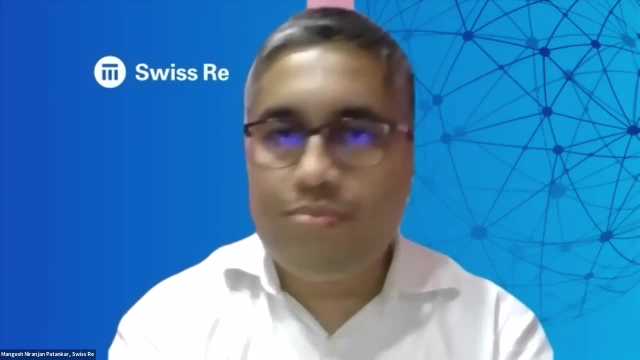 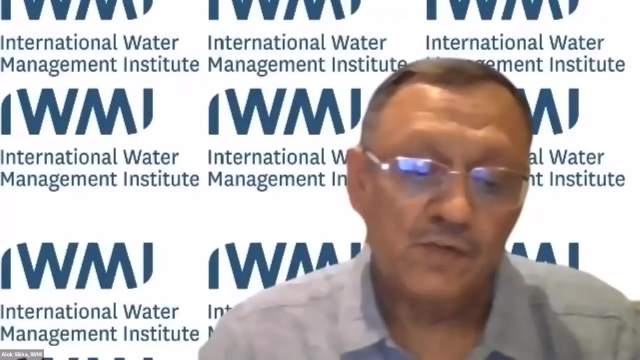 something which is relevant for the farmers, objective and scalable, easy to understand. it should be successful, Thank you. Thank you very much, Mangesh, for giving a very precise overview of everything what's happening. And now the final panelist here is again, with whom we are working: Anuj. 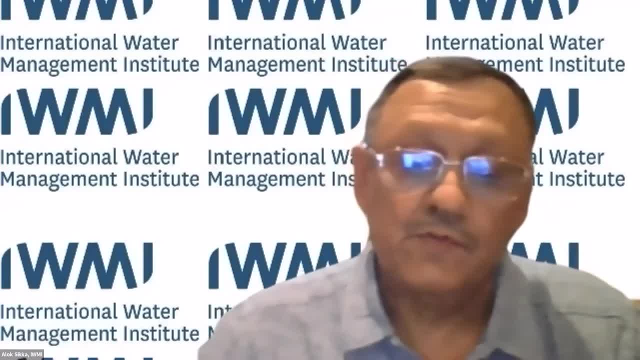 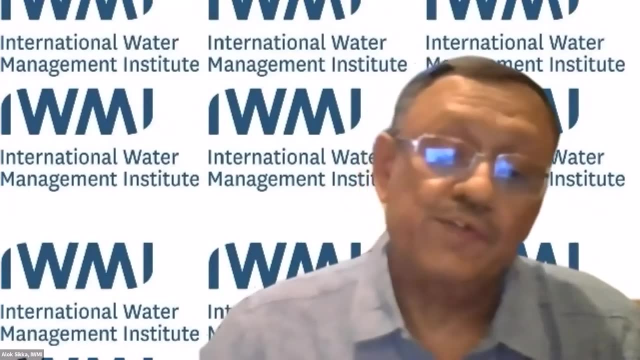 Kambat, who is the CEO of WRMS Private Limited in India, And Anuj, you are promoting the integrated risk management approach, as you know, that we all know, And how do you see the potential of bundled insurance solutions being jointly implemented by WLE, IME and WRMS? And 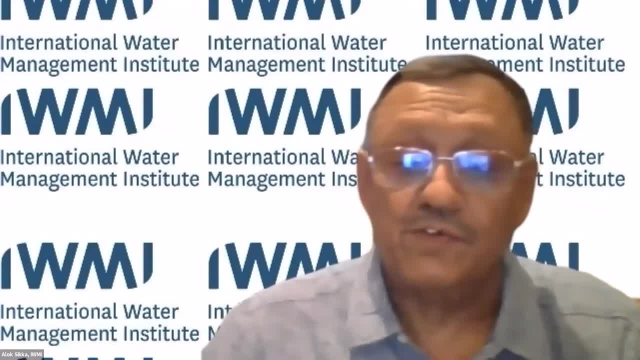 could you summarize the buying-in of such solutions among farmers and especially also the value chain partners for scaling and sustainability? And, as you know, we have a lot of questions in the Q&A because scaling and sustainability is really very, very important in the agenda. 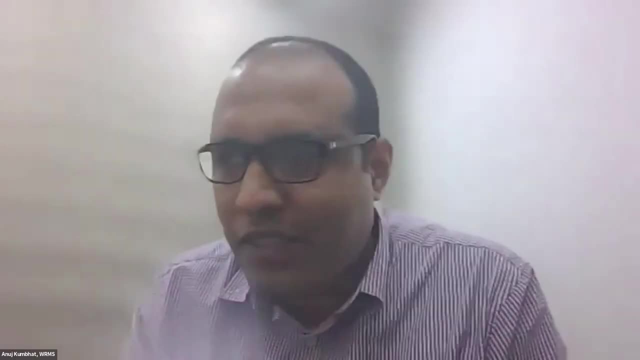 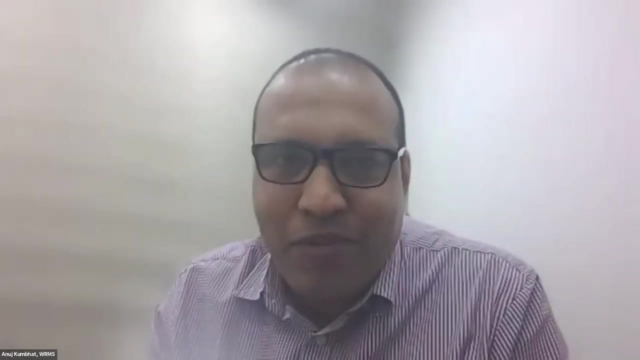 So over to you, Anuj, Thank you. Thank you, Dr Sikka. I hope I'm audible. Sure, sure, Pretty much. Yes, Thanks a lot. And yeah, we've been working with IME and Dr Giriraj in implementing the. 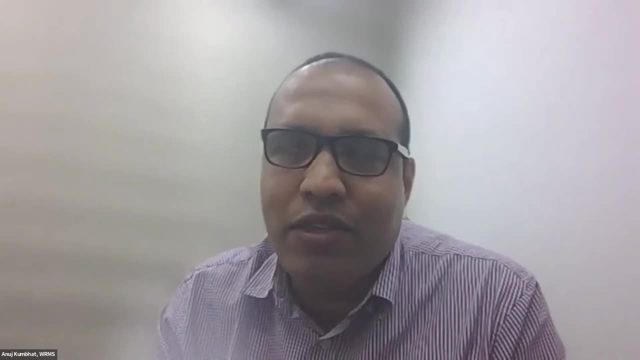 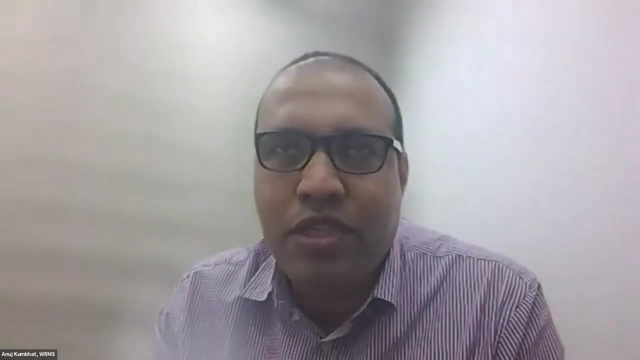 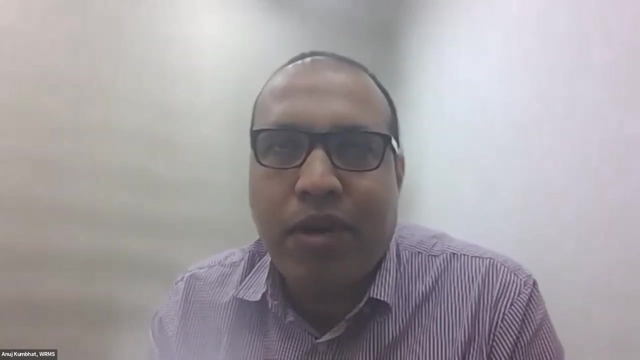 bundled solutions And primarily when Dr Giriraj talked about the solution where the risk reduction, risk transfer and post even reduction of the bundled solutions. So we're very excited to see how the solution can be bundled together and offered as a solution to the farmers. We were very excited to participate as this has been also our agenda in terms. 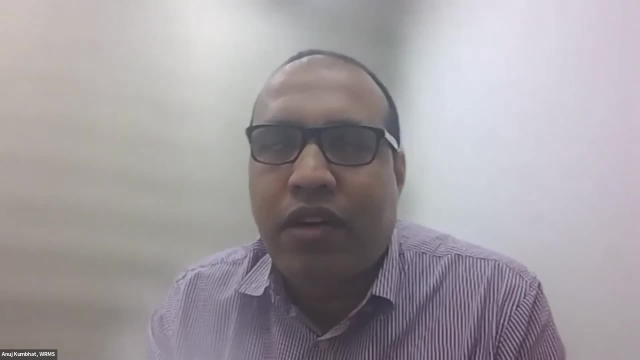 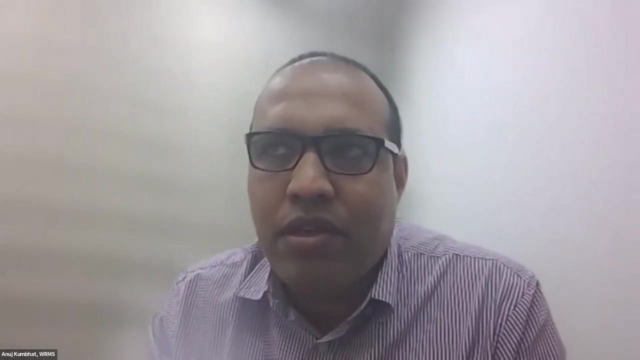 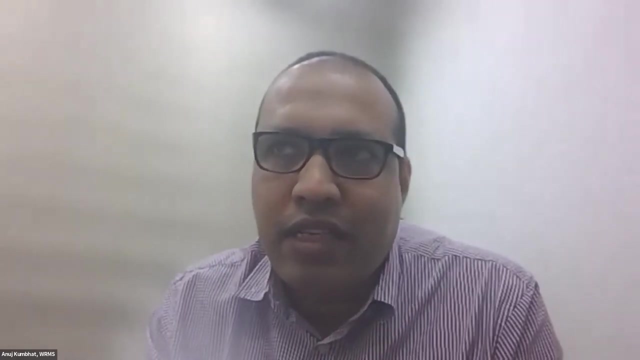 of offering the risk management solutions to the farmer in a more holistic way, And what we realize is that the uptake among the farmer is much higher because it is more involved risk management approach, where we are talking about first working on offering them the varieties which otherwise wouldn't be possible, And then we are also working on offering them. 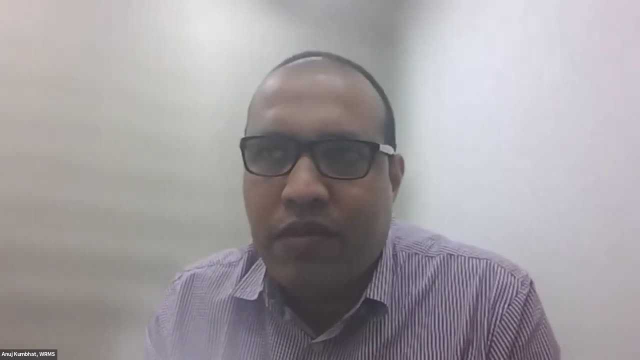 the seed systems. So we again, if you know is not working, then you're happy to talk about. but if you also want to look at the 1970s and 1980s as well, you can do it directly. 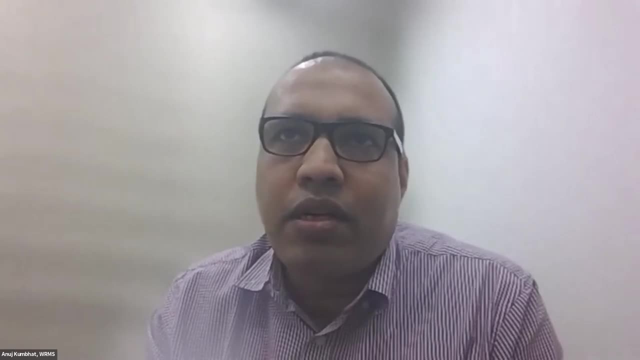 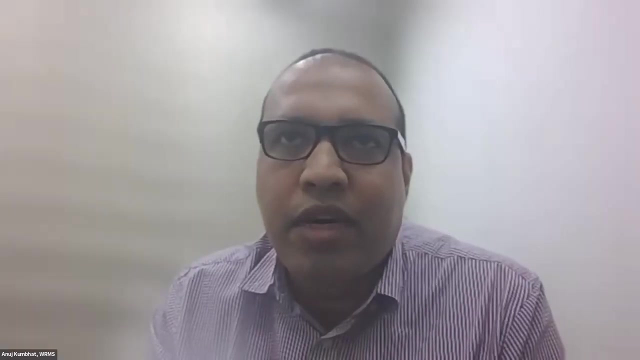 for your customers. So they may hesitate to buy because of the risks involved, But those varieties probably would help them in managing those risk per se. So insurance bundling insurance with such seed systems helps in resolving this dilemma in the minds of the farmer. that if 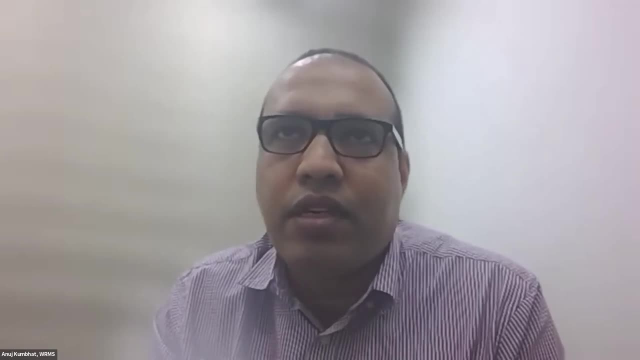 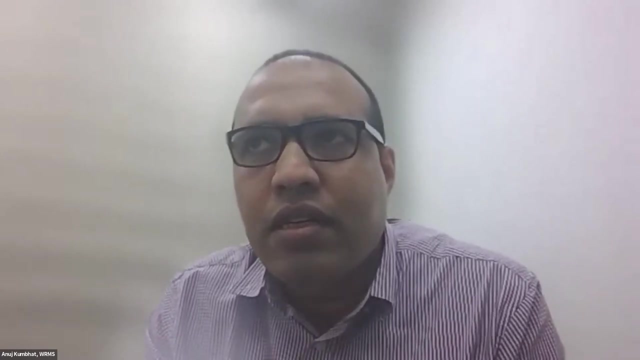 they're investing in new technology, are they covering themselves for the downside risk of it? The other thing, which obviously also most farmers won't, is that once they're operating, uh, the seeds are provided, are they also? they also need advisories or support in terms of how, when. 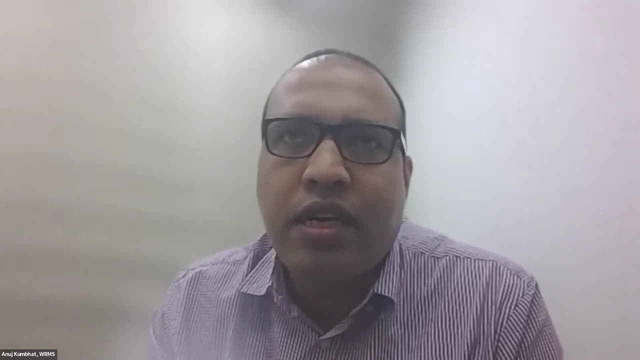 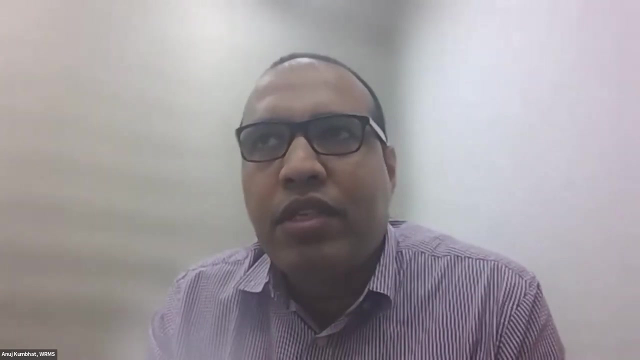 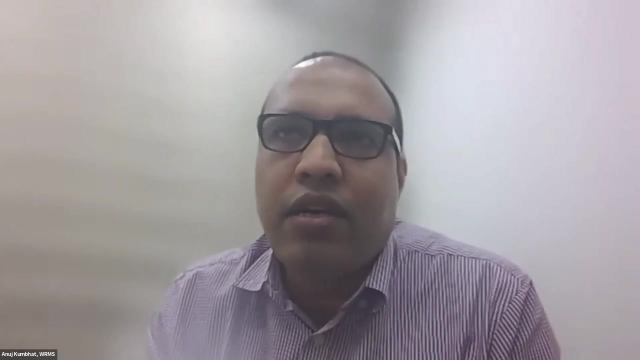 and what to do with the crop, and with more holistic, climate-based uh advisories which we provide to the farmers in this big star project. uh, we have been able to tell farmer, uh what is the ideal time to irrigate, when not to irrigate, when to apply pesticides, and all these things were. 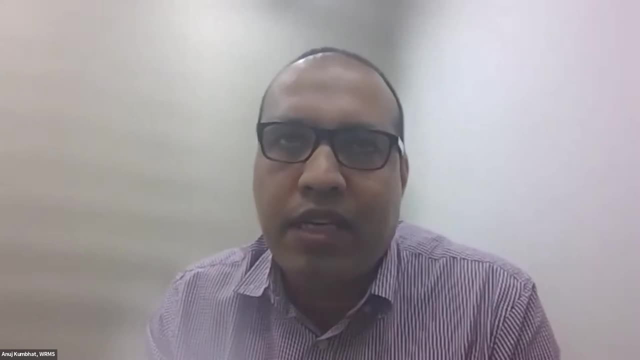 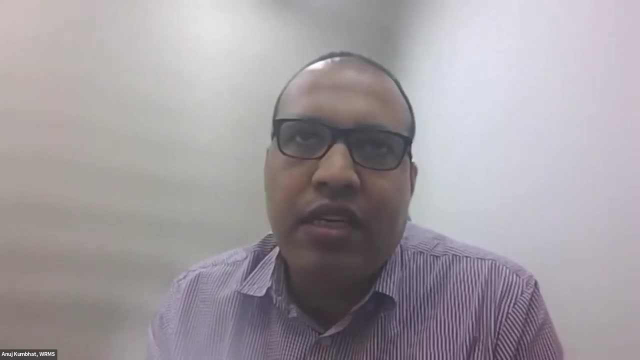 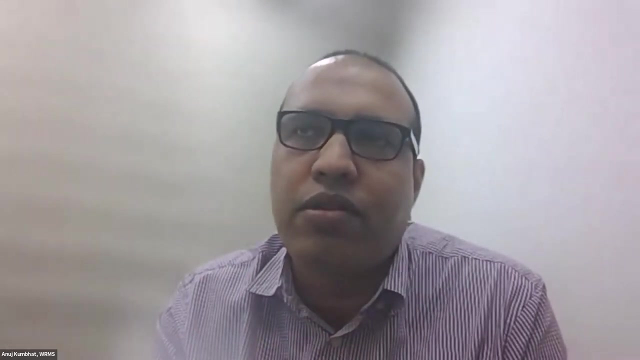 offered to the farmer on a platform or sms or or an application which was offered to them. so basically, it's a more holistic risk management approach and, interestingly, uh, we see that there is an uptick about uh for this approach, not just in uh among the farmers, but also the value chain. 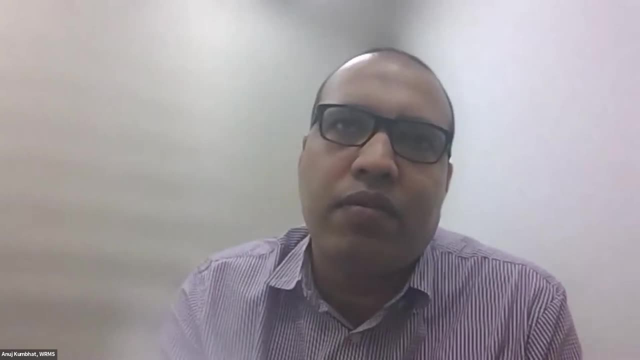 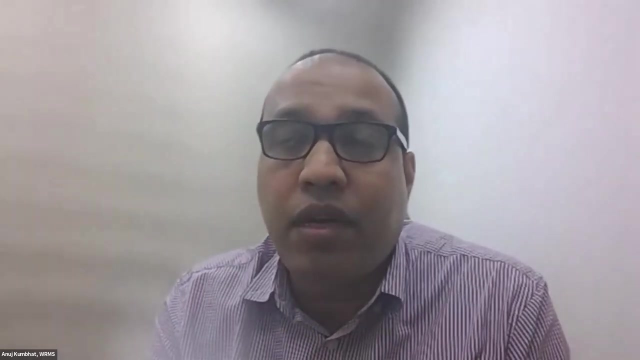 players, uh like the credit providers. we're now working with some of the credit providers who want to offer some similar solutions uh to the farmers and uh a large part of the seed production systems or cta systems, so new varieties which are coming in the market and a lot of private. 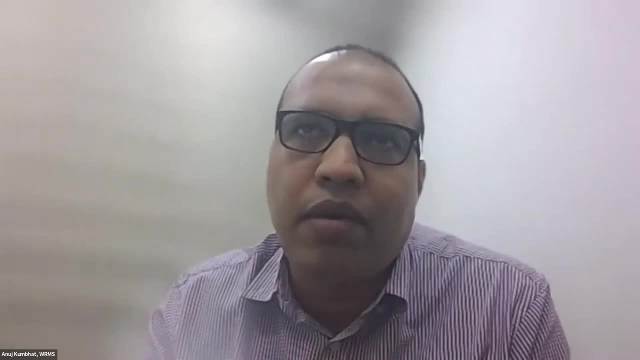 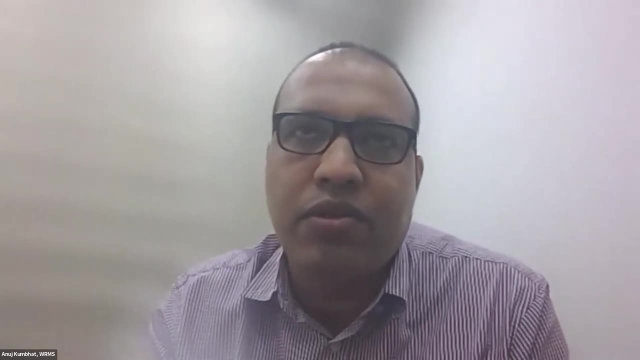 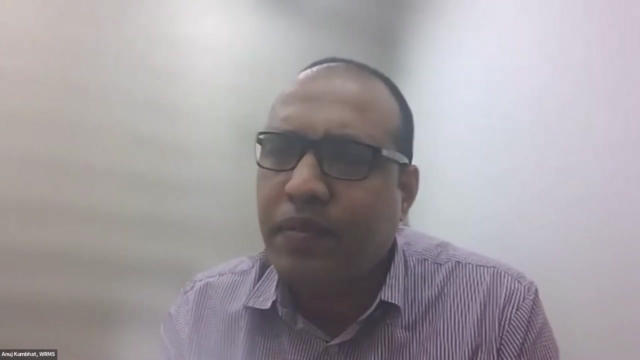 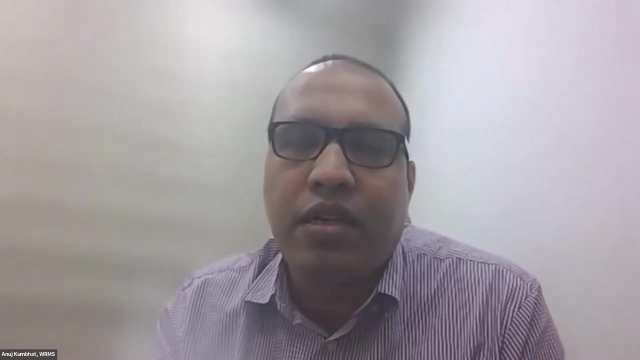 sector. uh seed companies are interested in bundling the risk management solutions so that farmers understand the benefit and they are able to invest in those new solutions without hesitating about the uh losing the crop or risks related to that. so i see this opportunity in almost all uh crop areas where the risk is high and where uh uh the risk management approach can. 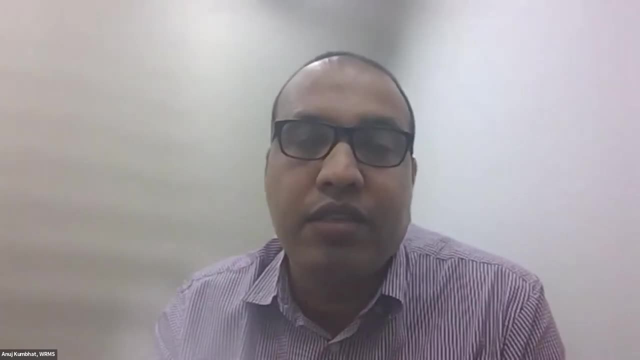 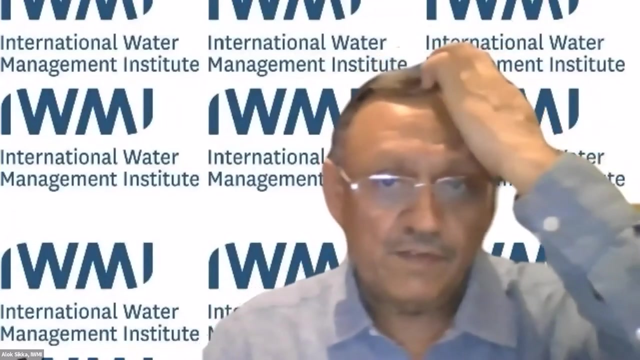 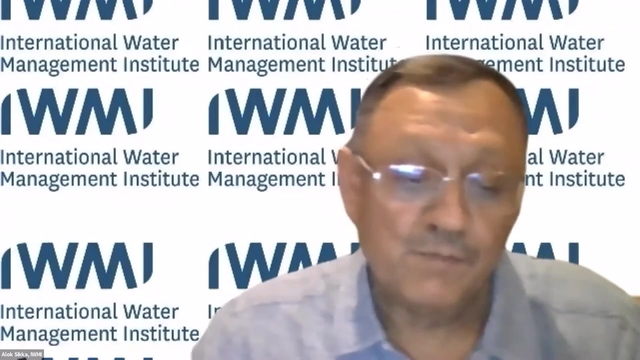 lead to better input, uh uh, utilization by the farmers. okay, thank you. thank you very much. so now i see a couple of questions, so i think. so first of all, i thank all of you panelists. please be with us because there are a couple of questions, so i'll i'll, i'll be just 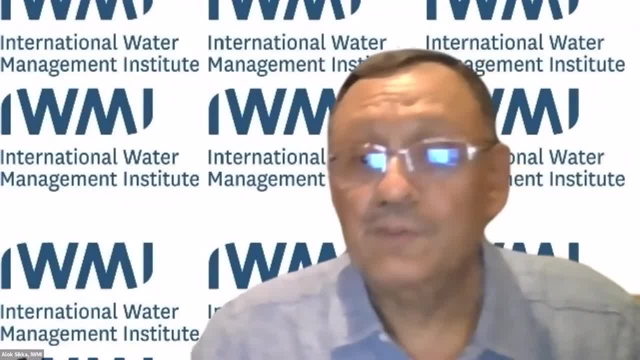 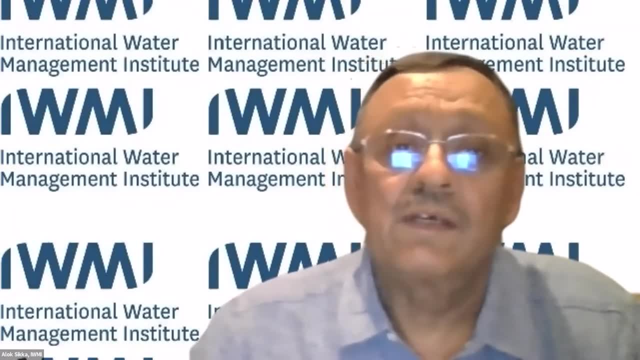 coming back to you- and the first i come to- i guess manges is a question in the q a about this- is the extreme precipitation is notoriously difficult. as we know, it's very difficult to predict. can the participants comment on the predictive capacity of the flood indices? for what time? 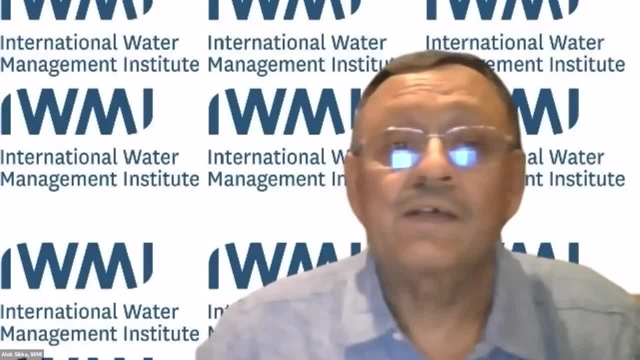 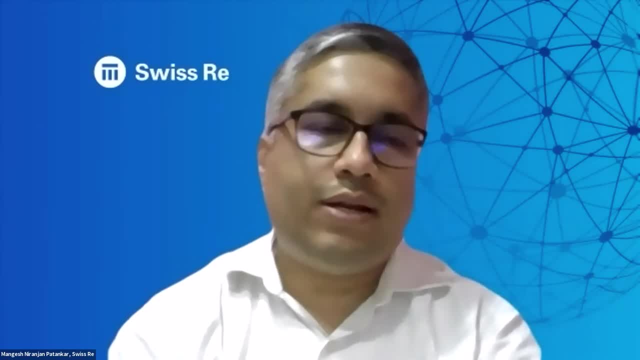 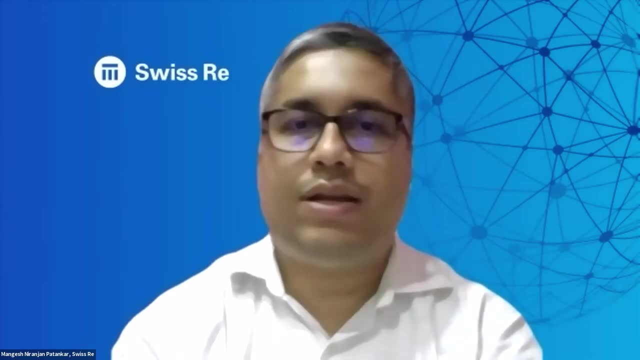 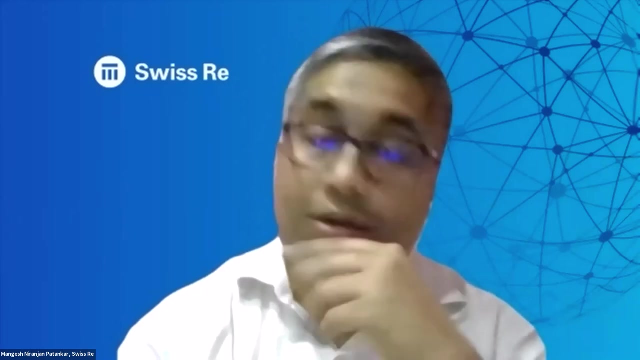 periods. can we get reliable flood prediction in the cases covered over here? yeah, happy to answer. indeed, i think accurate prediction of extreme events remains a bit elusive target so far. however, the flood index insurance product that we have designed here focuses not on the prediction, future prediction event rather than the measurement. rather than that, it 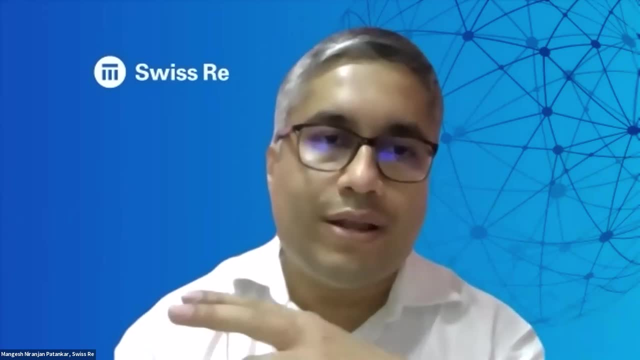 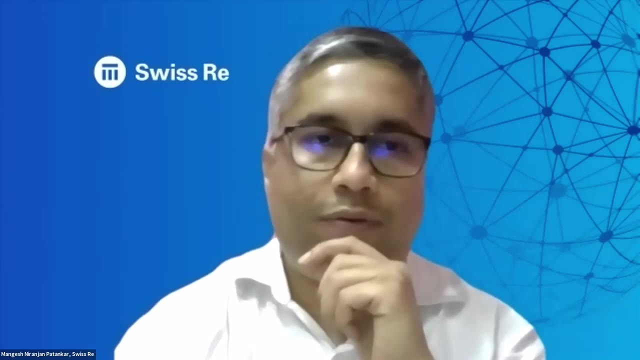 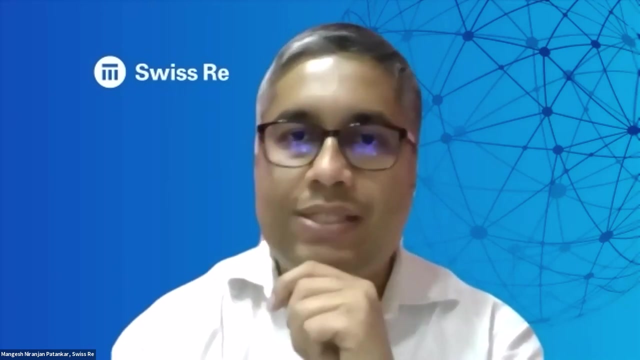 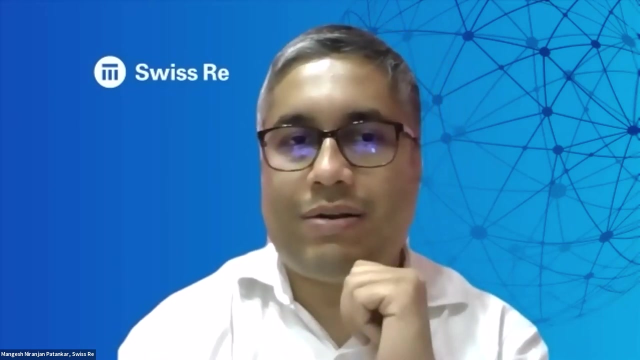 focuses on the measurement of actual flood event that has occurred. so so i i believe the question here is: is you know uh fairly i would say relevant uh to to the flood prediction, uh related topics, whereas as far as the ibfi project is concerned, that that uh uh particular project? 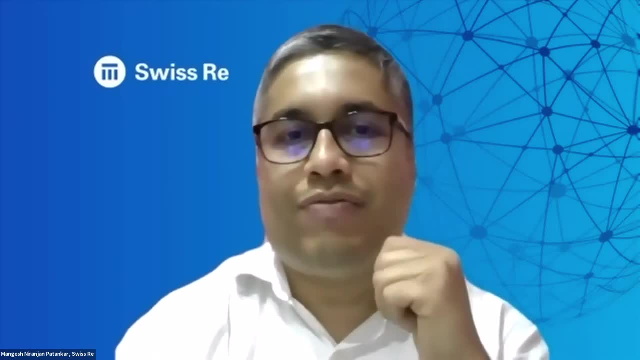 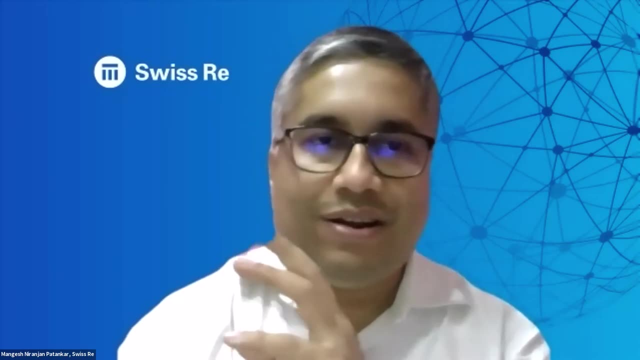 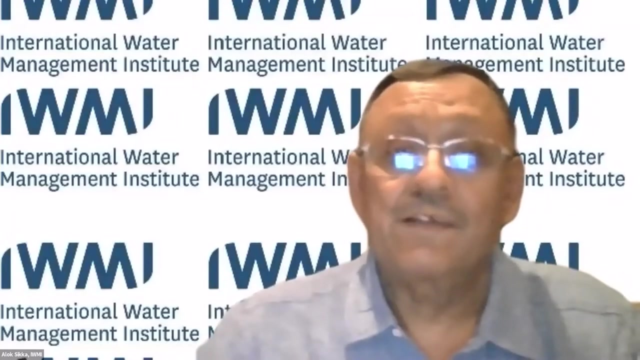 relied on uh creating indices for the measurement of actual uh flood event. that has already uh. okay, sd相 Undertak ait answer in the current context i would say yeah, i do agree with you. i mean, of course, they are not really very straightforward answer to that question, because for what time? but definitely i mean so. 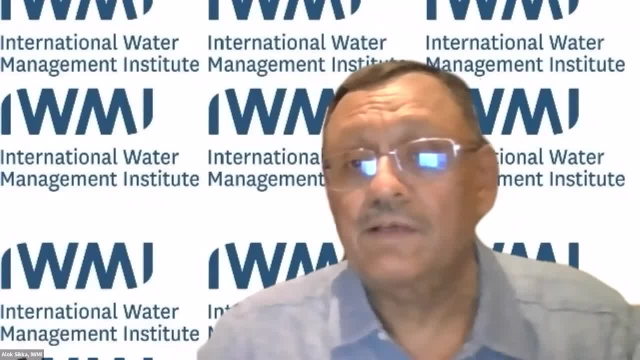 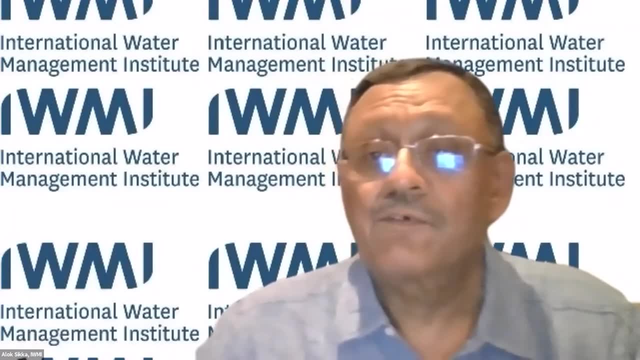 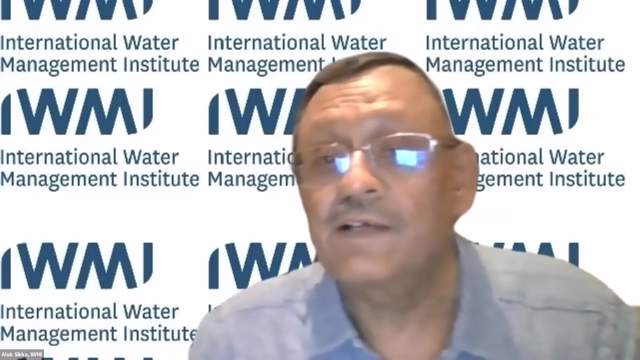 the next question. i mean there is somebody has asked: uh, delphi has asked shirish if you could share some satellite images for her for the project, but i think the person is there in the chat and you can just perhaps i do not know which particular research project area the person is. 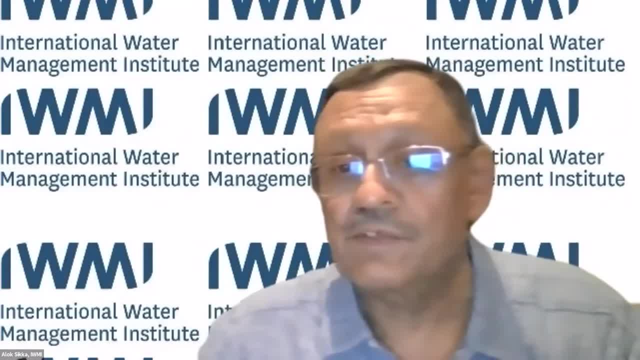 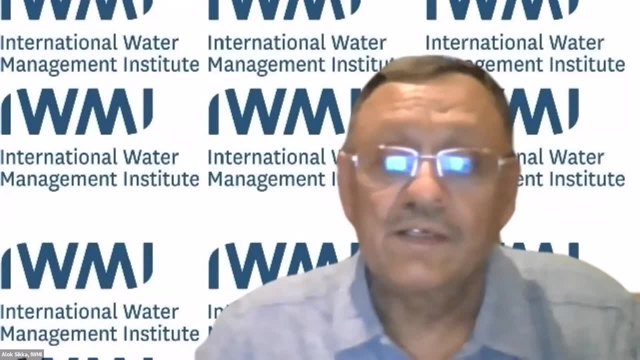 talking about. so, anyway, you can chat with the person on the this thing. the other one, uh, is a question for enamor uh, and this is a question from one of the indian icr scientists, vamanan, that if he would like to know whether ibfi has been accepted. 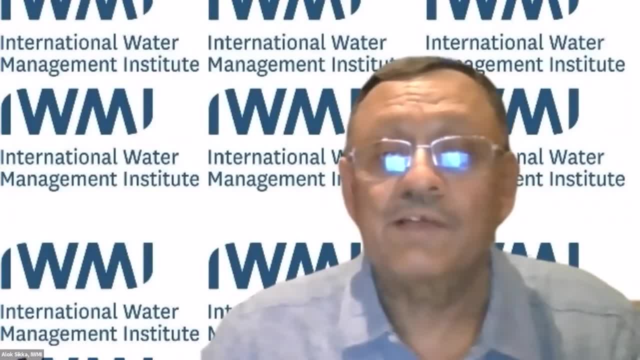 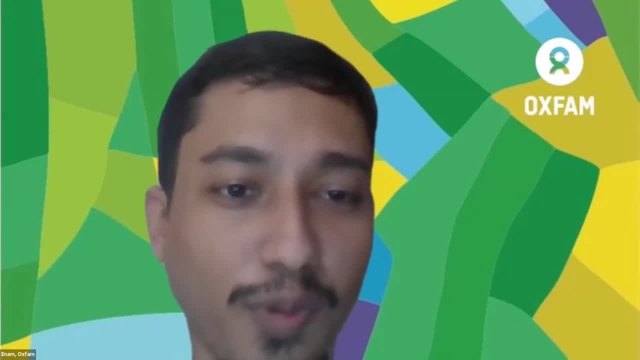 at national crop insurance policy in bangladesh? thank you for the question. we don't really have a crop insurance policy, but there is policy framework for insurances and there is agricultural policy. so none of them specifically mentions index based insurances. but it is legal, it is legally accepted, which is why we could. 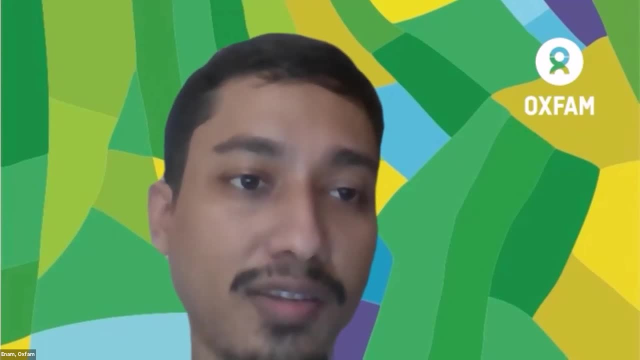 implement. however, we are trying to bring some changes in the policy scale. for instance, uh, people who need this access are close to the microfinance institutions and mobile money transfer platforms rather than banks, so some of the insurance regulations are really like requiring people to use the banks, which is a challenge. this is just an example, so we are trying to change that. 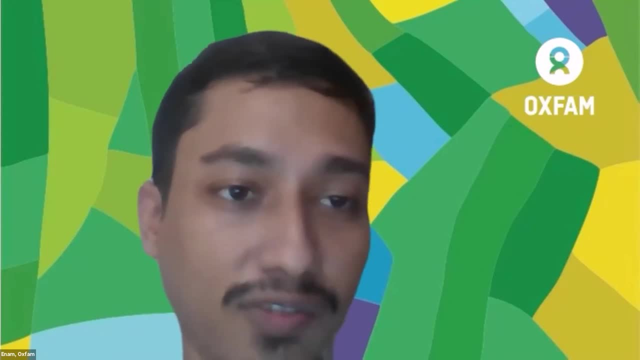 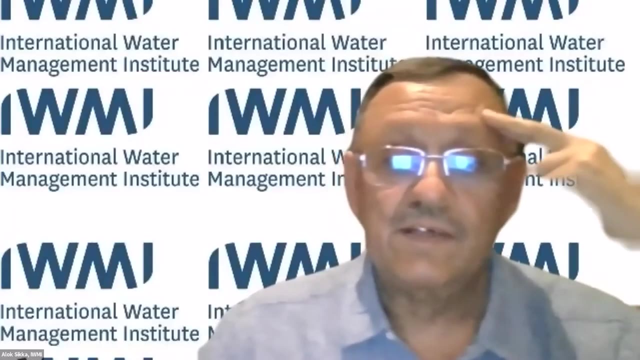 so, with context, i think our insurance policy will be more inclusive of index-based insurances. but it's not illegal, all right. so now i see a question in the q a box from eric and he thanks especially mangesh for your answer. but he feels that a key focus on the 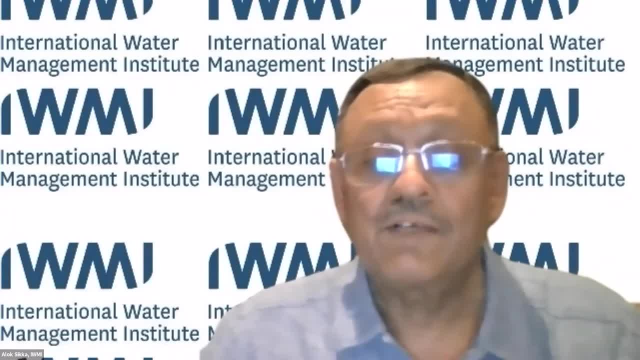 flood risk reduction should be on flood prevention and not on disaster management. so i leave it to any panelists, to, or the key speakers, those who are there, giriraj and adulu- to take up that question. if you can, anyone can, or if no one, or if you guys want me to answer, i'll do that, but let's let me. 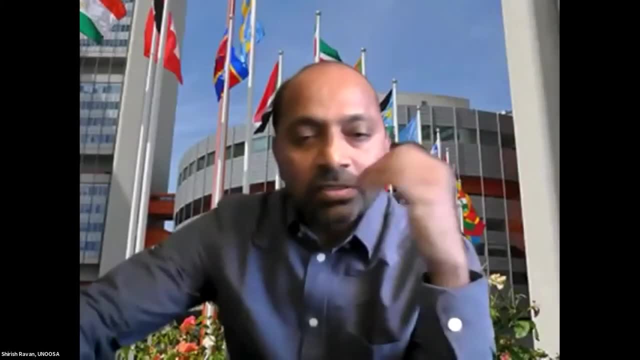 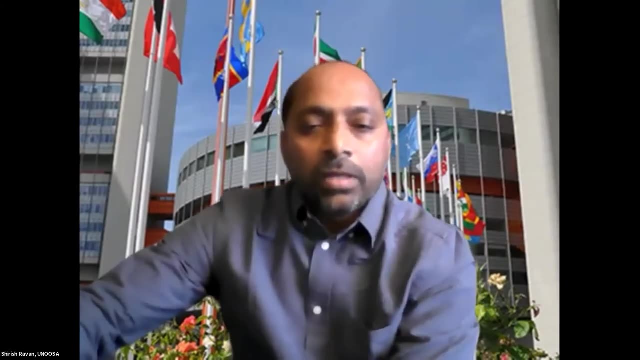 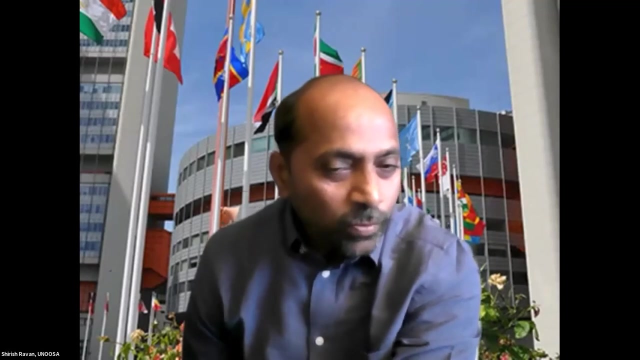 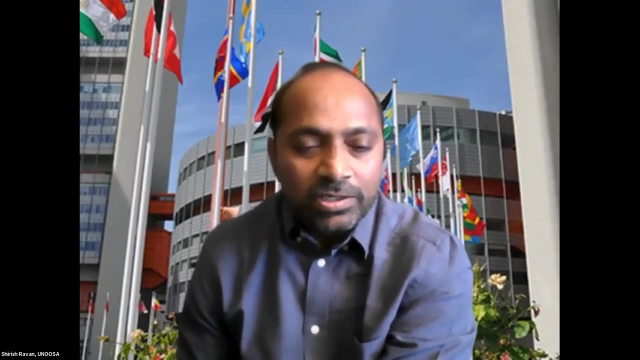 first come back to come to all of you. i can. i can answer, sure, okay, so uh, he's right away that if you see uh look at the global frameworks, also yoga framework- recognize that the should not be on the disaster management per se, but it should be more on the building resilience. 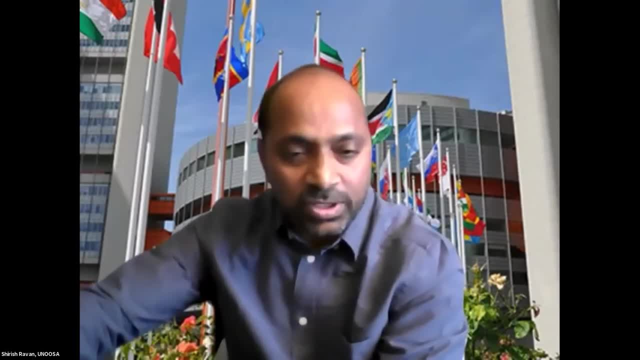 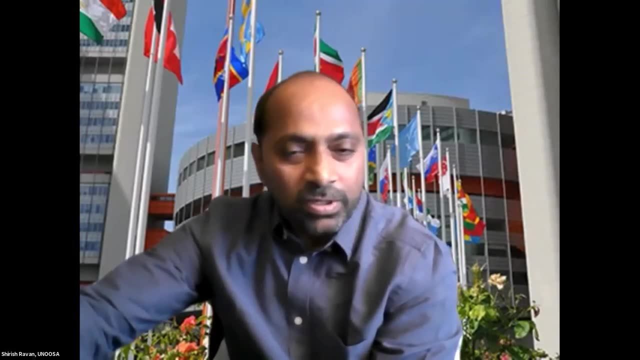 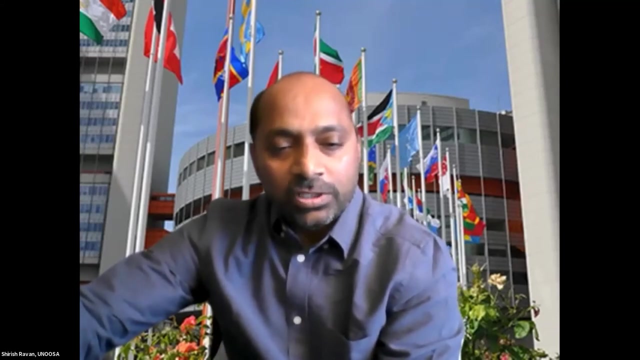 and, you know, avoiding the new generation of new risks. so that is what is more important and i think, with uh existence of sendai framework from 2015, more and more countries are aware that it is very important to really not just focus on the disaster management but to 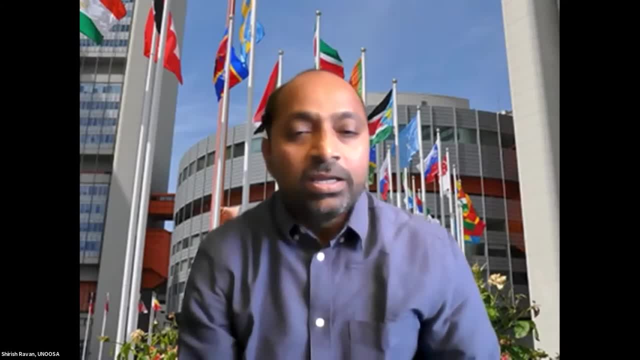 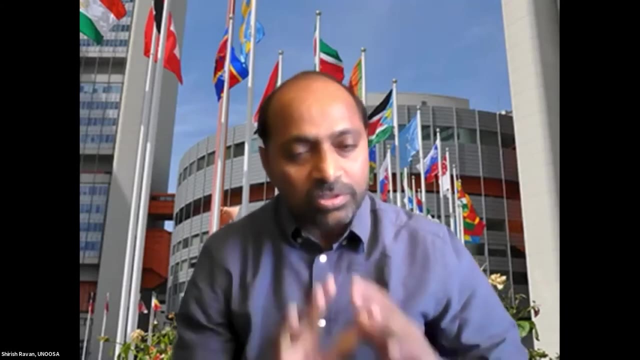 build the flood resilience or, for that matter, resilience for any disaster. uh so, uh, whatever work that we are doing together- i mean iwmi and un spider are partners, and we have 26 such regional support offices all over the continents- the main emphasis is, uh, advocating on building resilience, or use the tools, not only the space-based tools, but any tools that are. 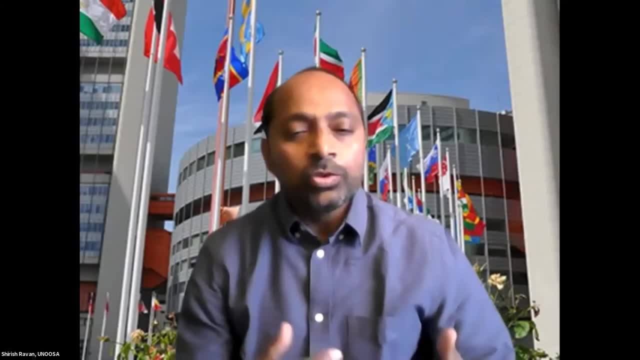 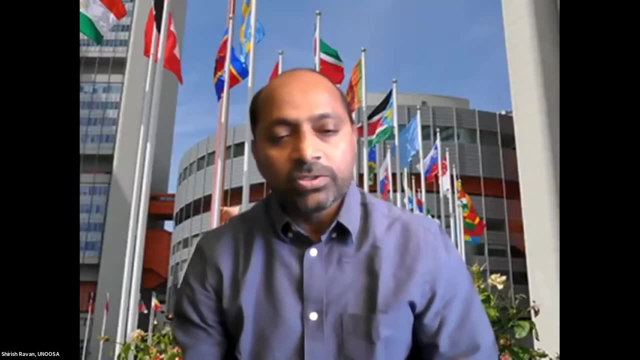 developed for addressing uh floors or any other disasters. use them on regular basis to build the resilience. and if you are using that very, very effectively on regular basis, you can use it if a during actual uh when the disaster happens. so that has been uh the advocacy and efforts of uh. 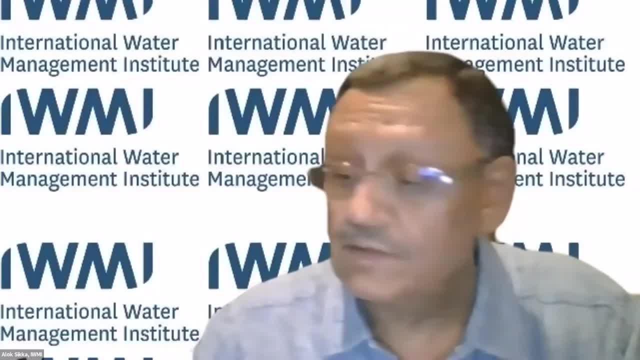 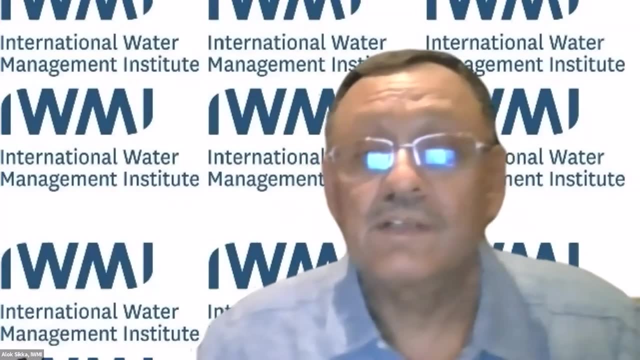 thank you, siris. thank you, siris. yes, i think this is the way because, ultimately, our objective is to build the resilience of the system to try and cope with that, and which also requires to be really looked into, because, you know, if somebody says prevention, prevention of course, perhaps on the 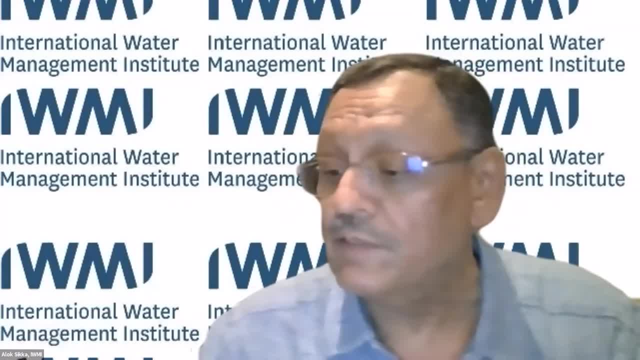 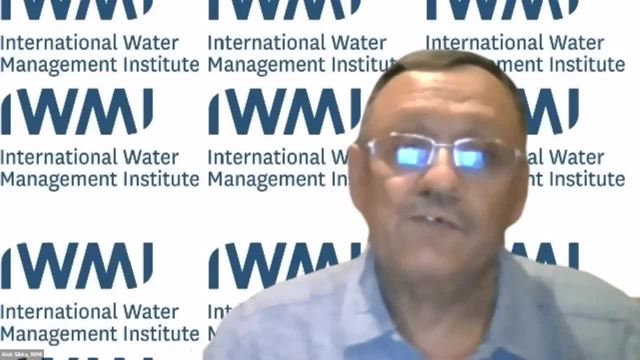 front kind of things nobody can really say. but we can always say: build the resilience and also the preparedness strategy, because the preparedness would also lead to enhanced resilience. so that's the kind of the essence of thing when we are working into any kind of a water. 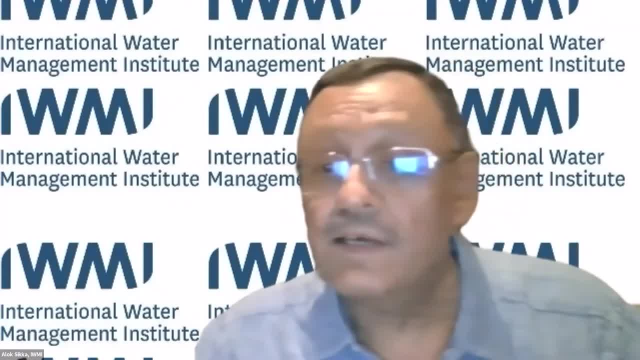 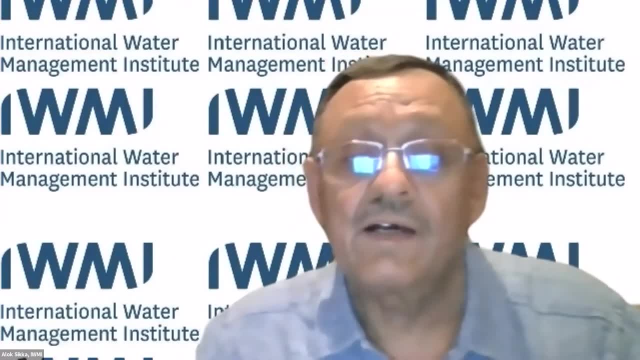 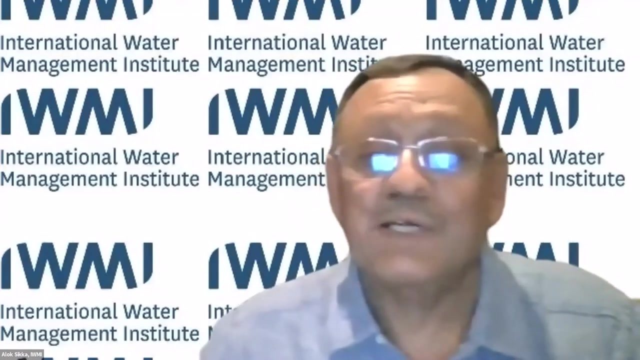 related risk. so i am left with three more minutes for this particular session and i see, uh, another question. good presentation, please. how do you conserve water for agriculture purposes in a flood prone community? so any speaker or the panelist would you like to take that please? how do you conserve water for? 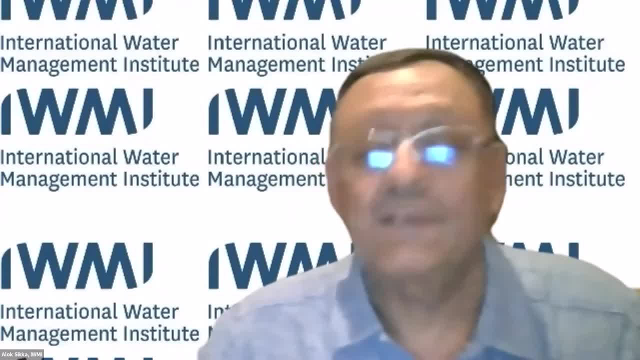 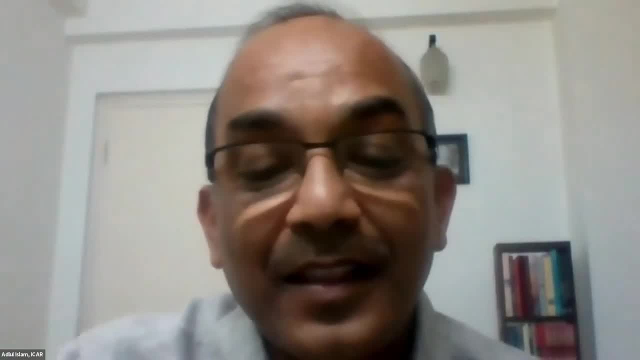 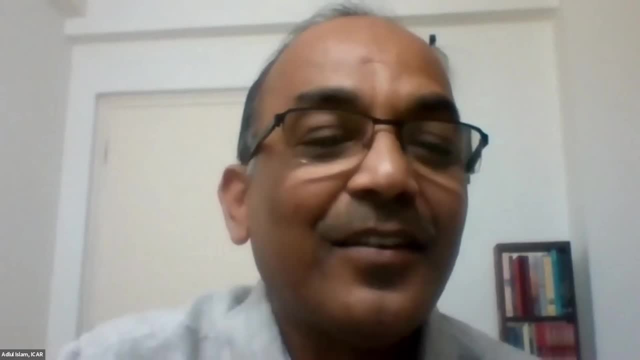 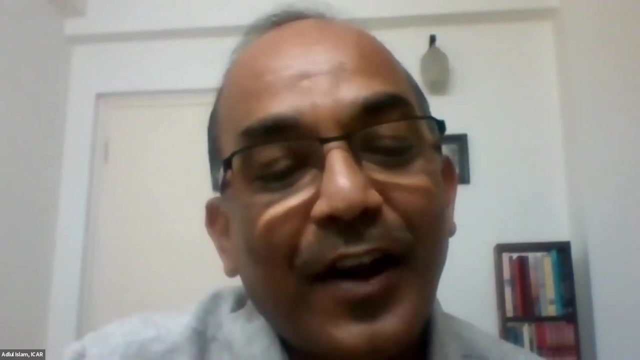 agriculture purposes in a flood prone community. yes, sir, in the platform area, the one of the options we say that, uh, you mean i share as well- that is the water that is used to purify where the water- flood water- is diverted for groundwater recharge and that water is used during lean create for irrigation purpose. so that is one of the option. 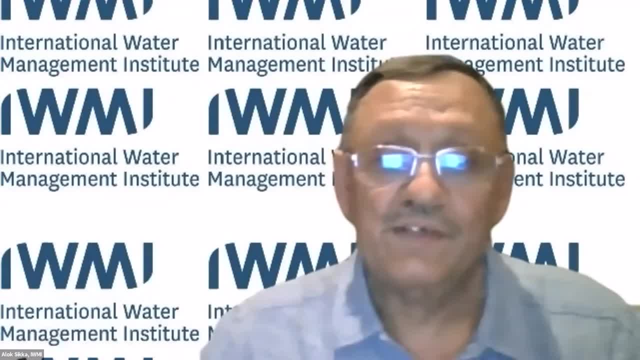 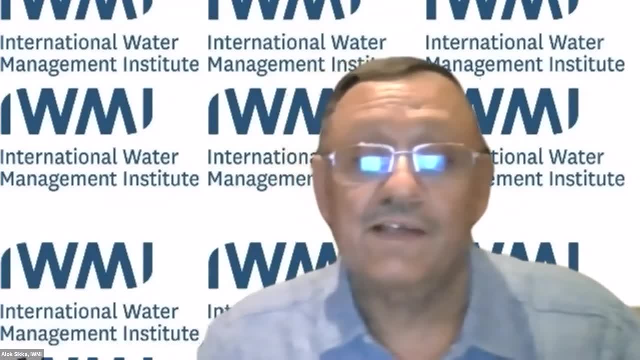 yes, thank you. yeah, so that's there, and the manager i keep for each, that's also a kind of a manager. i keep a recharge system, so we are working. so yes, so thanks, thank you very much for that, and i see again questions pouring in, so, but i have got another two minutes left, i guess. so 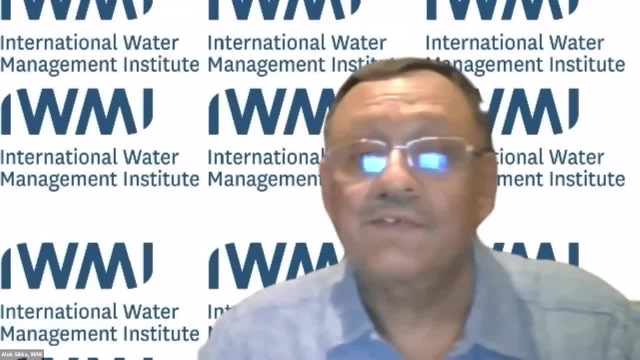 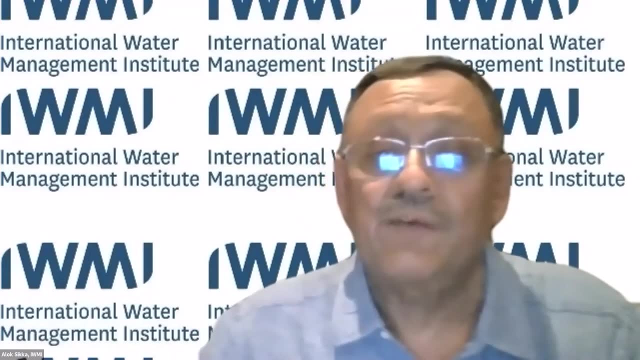 the uptake by farmers and our efficiency of approach comparable. would it be faulty, since each strategy this is a different part of so and uh. so i don't say. i mean somebody is asking what the uptake of the farmers and the efficiency of approach, how they are comparable and how. 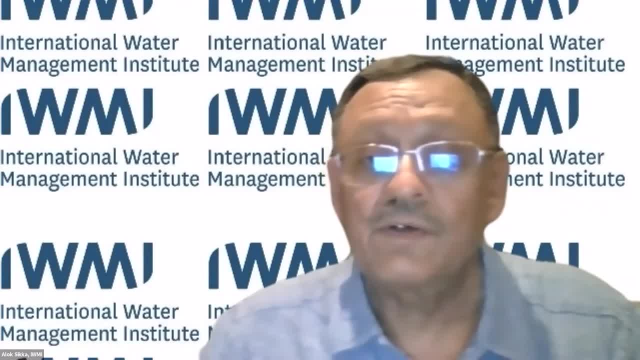 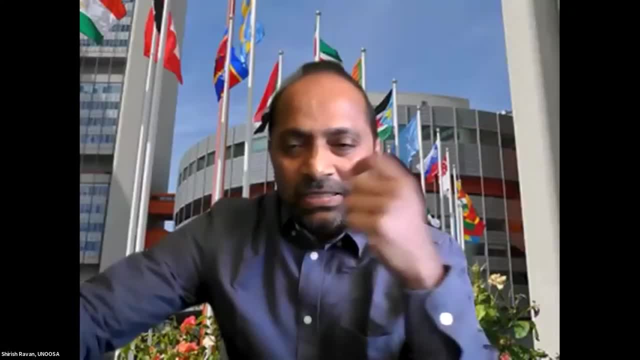 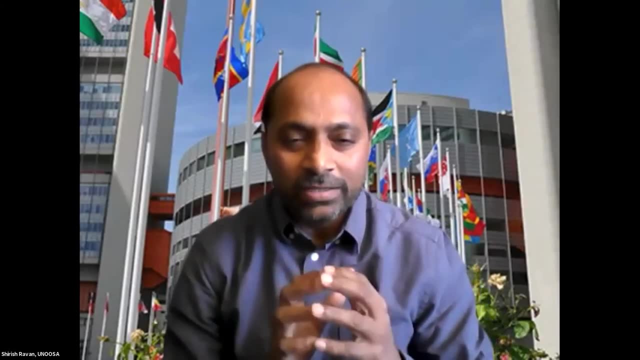 they are going to be looking into, so i do not know if anybody would like to take on that and how much time is there. I can just briefly say something about this now. See, farmers are very important players in the food security, And I think everyone is aware of the Food System Summit which has been launched on 23rd September. 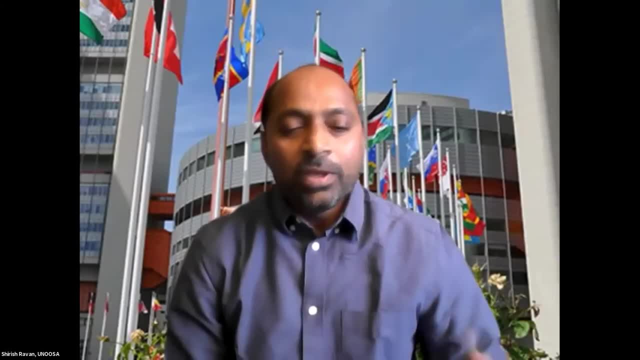 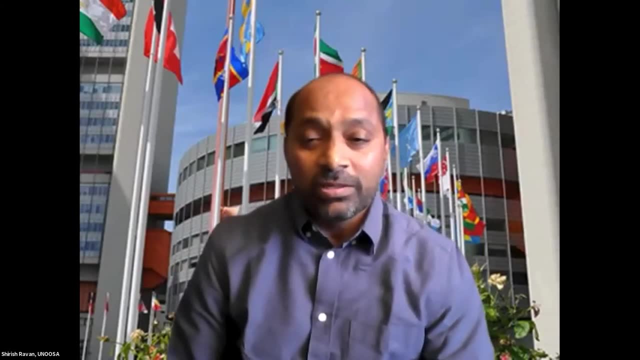 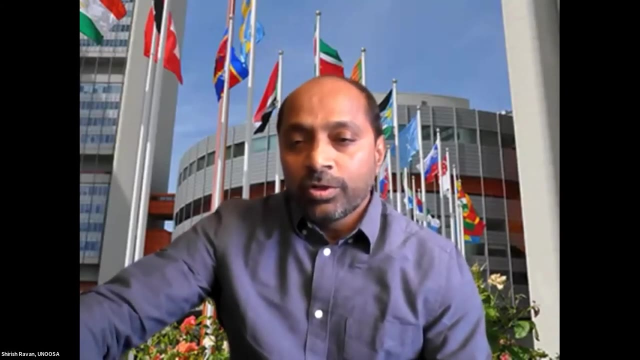 which is the beginning of the way we produce, transform produce, consume waste or even store the food, And I think farmers are one of the biggest stakeholders in building resilient food systems, And that is where I see it is now the time where really this farming community will be involved in a lot of those aspects related to risk management. 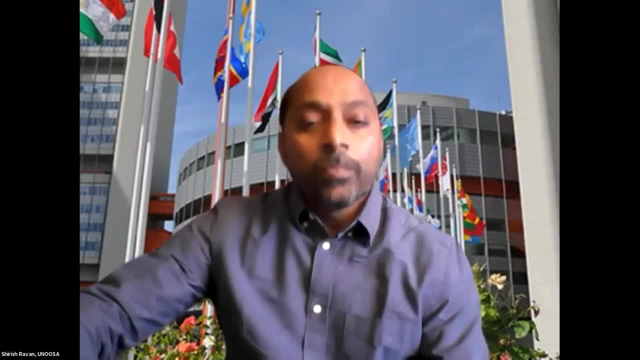 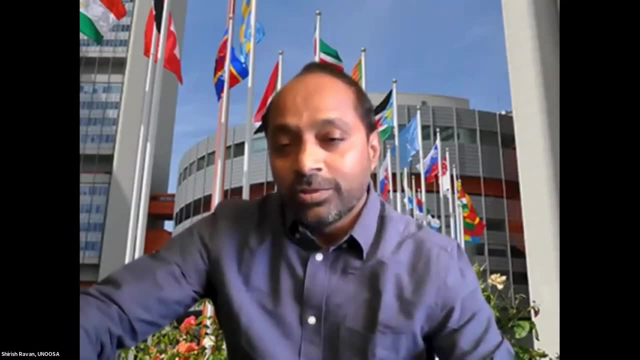 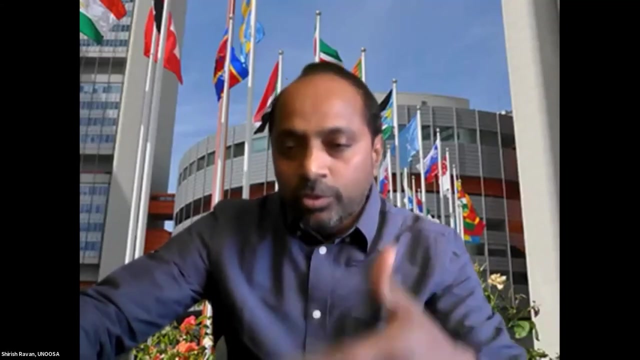 because any risk to the agriculture is the risk to the food systems, And food system is a very significant initiative to advance on the sustainable development goals. So I think this will be a new focus and a lot of strategic inputs will happen now, basically involving the farming community into this panel. 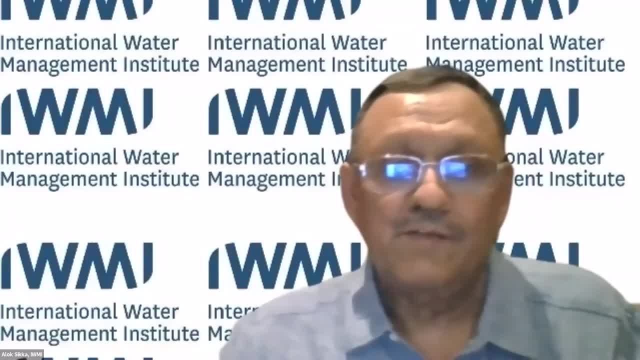 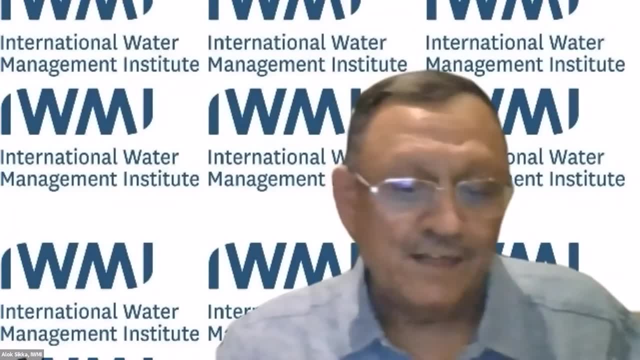 So thank you, Sirish, and thanks to all the panel members and the speakers, And now over to Alex or other organizers for the last point on the agenda on the closing remarks. So over to you guys, And thank you all very much. 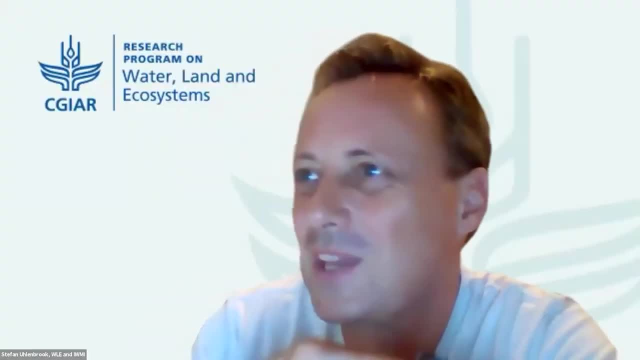 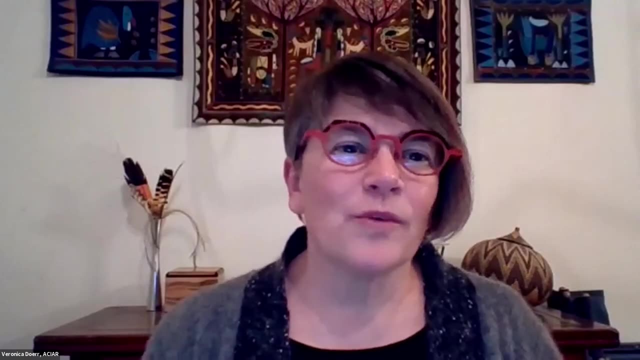 It is now Dr Veronica Dürr Over. Thank you, Thank you, Stephan. Thank you so much to all the speakers. Hello everyone. So I'm the research program manager for climate change at the Australian Center for International Agricultural Research. 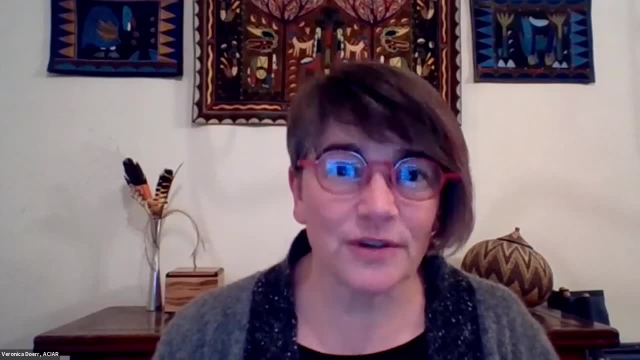 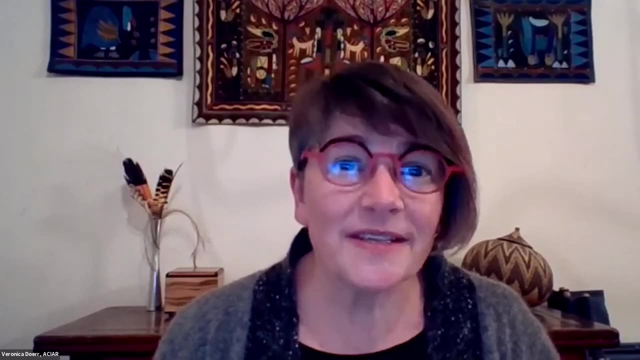 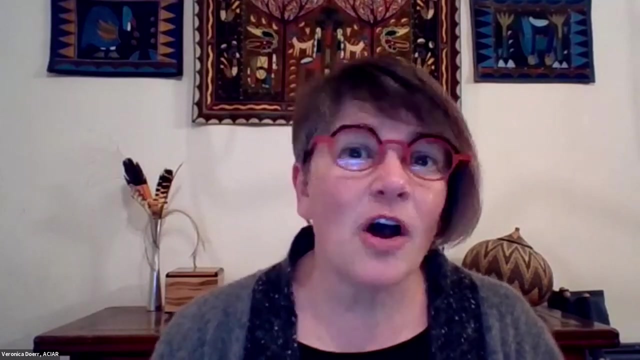 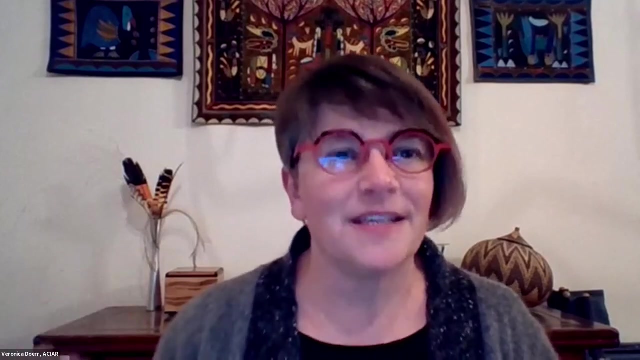 And in Australia we we say disasters are not natural. Extreme events are natural and disasters result from the choices that we make that have put ourselves and particularly naturally vulnerable people in harm's way, And what I I've heard today really reminds me that what's so innovative about everything we've been hearing is is actually about the partnerships. 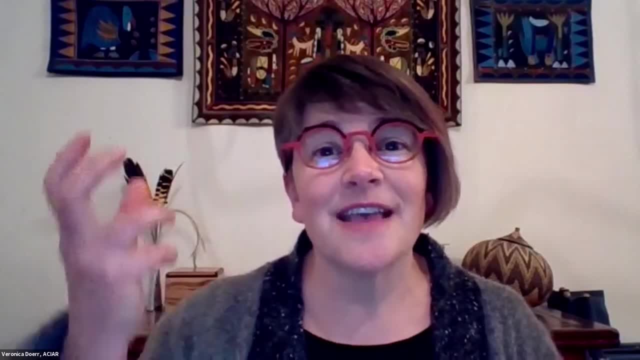 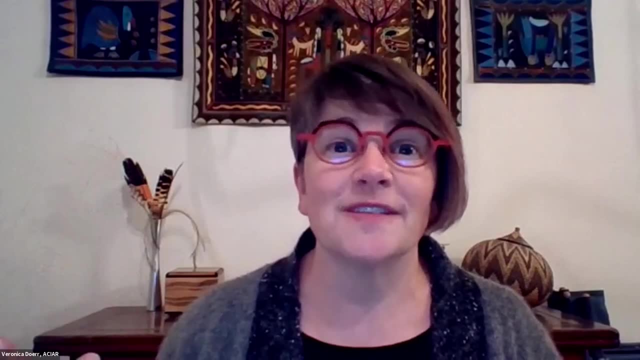 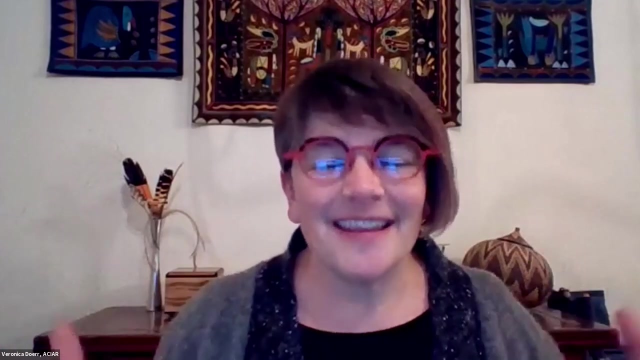 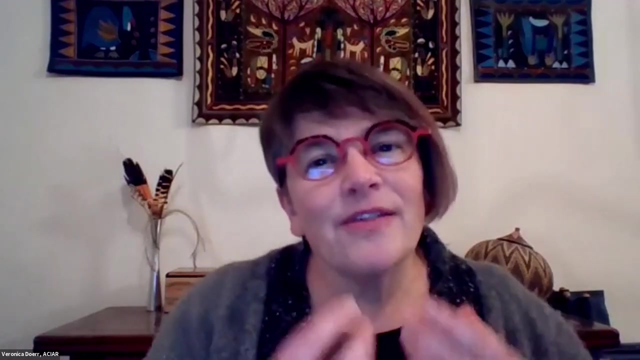 The partnerships between technical scientists and the people who have the ability to change and shift those decisions. And so so you could- you could- be amazed by the knowledge products coming out of W L, E, And, and, and you know the program initiatives, But what I'm really amazed about is the way those are so carefully tailored and 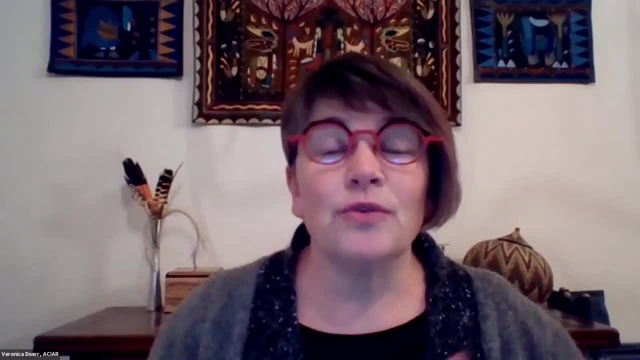 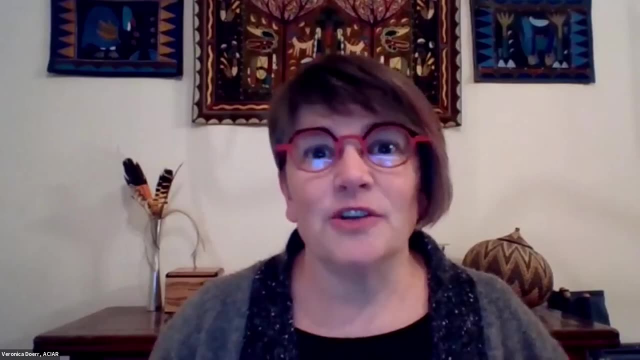 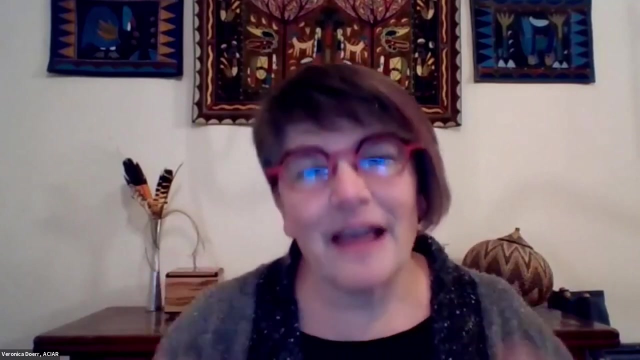 co-developed to be able to make data and information democratized and available, to be able to make insurance affordable and available, to be able to shift people's decisions. And it's those clever partnerships and the clever ways in which we use technical information. 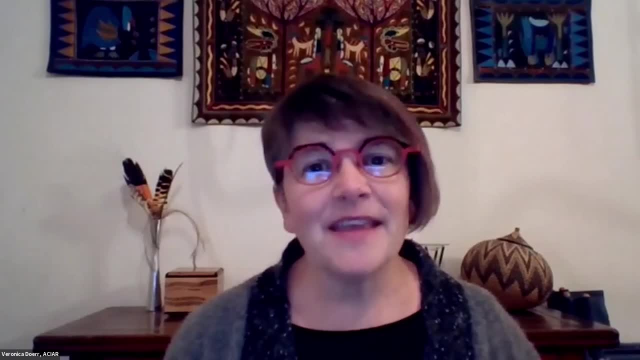 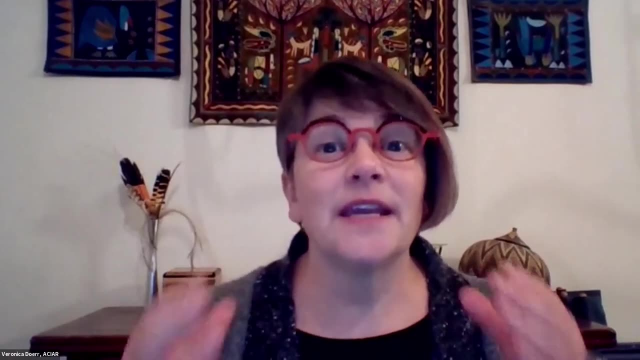 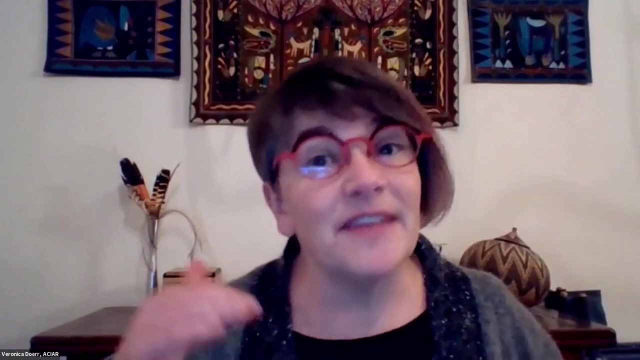 that I think are so important going forward And we need to scale those out in many places. but we also need to keep innovating. We need programs like this that keep building the next new idea and the next new partnership, because climate change gives us a 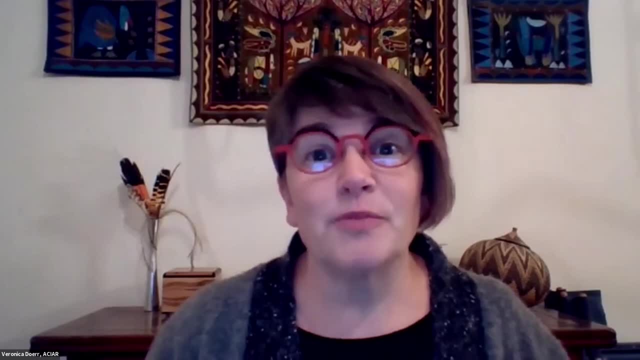 shifting baseline. We know from the climate projections that extreme events are, in some places, going to be the most important And we need to keep innovating And we need to keep building the next new idea and the next new partnership, because climate change gives us a 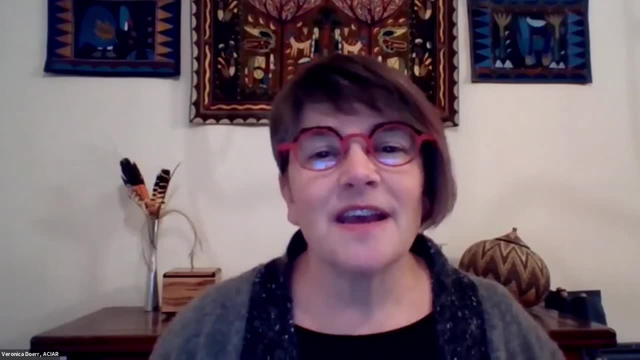 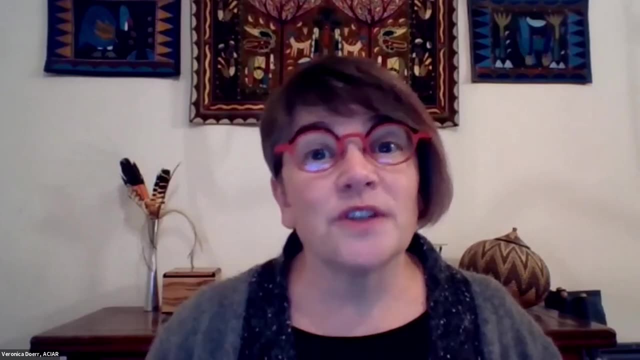 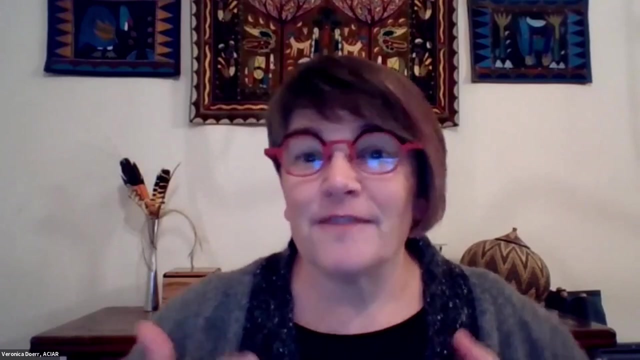 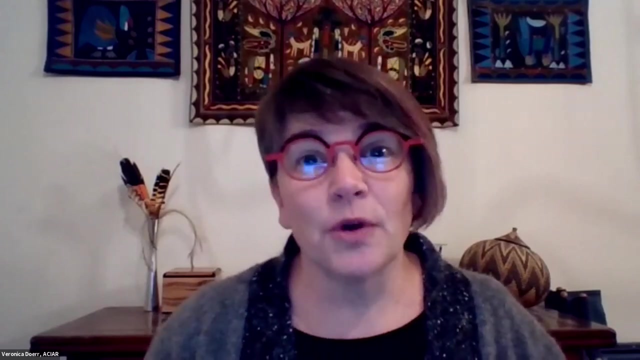 more intense, sometimes more frequent, And in Australia we're already experiencing the situation where parts of Australia we're starting to worry are going to become uninsurable. So the novel aspects of delivering index-based flood insurance will apply in some places, will be useful to us for a while, but we really need to keep thinking beyond the horizon. 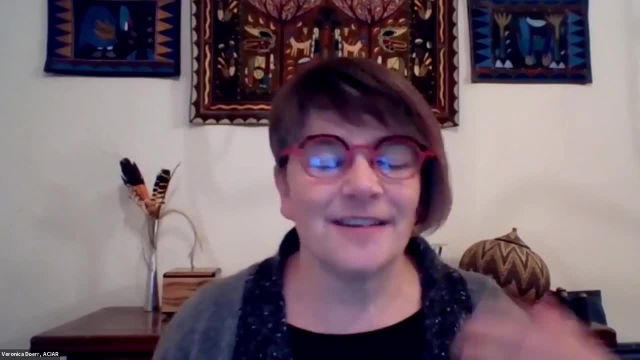 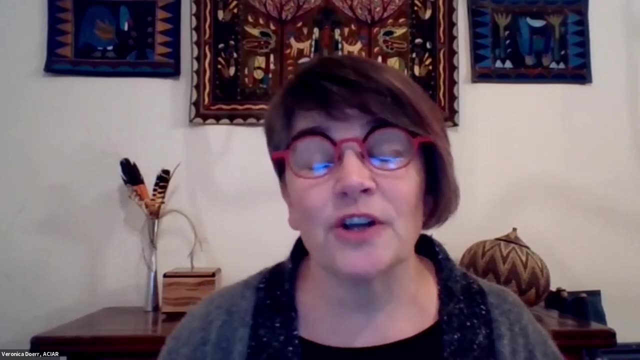 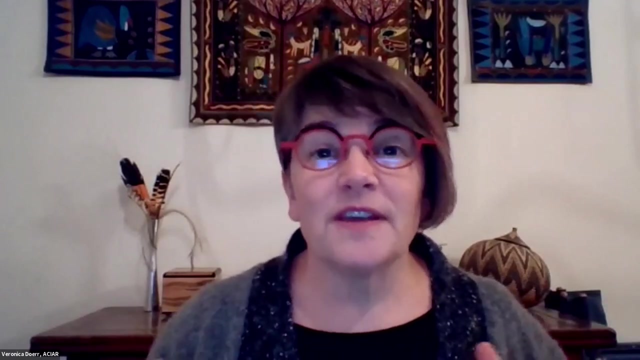 And it's that kind of combined need of scaling and further innovation that the Australian Centre for International Agricultural Research really believes the CG can deliver for us. So, as many of you will know, the CG is going through a process of wrapping up the programs, like the one we've been hearing. 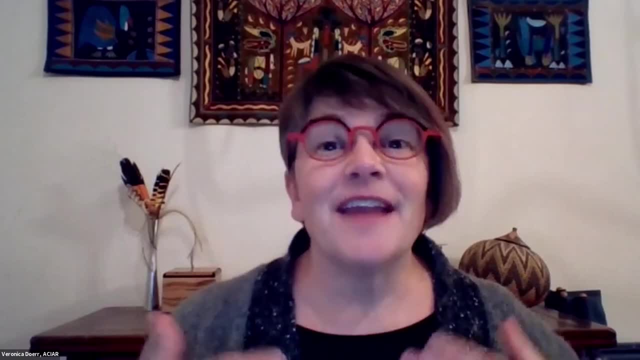 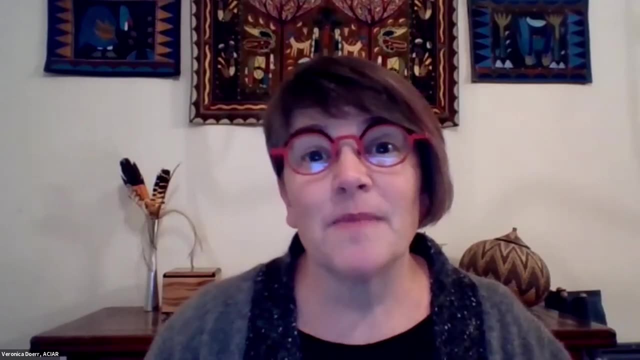 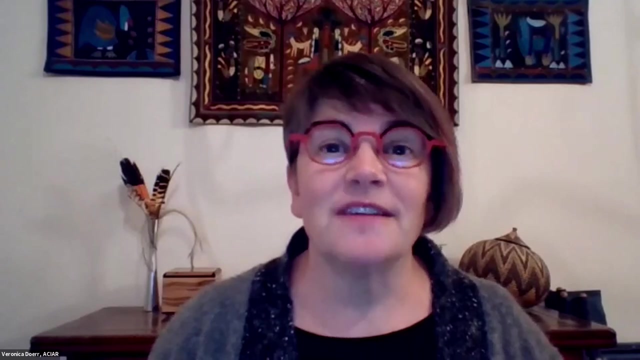 about today, but it's not the end. The next stage, commencing in January, is a set of new initiatives Where the type of work you've been hearing about today gets to be embedded even more deeply in a scaling agenda, in an innovation agenda to change systems, to really build resilience. So initiatives like 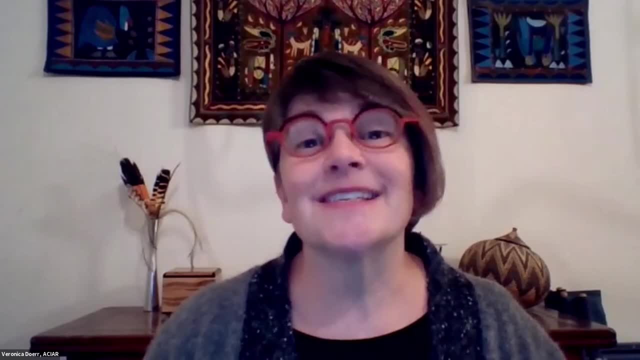 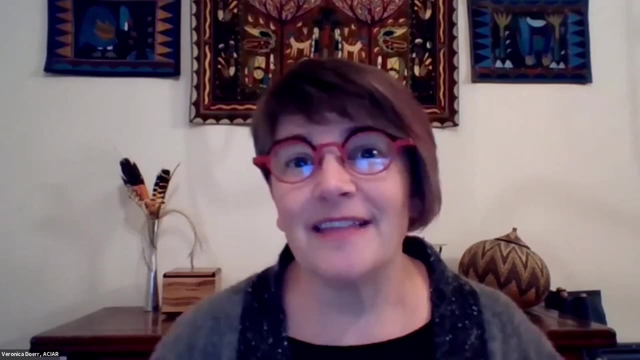 CLIMBER, an initiative that's all about building systemic resilience, are going to become the future home for the sort of work that we're talking about here, So it can keep building and these new partnerships can keep growing. So I'm really excited. 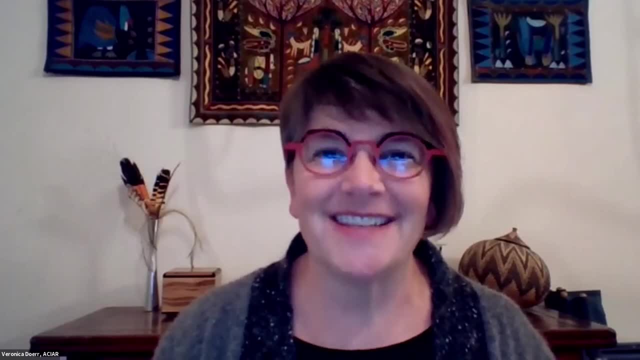 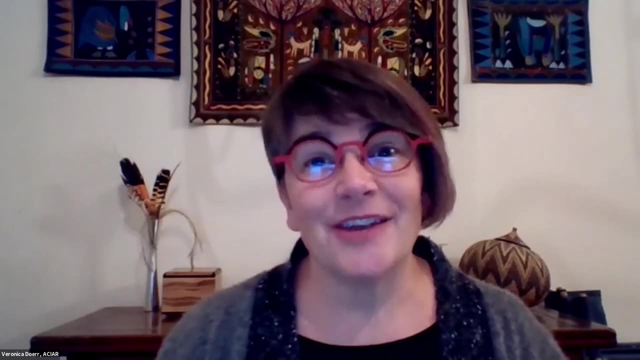 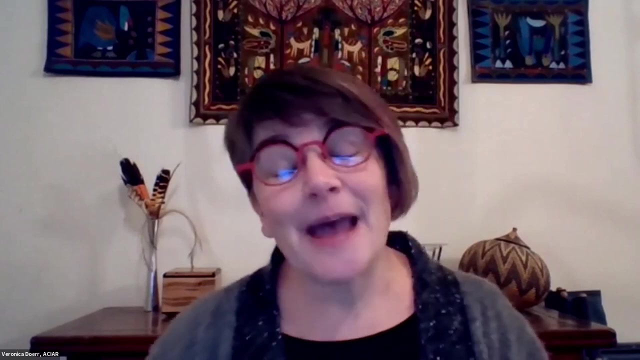 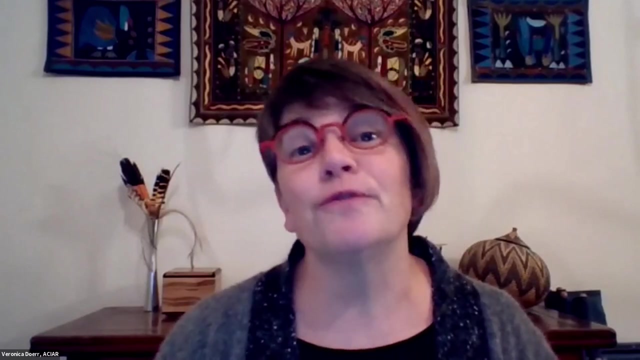 To see what the new CG is going to be delivering for us in the coming years, with the great researchers that we've been hearing from today. If you've really appreciated hearing about research that delivers on resilience, this is part of a seminar series, So the next one is happening next week, on the 12th of October, and its focus is on resilient city region food systems. 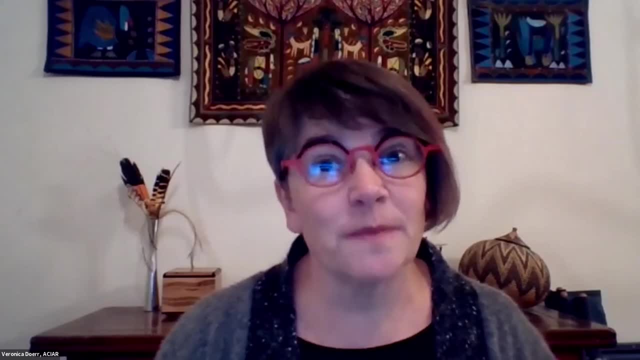 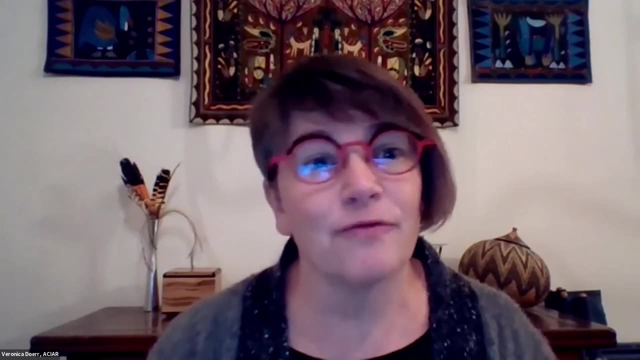 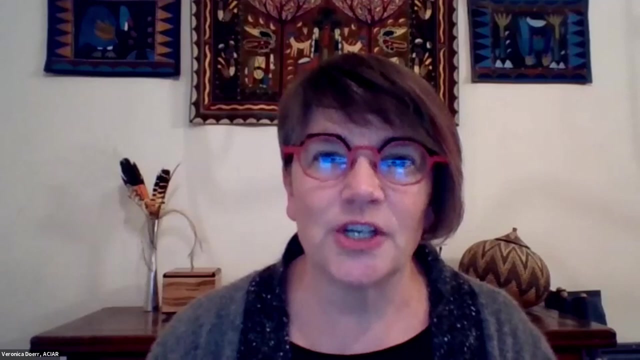 So again a very forward looking, innovative partnerships type of talk That's really digging into the critical need for us to have resilient food systems in an increasingly urbanized world and that may need to look very different than what we traditionally kind of envision when we think about food production and food systems.